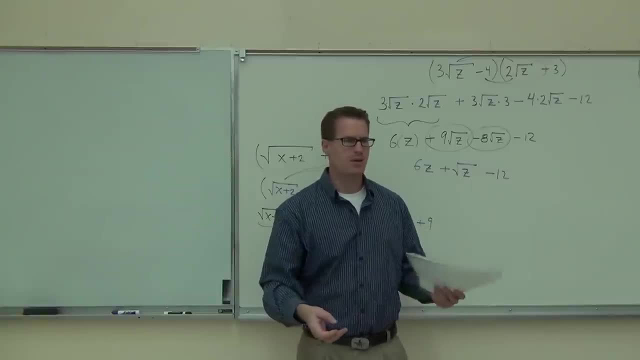 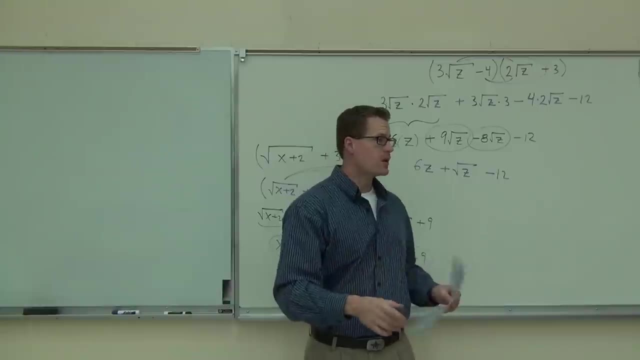 or your calculus class, You know. wait a second. how do I get rid of this? How do I move a radical around from the top to the bottom, bottom to the top? What that is called is called rationalization. We're going to learn right now, in section 10.5, how to rationalize. 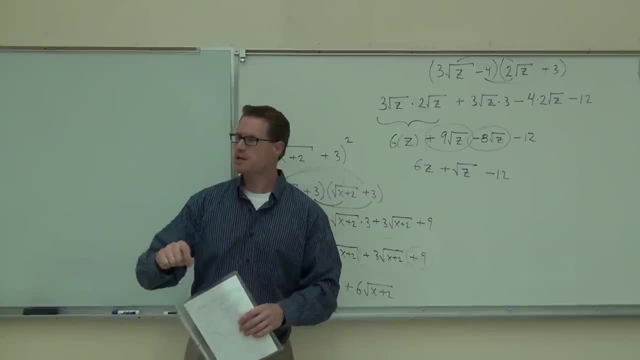 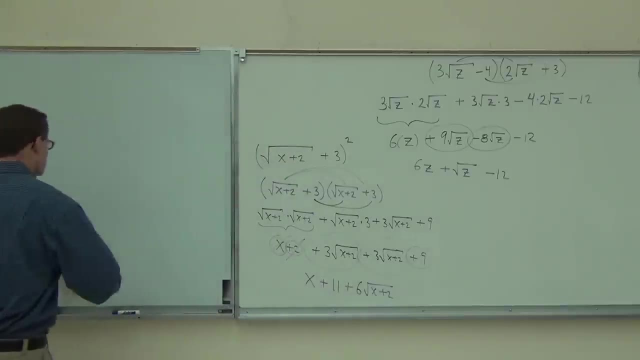 either the numerator or the denominator. Most of the time, 90% of the time, it's the denominator. We want to get a square root off the denominator Or the root off the denominator. Rationalization: We're going to learn how to rationalize. 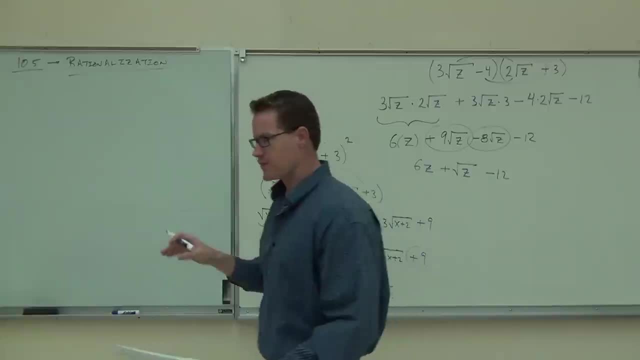 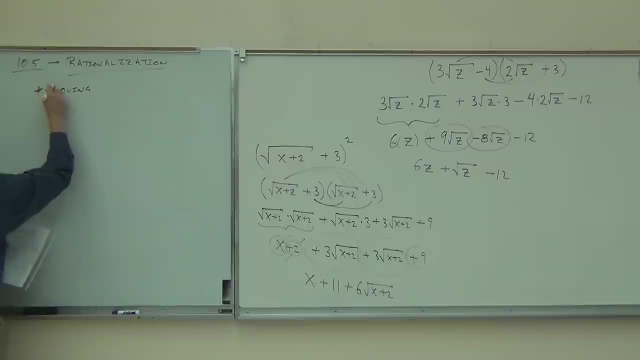 the fraction to get the radical off the numerator or denominator. So basically, we're moving a radical off the top or off the bottom of some fraction. Let's start with denominators first. We're going to learn how to rationalize denominators. 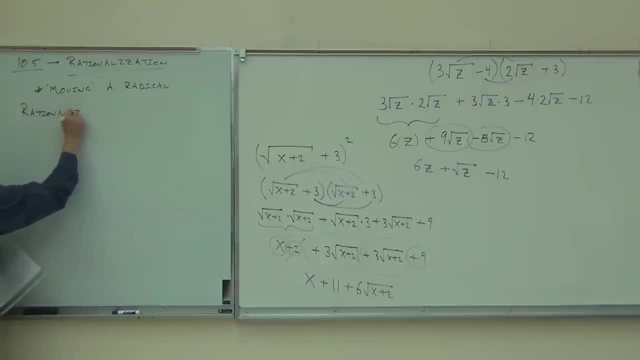 Now, there's a couple things I need you to know, and this is why I kind of went over. 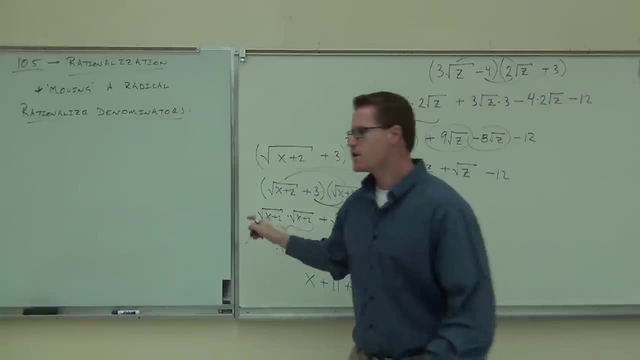 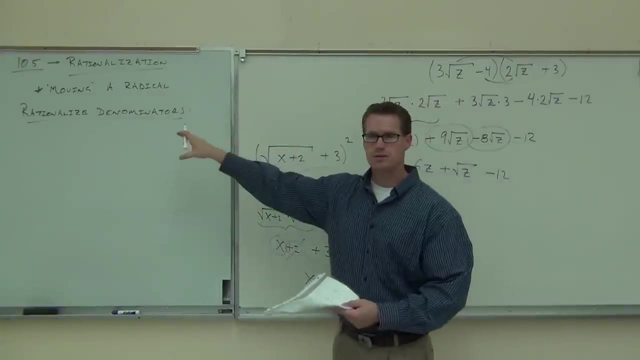 this so hard with you to make sure you knew how to do this stuff. You are going to be doing this stuff within these problems. If you don't know how to do this, you're not going to know how to do this. It's important that you get this stuff really down, which is why we went over it for another. 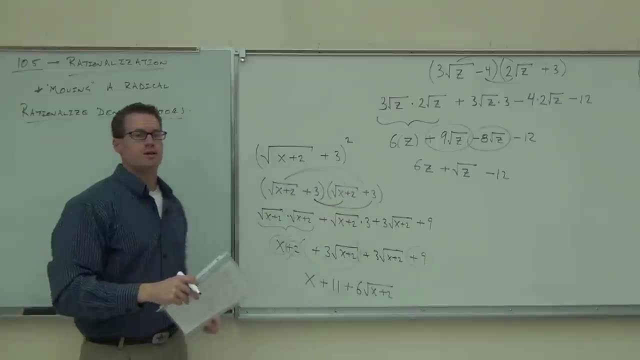 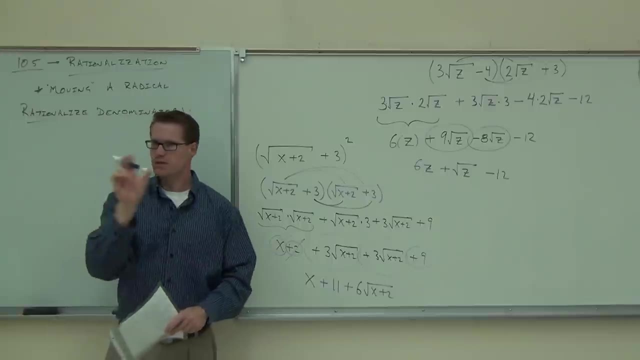 25 minutes right now on three examples, four examples: Make sure you really know how to do this. You see, the thing about what made this work so nicely is that you knew what to multiply right. You know you can multiply a root times, a self, and get the radicand. 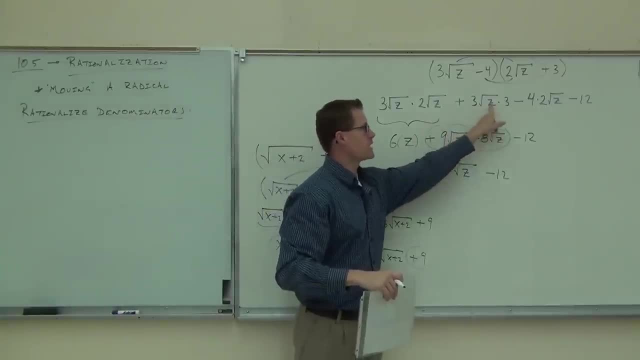 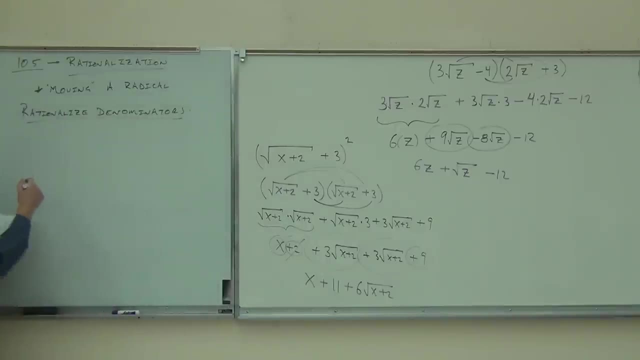 You knew you couldn't multiply three inside of that root, Namely, there's two properties we're going to be using here. The first one is, whenever you get a square root times a self, notice how X could stand for anything, Any expression, no matter what. 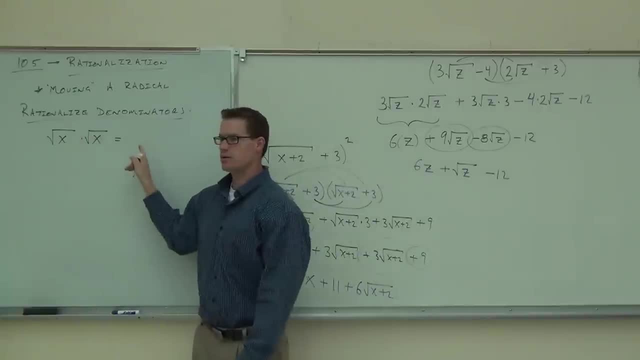 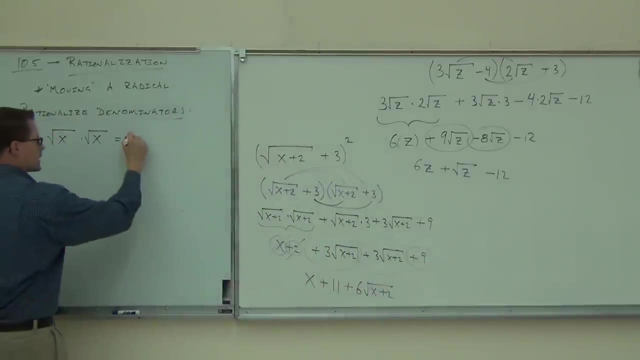 We've dealt with this several times. How much is this going to be? No square root, No square root, No, no, no. It takes care of itself, right. A square root times a self gives you the radicand every single time. 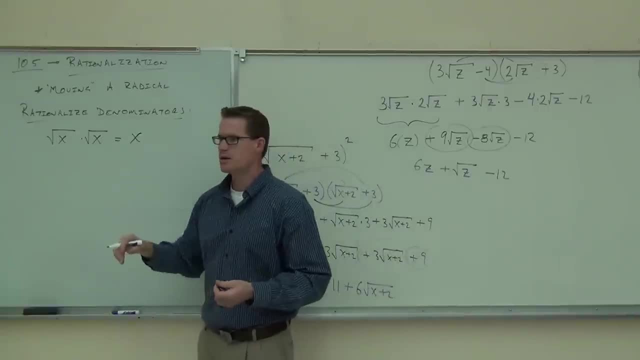 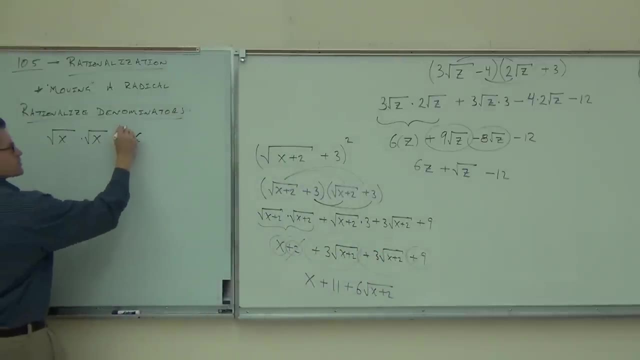 No root, No work. You didn't even show me work. I mean, this is because I'm going to show you this one time. You don't have to show this, but this is why this works. It's because you have a square root times a self that would be the square root of X. 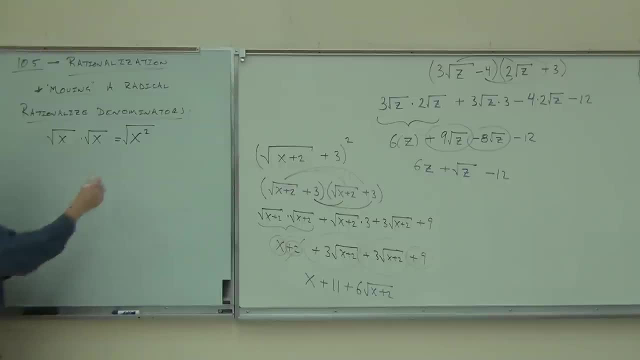 squared You with me, Yes or no? Yes, You know a square root and a square simplify and you get just an X. That's what we're getting. that a square root times a self gives you just the radicand. 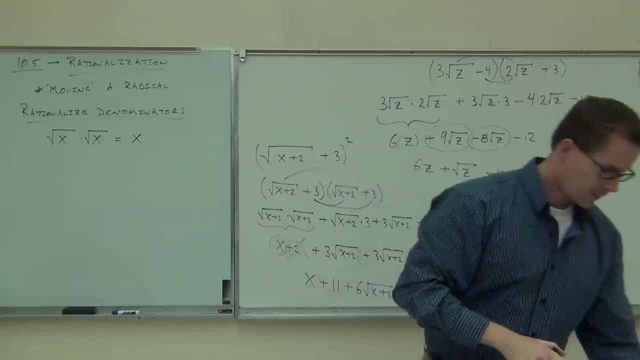 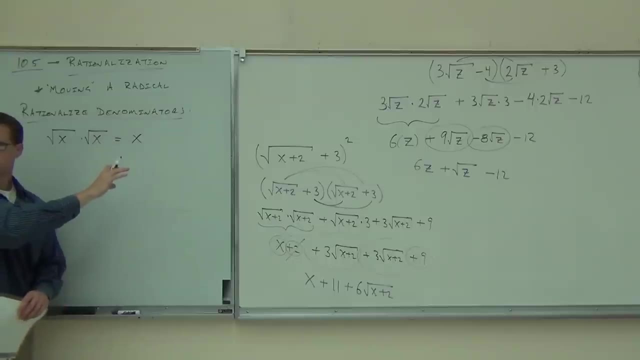 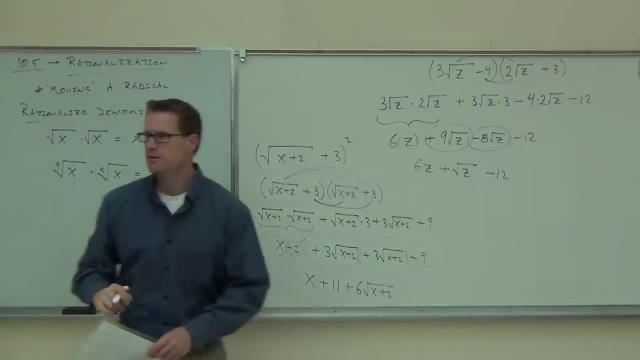 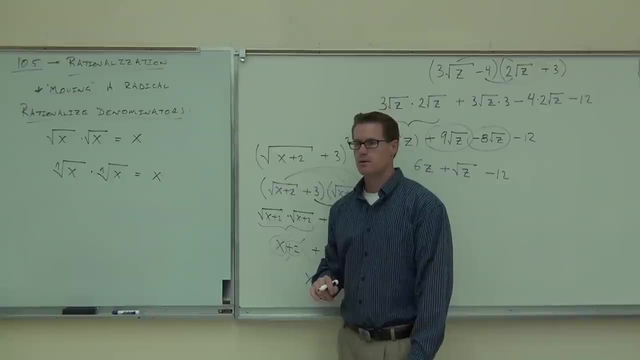 Yes, Yes, Yes, Yes, Please. I hope so. I hope so. Is that true? you think No? Well, you can't say yes or no because I haven't told you what M is. So only if M is 2.. 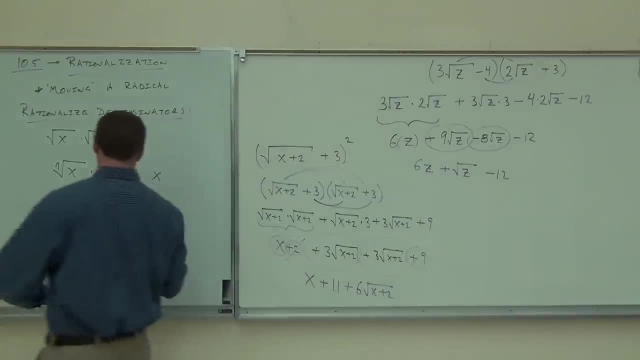 Only if M is 2.. Only if M is 2.. Only if M. why Why not? Why? Why doesn't it work? I want you to really watch this, because a lot of people get screwed up on rationalizations. 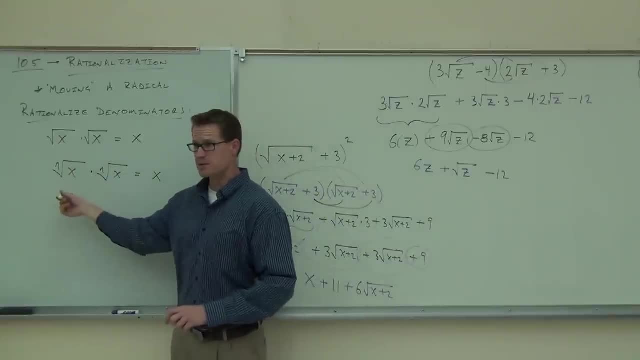 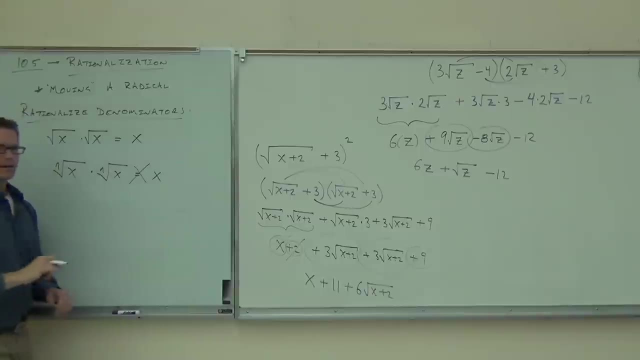 because they think that this is applied for this. okay, I'll prove to you right now, with just one example, that this is not true and not true. true, unless n is 2.. Here's why: If you have a cube root of x times a cube root of x and 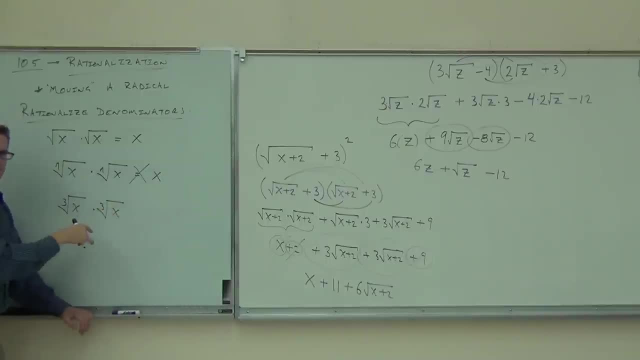 this will work for any other type of root. watch what would happen. Sure, you're going to have a cube root times a cube root, which means you can multiply those things together. right, A cube root. but what's x times x? Is it x squared or is it x cubed? What do 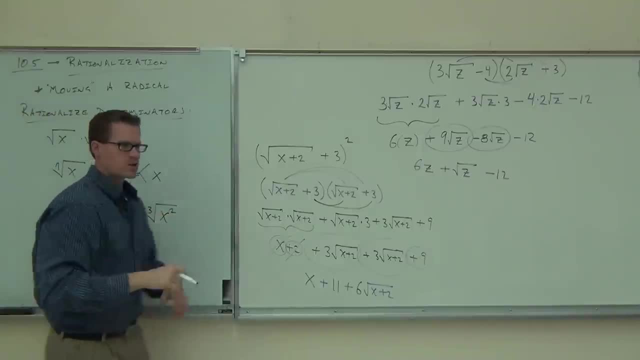 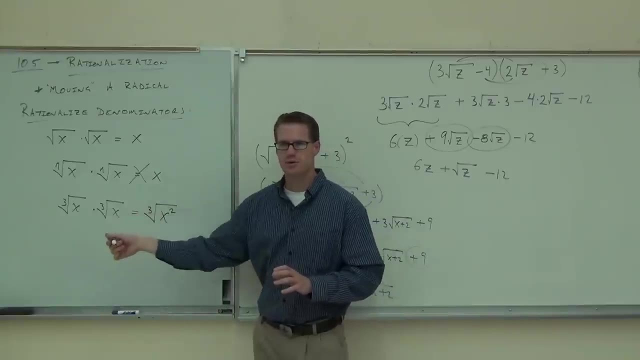 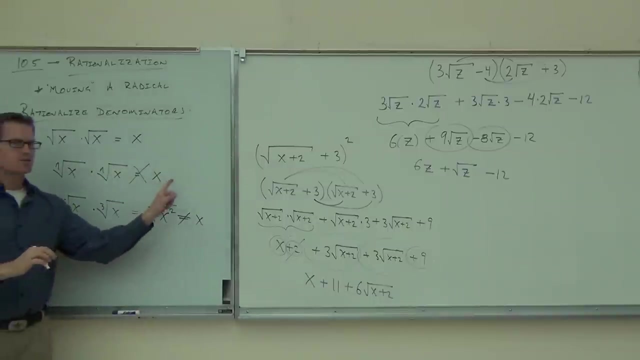 you get. Does the 2 match up with the 3?? Does the 2 match up with the 3? Exactly? Can I simplify that? The power is actually less than the root. So wait a second. this goes well. this isn't, that's not equal to x. That means that this times, this doesn't give you. 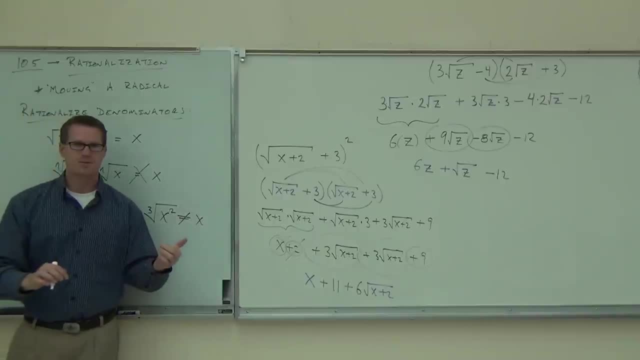 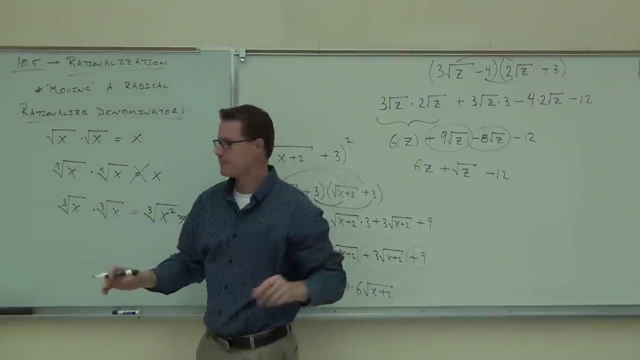 the radicand anymore. That doesn't work out. Are you following me? Okay, now I'm going to show you something kind of cool. So you agree that this works? if you have a square root, no problem whatsoever. Square roots, no problem. 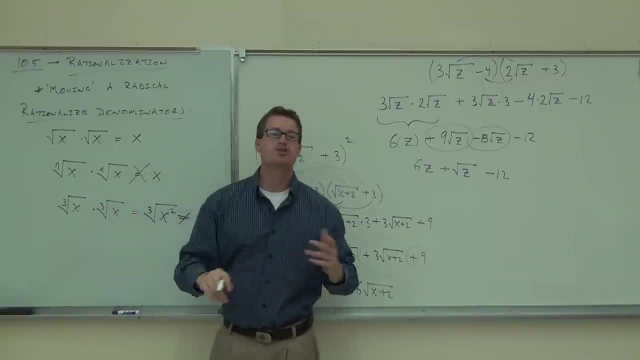 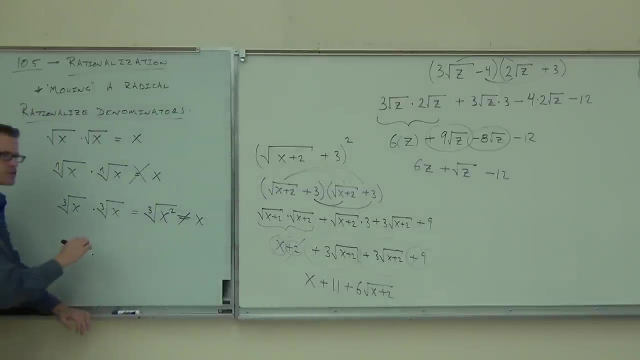 Cube roots, fourth roots, fifth roots. we have a problem here. My question is this: I don't want you to answer out loud. I want you all to think about this. The question I'm going to ask you is: is there something else? again, don't answer out loud, I want 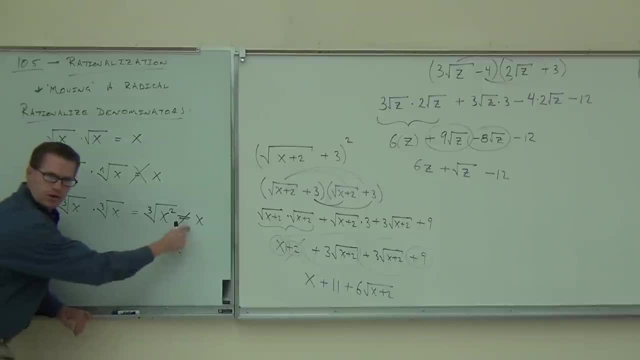 you to think: Is there something else? you know that this didn't work. is there something else you could multiply here that would limit the root? That's the question I'm going to ask you here in just a bit. So I knew that this didn't work, but let's pretend I still. 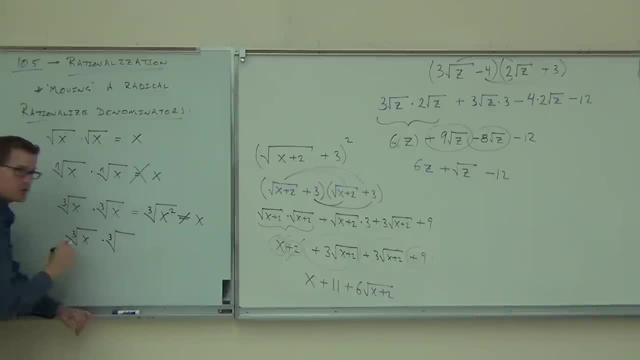 had that. okay, And I know that this didn't work. but you can think about what. I need to multiply by something And I need to multiply by something. I'll give you that it's going to be a cube root. that's the only way you can put those roots together. is there something I could? 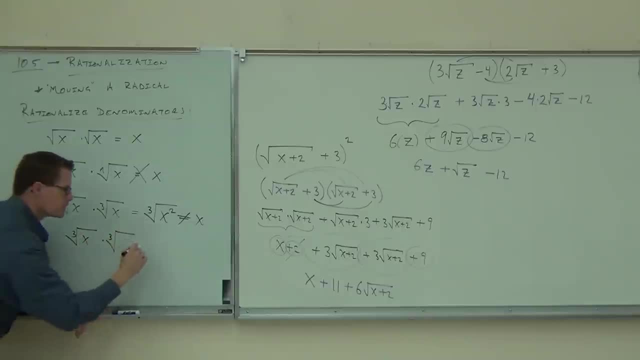 multiply by in order that I can get something that will simplify. What do you think? x square? Well, not x. right? X would give you x square. What I'm looking for, follow me along if you're not really getting this yet. What I want to happen, I want the power to match the root. 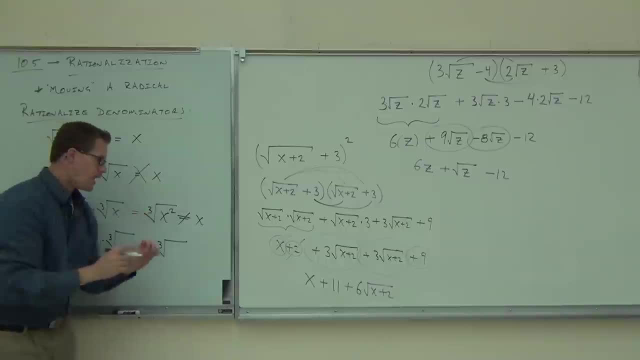 The power match, the root of the square, root of x squared. I want this. Can you explain to me why I want that? Sure, that's what I want. right, I want to get rid of the root. That's what I want. 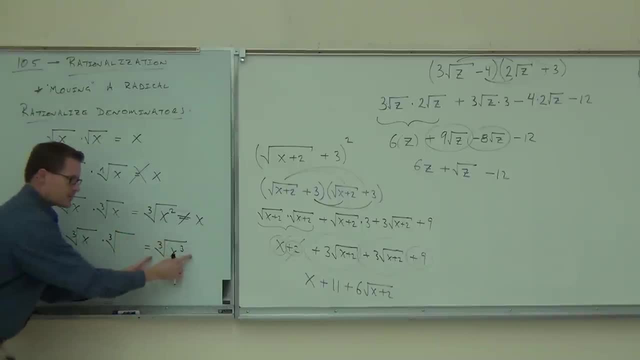 The question is: if I have this and I need this, what does this have to be? Sure, Yeah, Why? Because you know x times x squared gives you x cubed right. So for square roots it's easy. 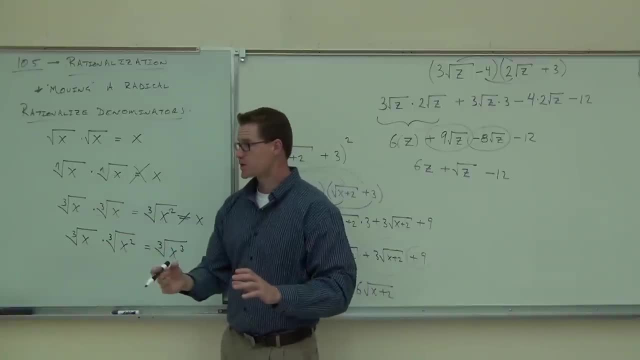 Square roots are nice. You multiply it by itself and that eliminates the radical, Because you know a square root times itself gives you the radicand. I don't know if you're with me, If you have any other type of root. you've got to multiply it by whatever you need to make the power match the root. 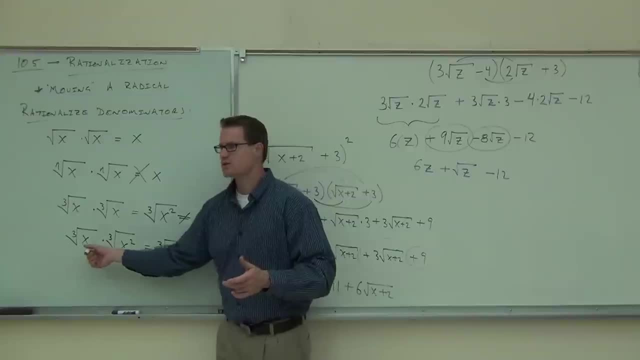 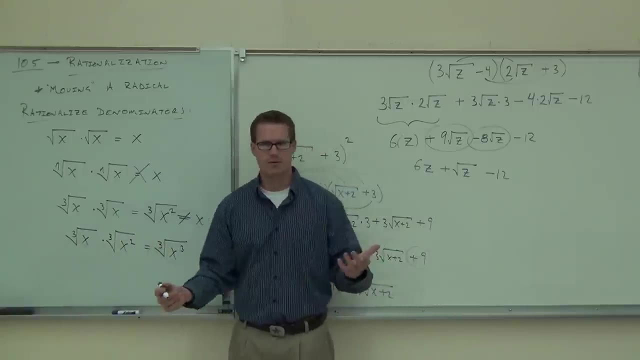 So in our case, right here, it's not just the same thing that's not going to work. It's whatever you need to multiply by to match up to a perfect cube or a perfect fourth or whatever n through you have. Do you see the difference? 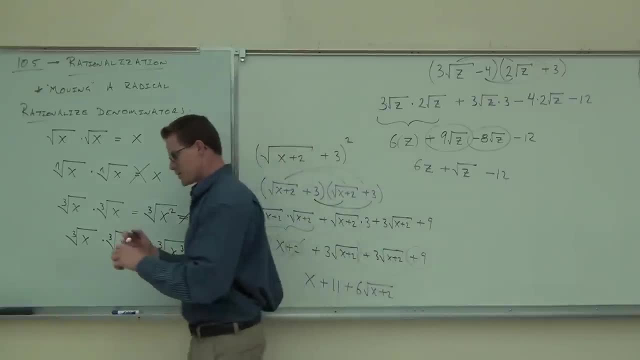 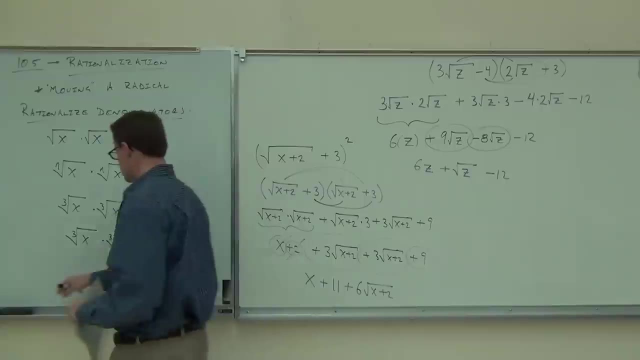 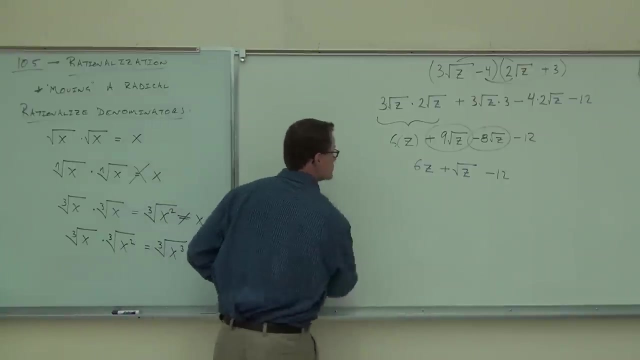 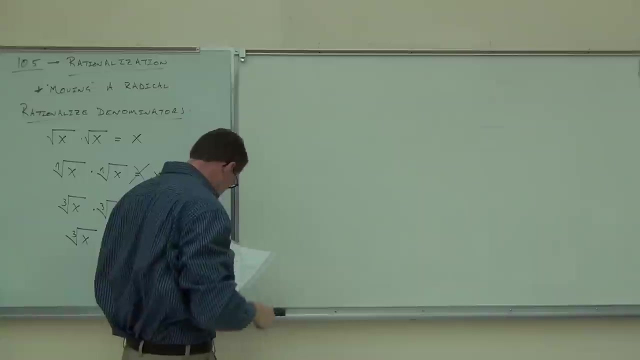 In that case, this would be great. That would be great. That would work for you. Now let's put this into practice. see how we're actually going to rationalize some denominators here. then move on. We're going to start off nice and simple. 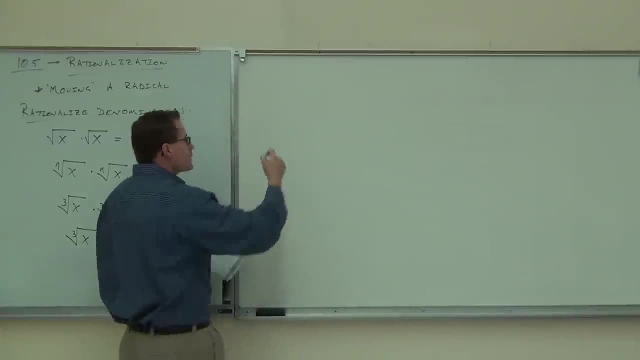 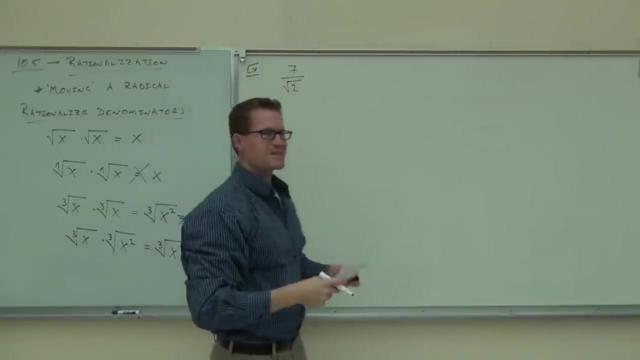 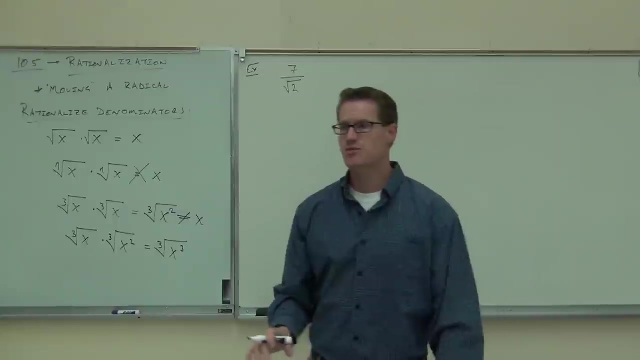 I just took some numbers. We'll gradually move on to some things that have some variables. Okay, rationalize the denominator means I want you to get the square root, or whatever root you have, off the bottom of the fraction. Rationalization means move the radical from where it is, out of where it is. 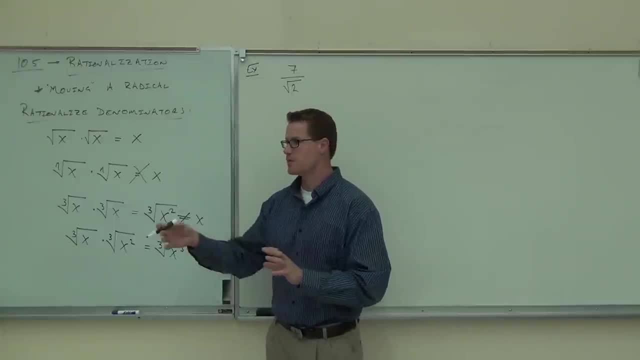 Okay. so if it's on the denominator, if I say rationalize the denominator, it means get the radical off the bottom. If I say rationalize the numerator, it would mean get the radical off the top. Are you with me on that? 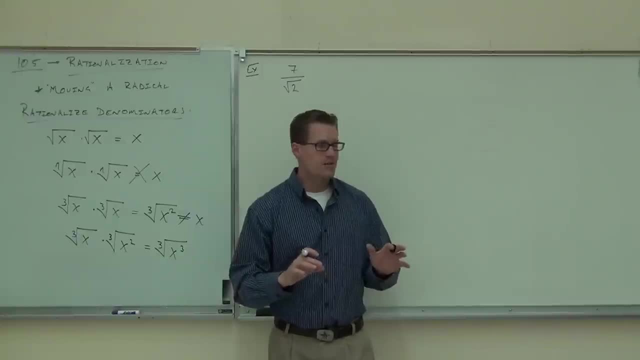 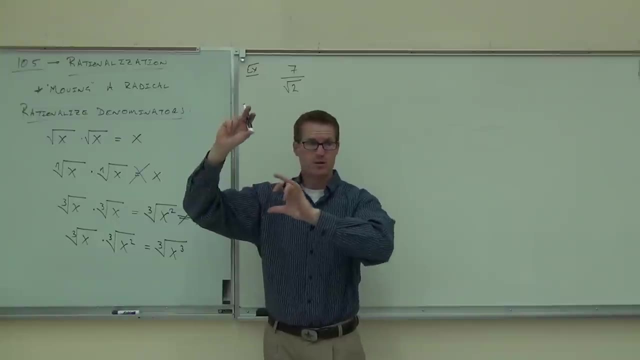 So you're going to be doing both. So you really need to read these problems correctly. If I say rationalize the numerator- and there's two roots, it means get rid of the radical on the top. If I say rationalize the denominator, it means get rid of the radical on the bottom. 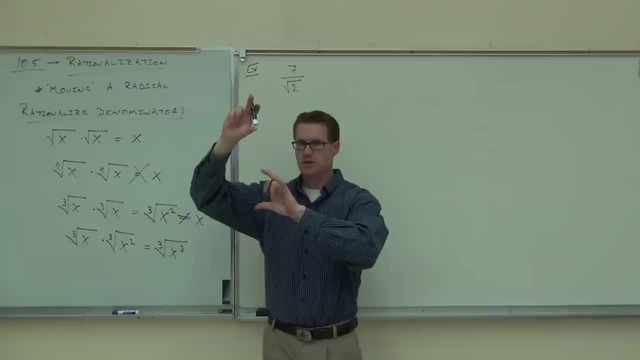 You're going to have problems where you have roots on both the top and the bottom. Okay, You need to read your problem and know what you're talking about. So 7 over the square root of 2, there's only one root. 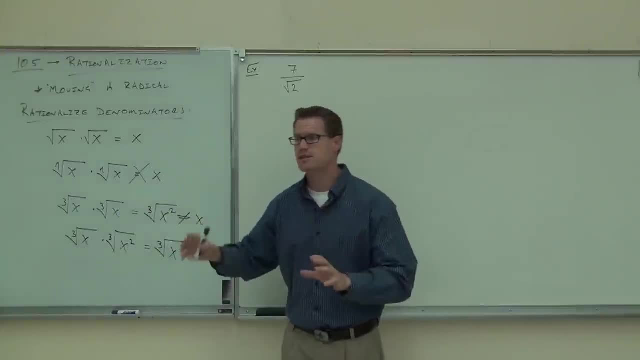 Chances are we're probably rationalizing that one, But this will all be rationalized in the denominator for this little section here. When I go to numerators, I'll tell you specifically what we're rationalizing in numerators after that. Now 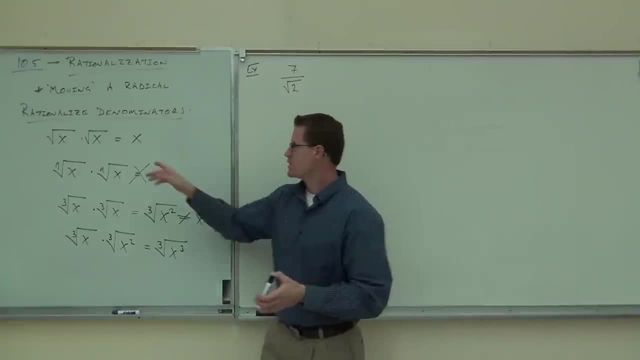 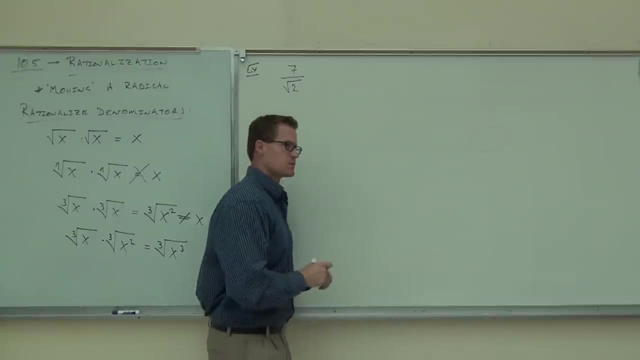 In order to rationalize the denominator, we knew that we needed to multiply by something. What type of root do we have here? Root 2.. What type of root? Square root, Square root. Okay, So we're going to be multiplying by something. 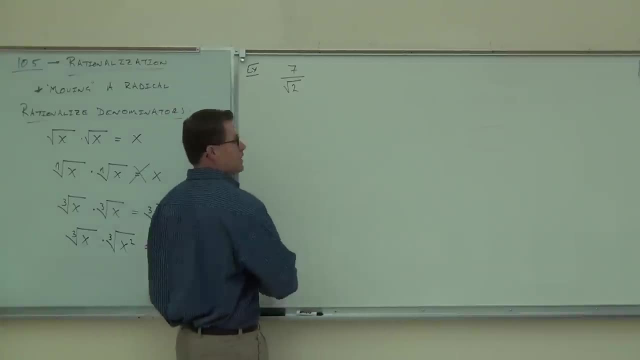 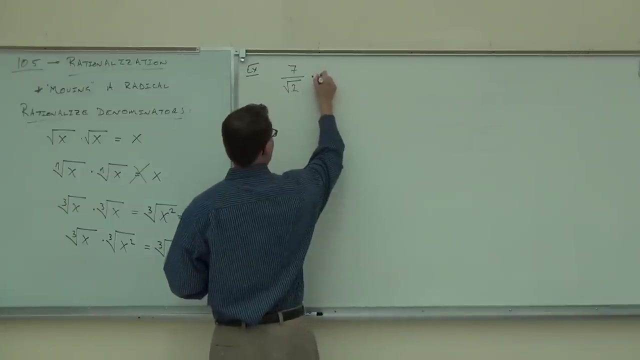 You agree? Yes, Okay, So somewhere we're going to be multiplying. That's the only way you can get rid of a root. You can't add anything to get rid of a root, You can only multiply. Now, when you multiply, 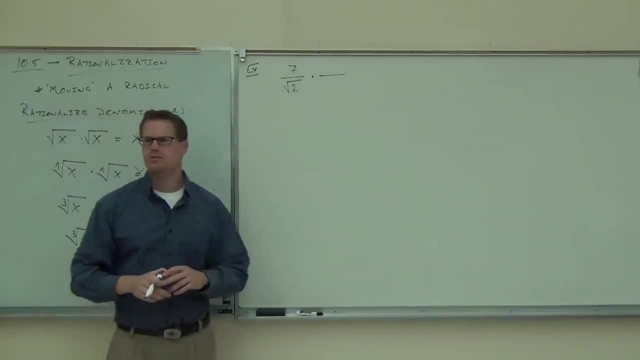 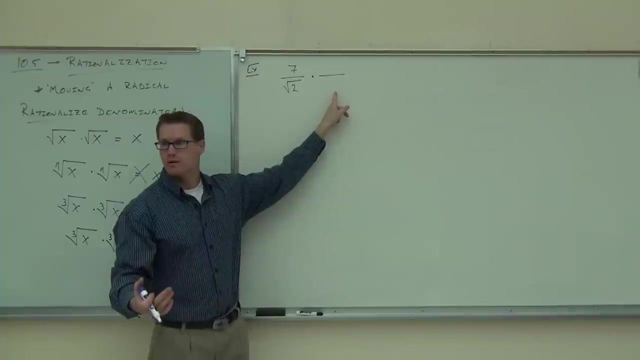 What I know. Actually, what do I know? What do you need to multiply by in order to get rid of the square root of 2?? So 2 won't work right, 3 won't, 6 won't work. 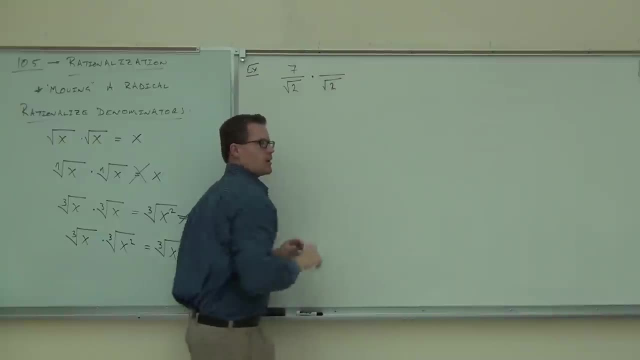 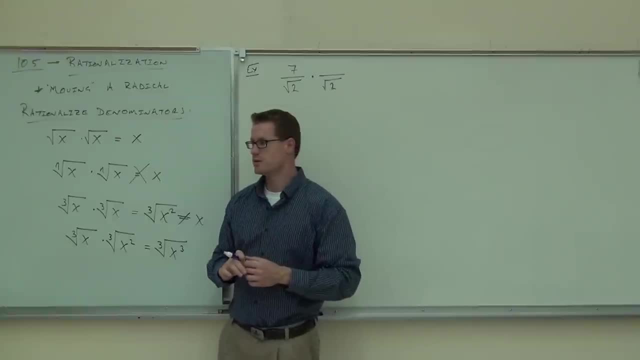 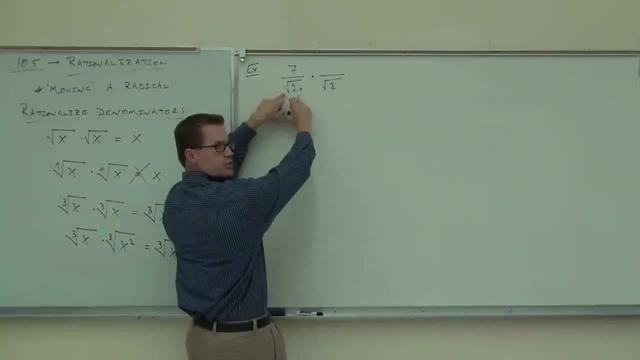 So here I know that this right here is going to deal with my problem. True, It's going to get rid of the root on the bottom. That right there is a necessity. It means if I multiply this by something, I must multiply this by the same thing. 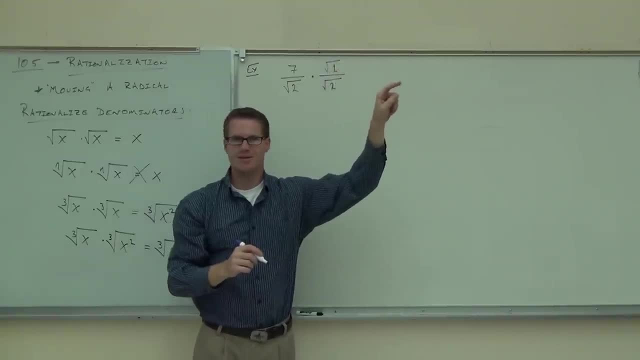 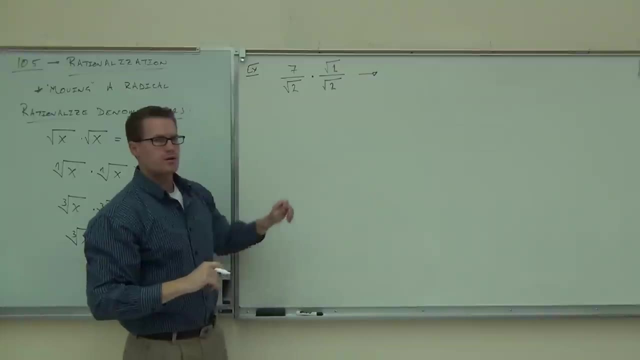 Otherwise it changes the value of my fraction. You okay so far? Yeah, Let's see what happens. Can you all tell me what we're going to get on the numerator of my fraction, 6 over 2.. Not root 14.. 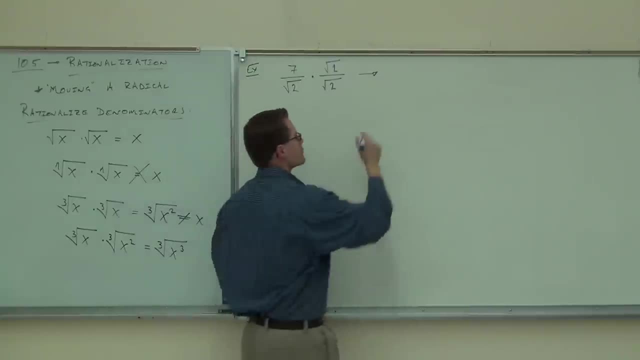 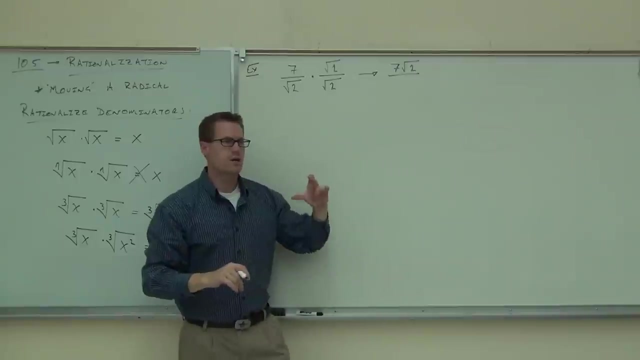 We already talked about that a lot in this class, right, That's why we did this, that other section first. So 7 root 2 over. Now let's look at that. What's the square root of 2 times the square root of 2?? 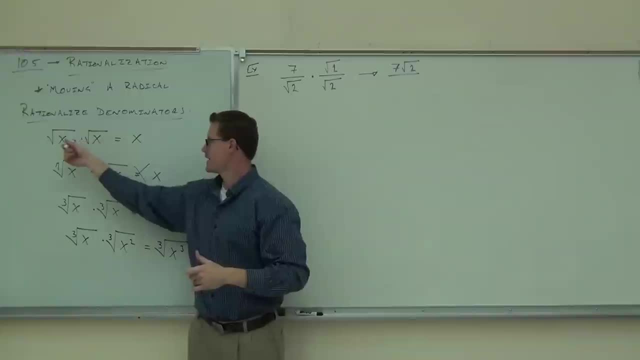 2. That's why that worked right. The x isn't just an x. The x is anything that you want it to be. A square root times itself gives you Just the radicand. Whatever you're multiplying inside of that radical, because you're going to get. 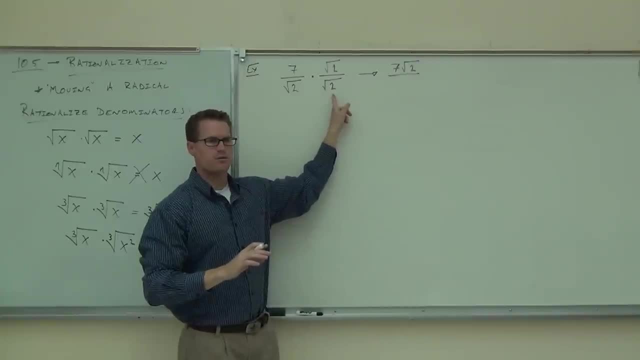 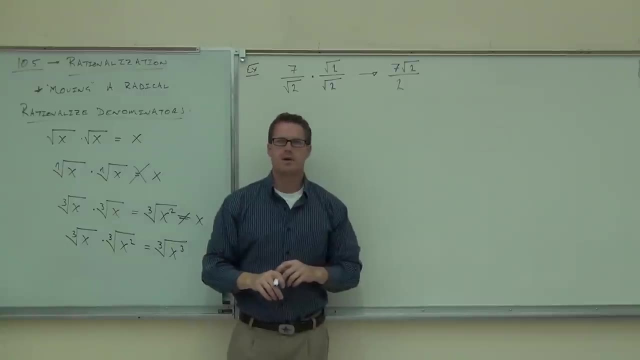 if you look at this, this is the square root of 4, right, The root of 4 is 2.. That's why it works. It works every time. You're just going to get a 2.. Now did we get rid of the square root on the bottom of the fraction? 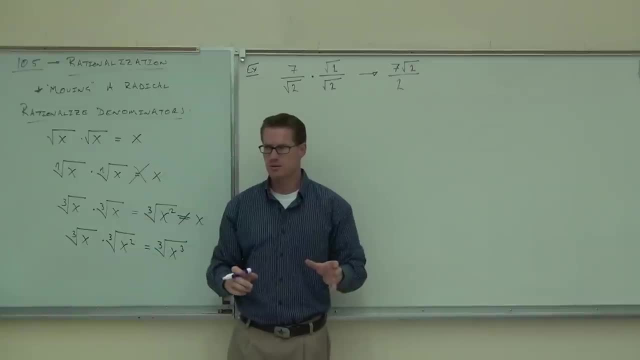 Yeah, Did we get rid of the square root altogether? No, No, it's still there. It will always still be there. You can't ever eliminate the square root- ever- unless you have an equation. Okay, remember the fraction fraction idea. 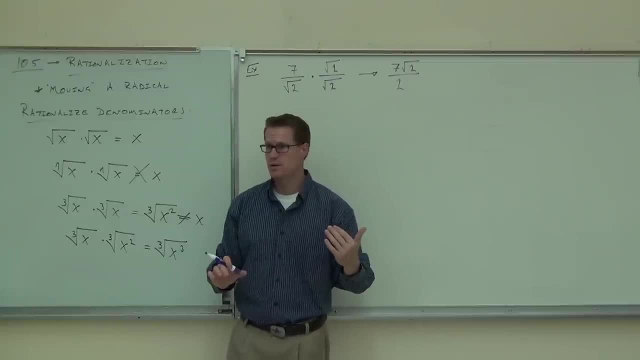 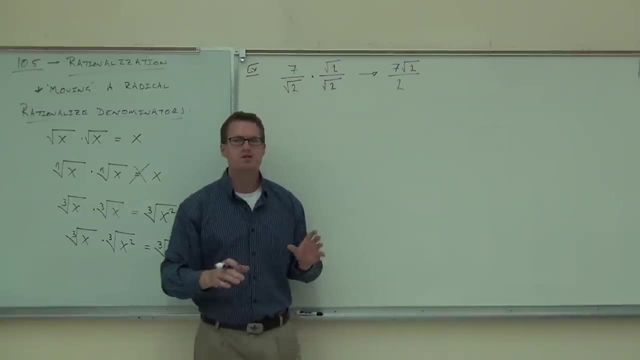 When you had an equation, you could get rid of fractions. When you didn't have an equation, you couldn't get rid of fractions. All you could do is find common denominators, things like that: Same idea here. all right, If you have an equation, I'm going to show you how to get rid of roots. 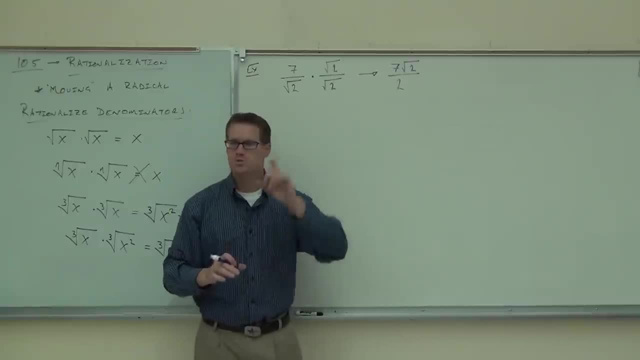 If you don't have an equation, all you can do is move a root around. All you can do bottom to the top, top to the bottom. That's it And that's the rationalization idea. Now, do you know if you're still okay with this? 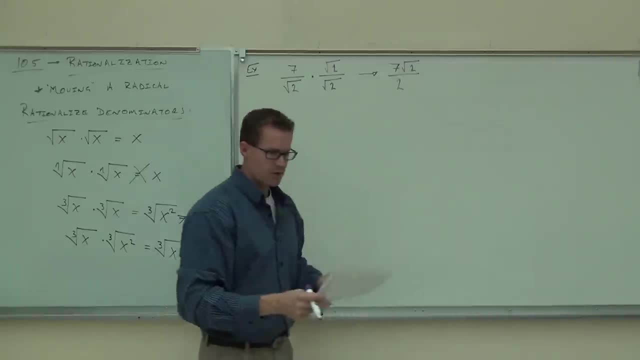 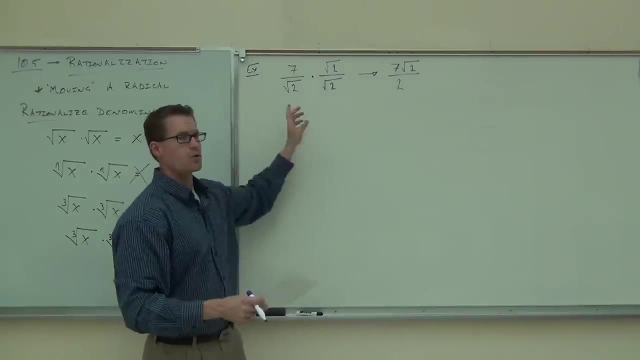 Cool. So to rationalize denominators, you're going to multiply both sides. You're going to multiply both top and the bottom of the fraction by the root, whatever root you need to rationalize, either, like a square root of 2,. 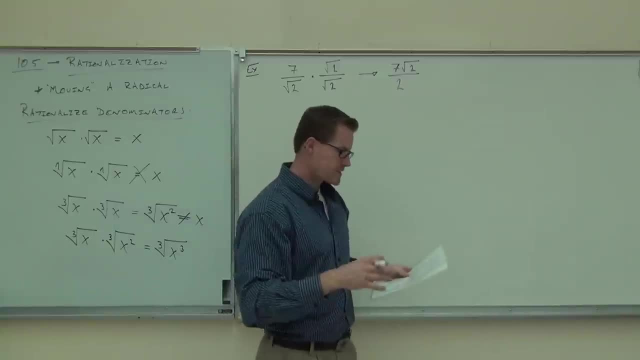 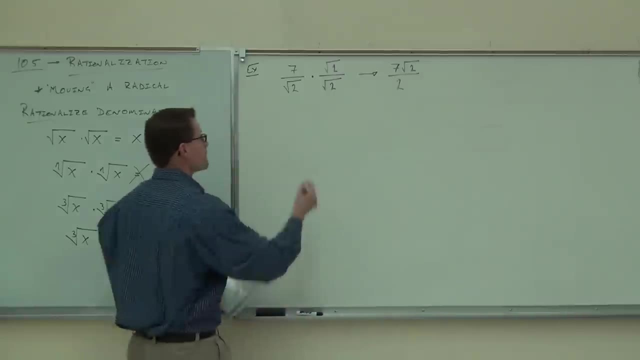 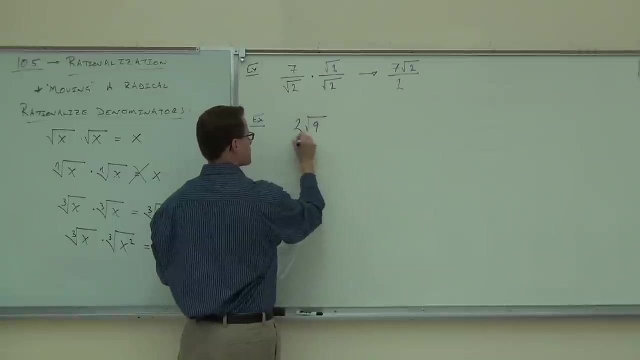 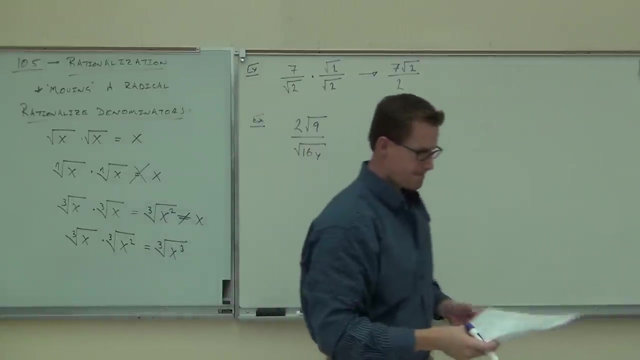 or if it's on the numerator, whatever root you have there. Essentially, we're multiplying by 1.. Let's do a few more examples and I'll show you how to do this with a couple different expressions here. Okay, 2 root 9 over the square root of 16.. 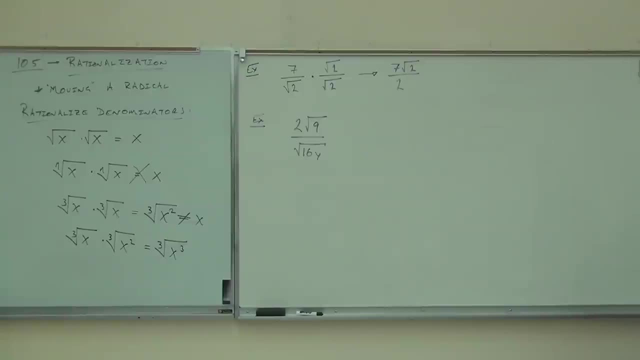 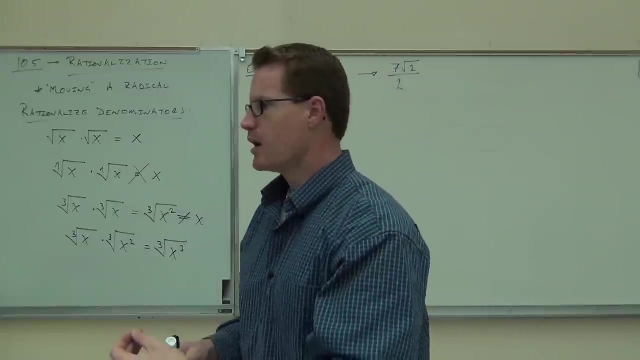 Now, before you get all crazy with these radicals, before you do that, you might want to try to simplify them, because the less you have to multiply, the less convoluted this problem is going to be. So when you look at this problem, do you see anything you can simplify first, 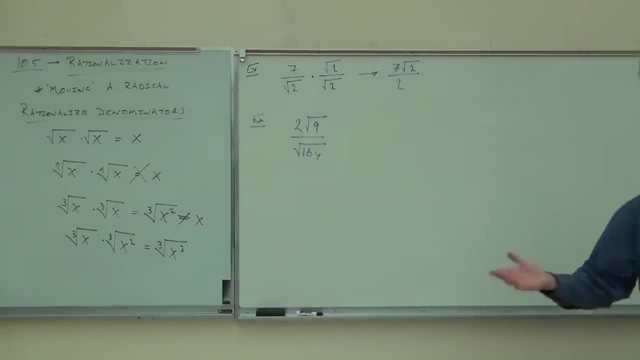 Yes, The root 9.. Yeah, let's get rid of the root 9.. I mean, my goodness, how much is root 9? 3. That's right, Let's get rid of that thing. Don't leave that root 9.. 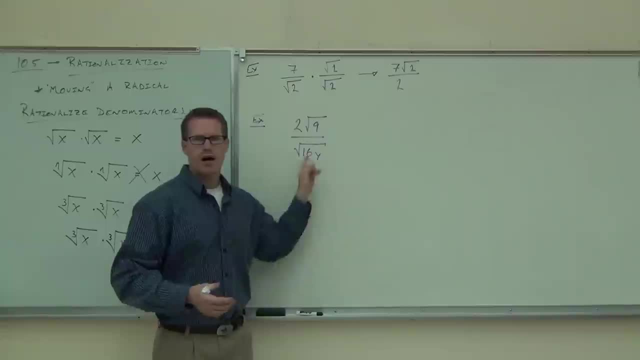 That's going to make the problem more confusing. How about the root 16y? Can you simplify that? Yeah, sure, That's what? 4y, 4y or 4 root, y, 4y. Okay, so the square root of y that power is 1.. 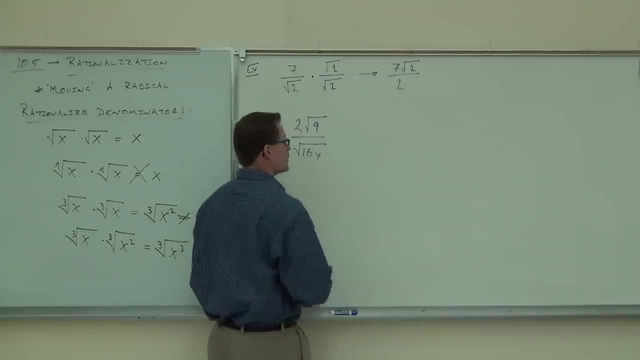 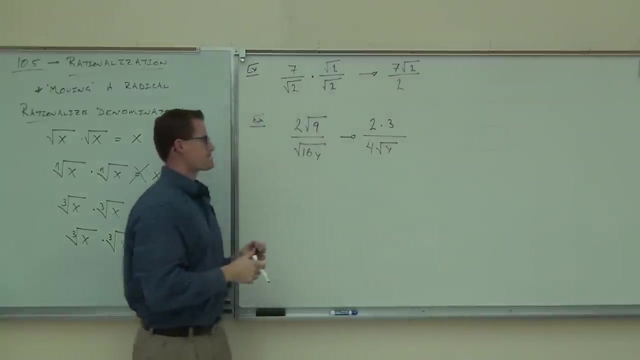 I can't simplify that, but I certainly could make this 2 times 3, that's 3, over 4 root y. You follow me on that, Mm-hmm? Okay, good, We've done a lot of simplification so far in this class. 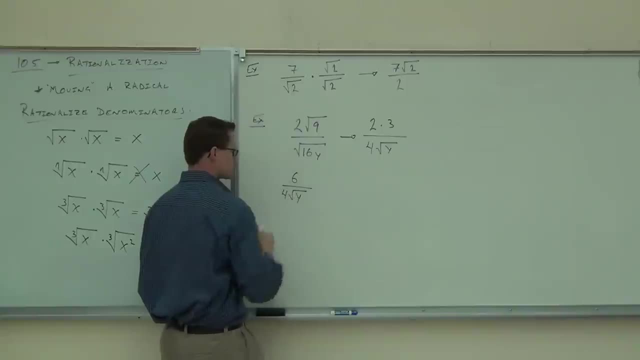 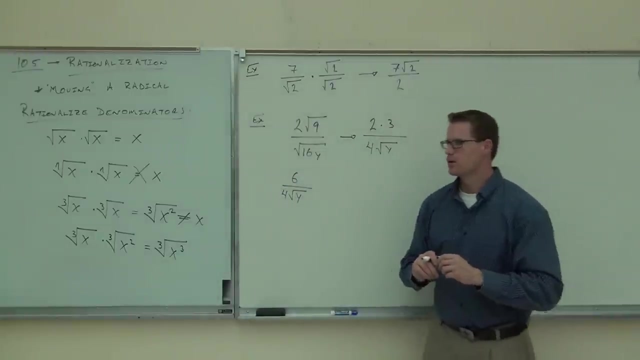 We have 6 over 4. root y Hey. anything else that you can do before you go any further, Simplify 6 over 4.. It's a fraction, right, It is. It's a fraction. In fact, you could have done that here. 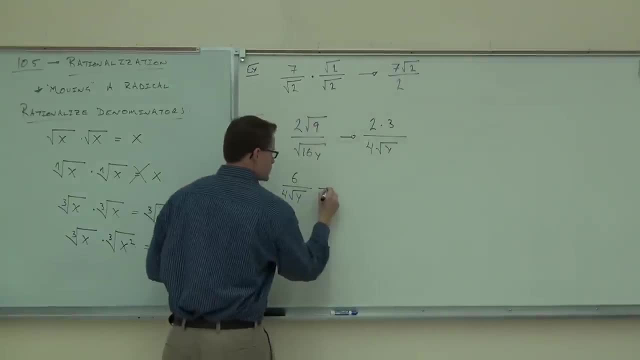 2 and the 4.. You could have done that, And it's 2 and the 4.. Let's do one more step. Instead of 6 fourths, this is multiplication. I could do 3 over 2 root y. 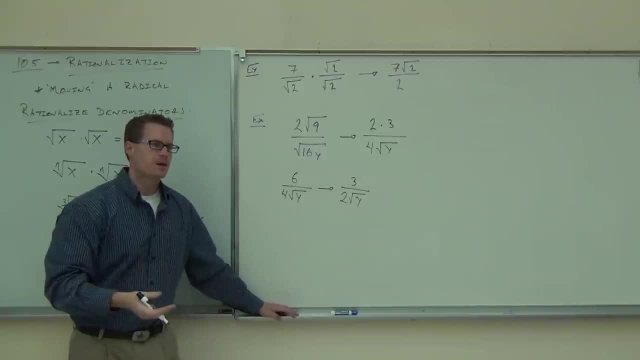 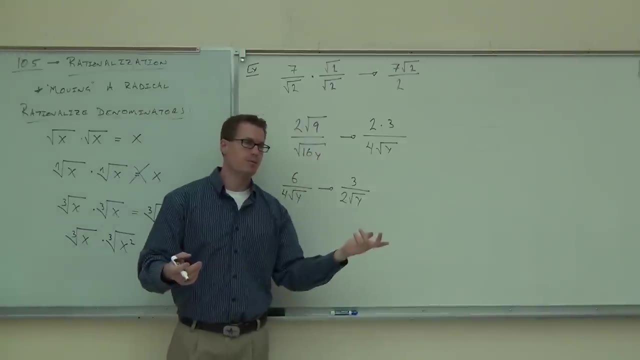 So far, so good. Mm-hmm. Okay now. Now you're supposed to rationalize the denominator. Could you have done it here? Sure, It's going to be more work and more simplification for you at the end of your problem, okay. 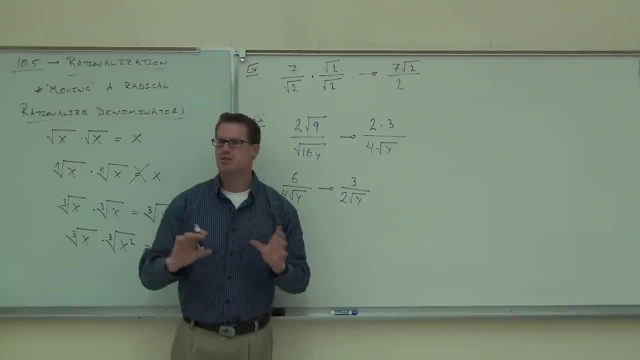 But if you don't do this, you can still get the right answer. It just requires you to simplify more. My question is: what exactly, if I'm supposed to rationalize the denominator, would you get rid of the denominator? What exactly am I supposed to get rid of here? 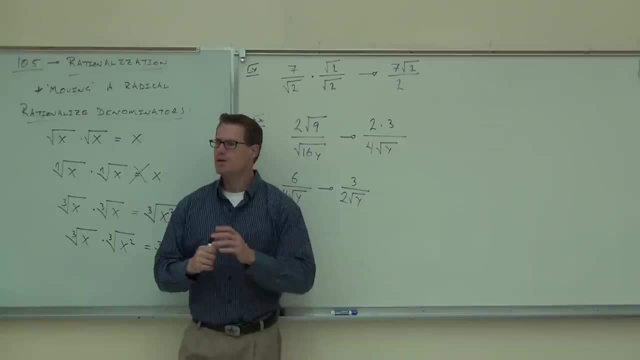 The y, The y, The y, The root, y. Am I trying to get rid of the 2?? No, I don't get rid of the 2.. The 2 is not in the square root. What I'm trying to get rid of is the square root of y, not your root. 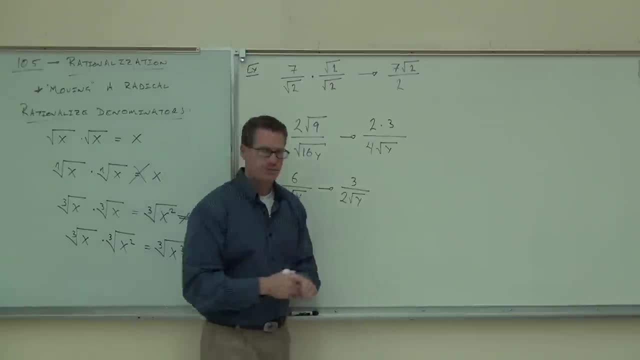 Okay, so when I multiply- which I know I'm going to have to do because multiplication is the only way that you can get rid of a square root, at least in one spot of this fraction- When I multiply, do I want to multiply by another 2 here? 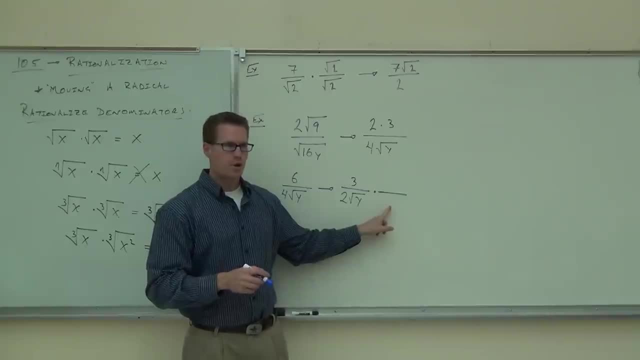 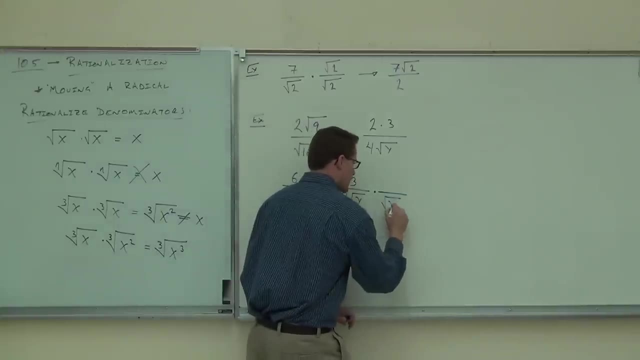 No, No, I really don't care. I don't care about the 2.. What I care about is the square root of y. What am I going to multiply by then? The root y, The root y? Sure, Why not the root y? 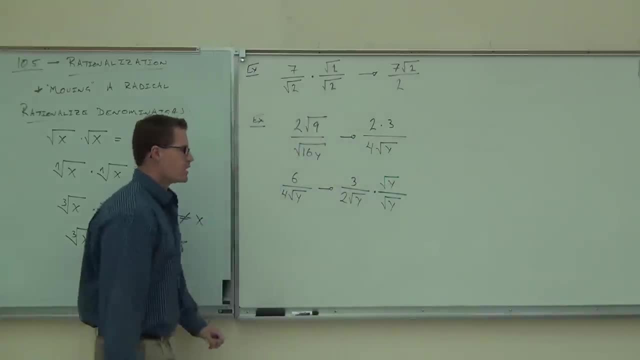 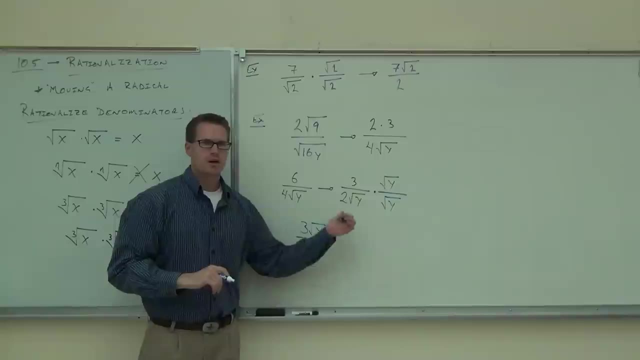 That would work. Let's see why that works. On the numerator, I'm going to have 3 root y. We've done that a lot- 3 root y, nothing else I can do. On the denominator, am I still going to have a 2?? 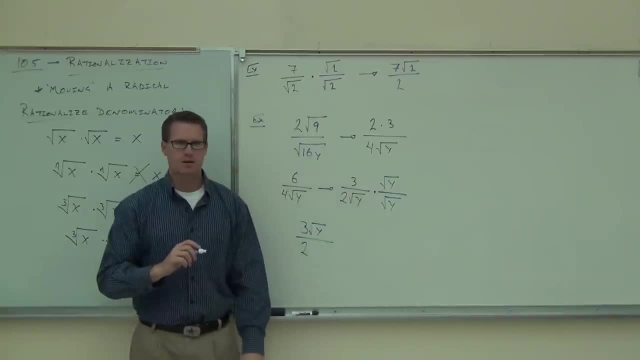 Yes, Am I still going to have a root y? No, No, No, Right. so the root y. This is a view of north top 2. times root y, times root y. The root y's are what I care about, right. 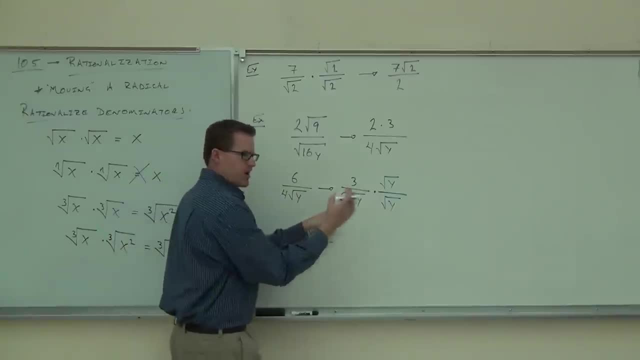 I don't care about the 2's, which is why we don't have another 2.. This 2, that's fine, that's great, but I'm looking at root y times. root y, That's giving you just y. 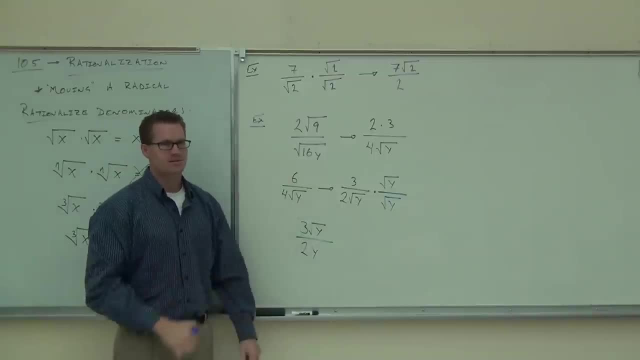 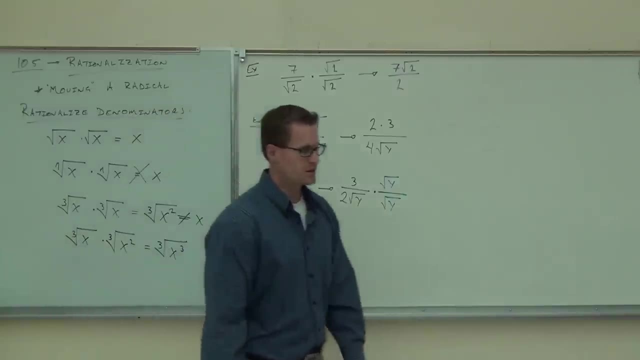 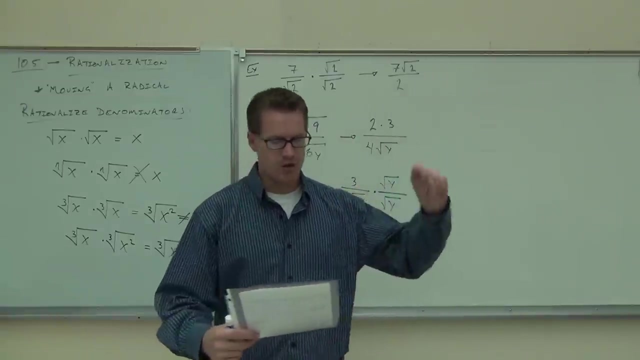 That's why we do that Now. can you simplify anything else in this problem? Can you simplify these y's? No, No, you can't. You're going to start seeing patterns also when you start simplifying, of simplifying square roots, where numbers go also. 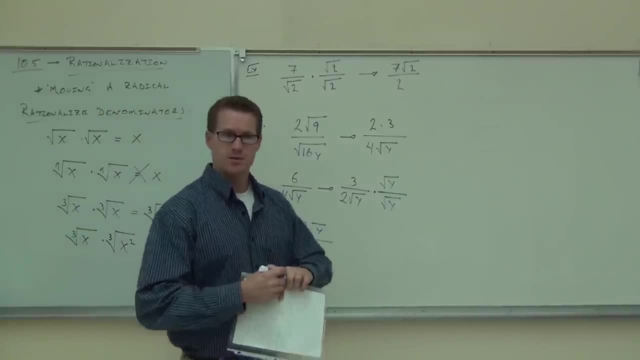 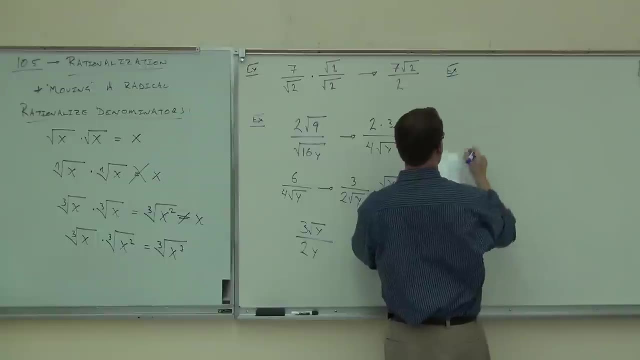 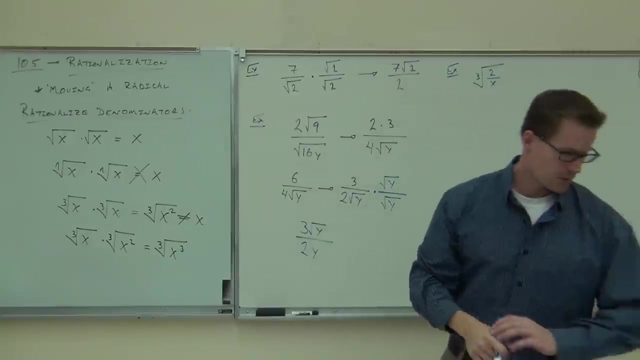 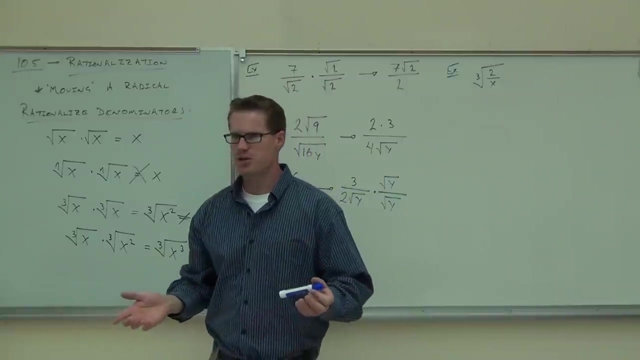 We're going to try something a little bit different. No, Too bad, The cube root 2 over x. Now wait a second. Mr Leonard, I thought we were supposed to be rationalizing here. I thought we were supposed to have something on the denominator. 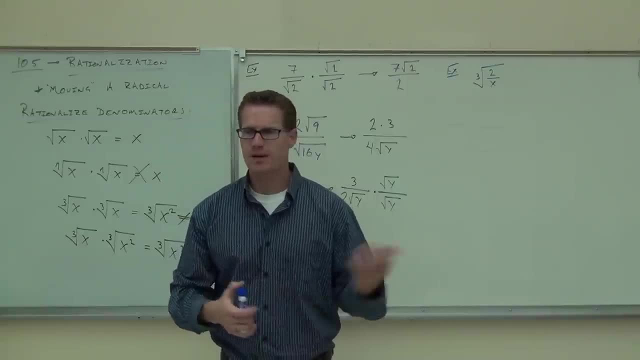 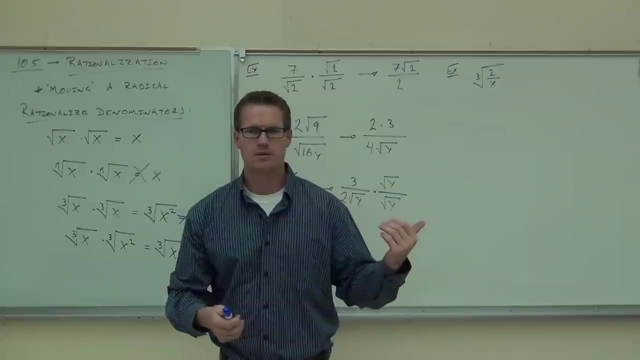 a root on the denominator and then move it to the numerator. But do I even have a root on the denominator? I do, Oh. so we say yeah, Why do I have a root on the denominator? Because you could bring the root to 2.. 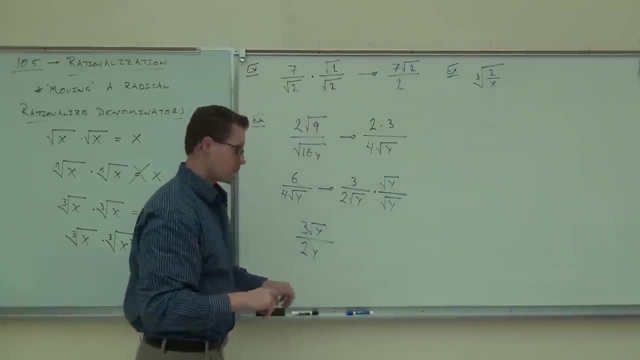 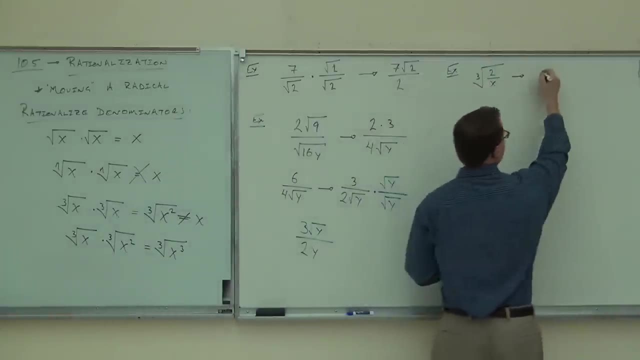 I could. So when you get this problem, you still do need to rationalize, because right here this really says it's not really the cube root of 2 over x. I could write it as the cube root of 2 over the cube root of x. 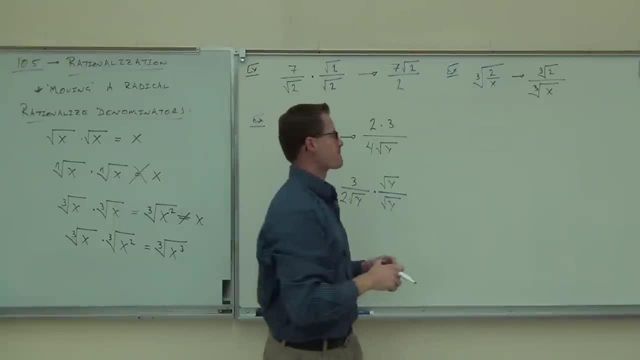 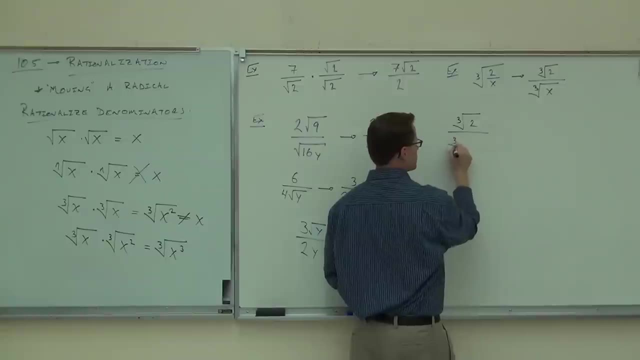 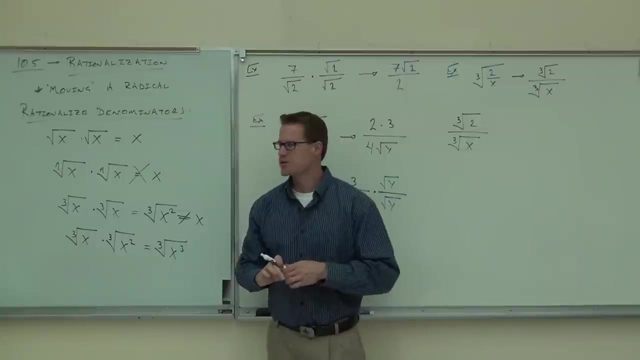 You believe me? Yeah, Okay now. Now I'm going to rewrite this down. I'm going to write it down here. So same thing, Just a little bit bigger. Cube root 2, cube root x- I'm trying to rationalize which one. 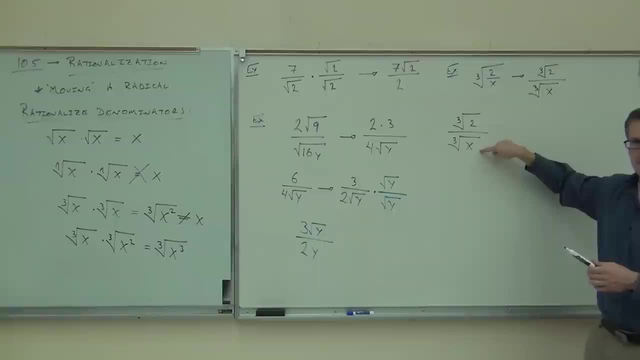 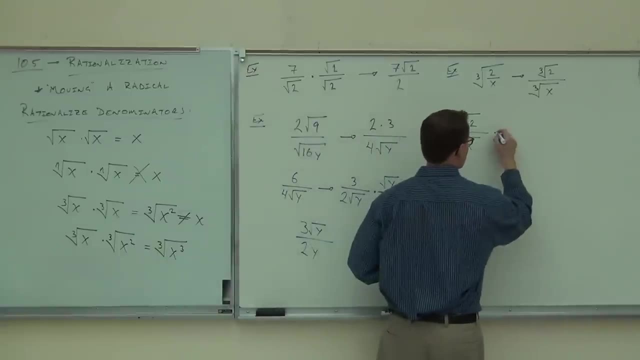 So am I trying to get rid of the root here? No, Here, Yeah, Yeah, okay, I'm still going to multiply it by something. That's the only way you can get rid of a root. Here's the question. We talked about it just a little while ago. 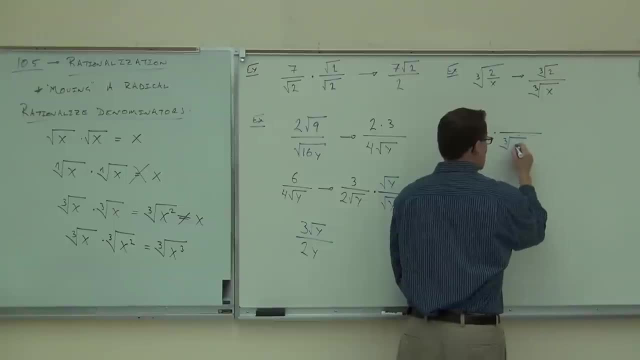 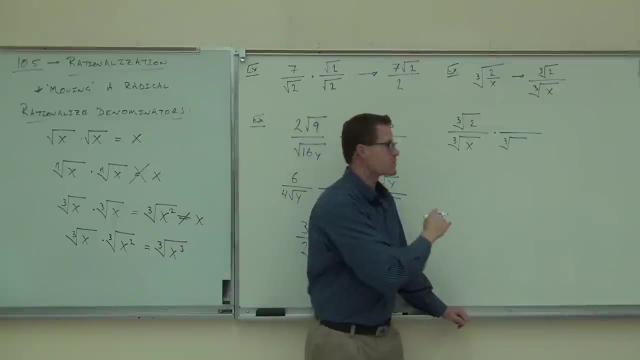 In fact, this is on the floor. If you're not really paying attention right now, you're probably going to think that the same thing that we did is going to be the same thing we're going to do here, But I want to show you again. 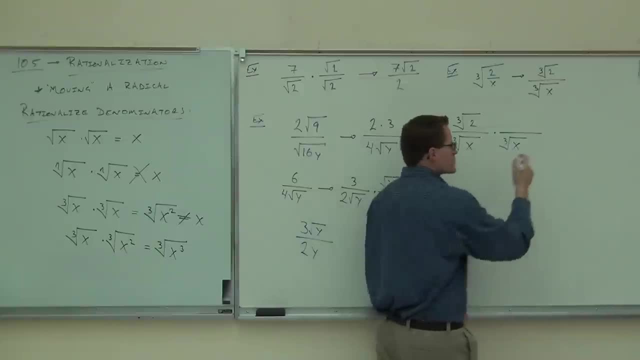 Is that going to work? No, No, what's going to happen is that this thing, this thing would give you the cube root of x squared. Does the cube root of x squared actually simplify out of this expression? No, You have a problem here. 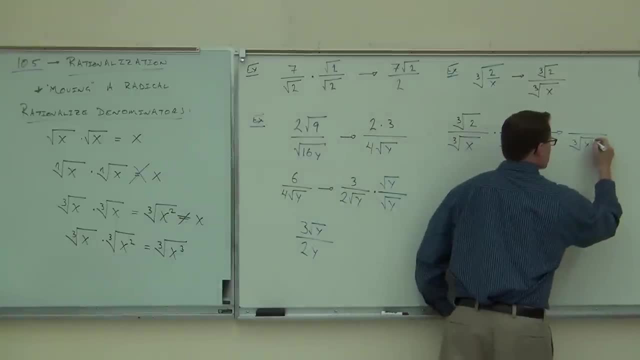 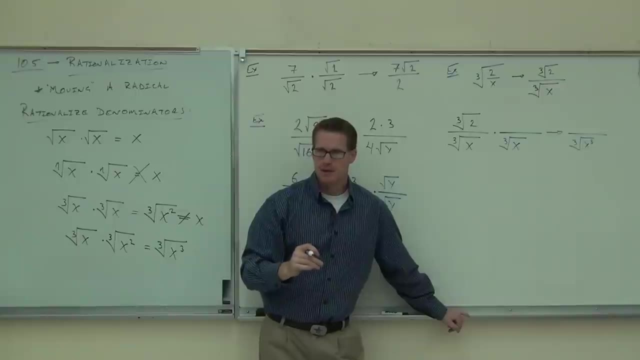 What you want to happen Is the cube root of x cubed. So you really have to notice what type of root you're dealing with. If it's a square root, things are pretty easy. You just multiply by whatever root is there. 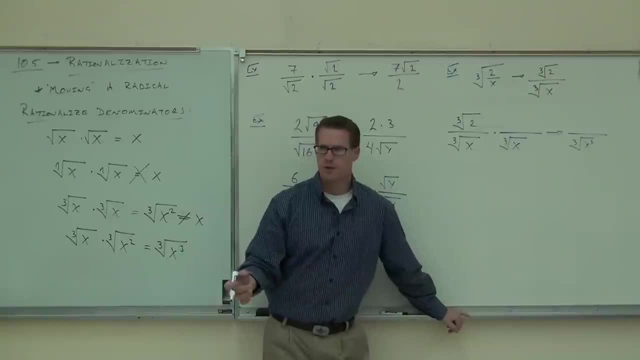 That's nice. If you don't have a square root, you have a cube root, a fourth root, a fifth root, whatever you have to match up the power of the root. That's how we simplified radicals in the first place. 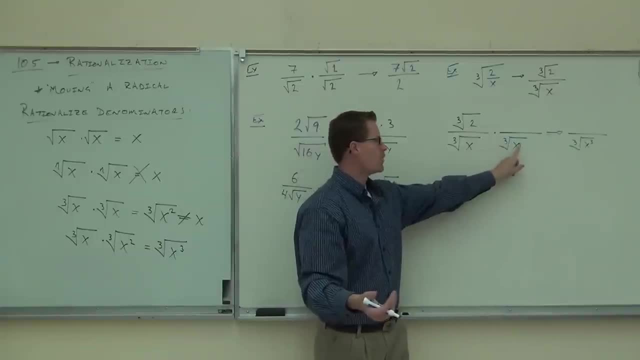 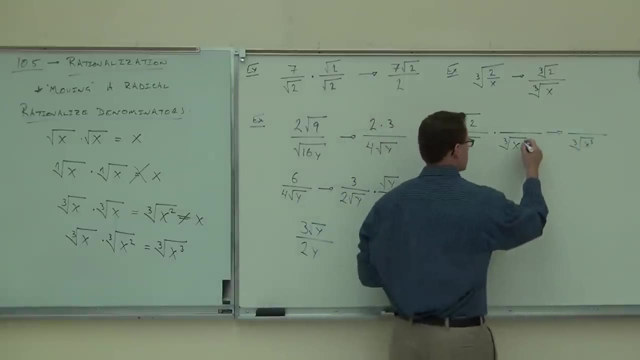 So, instead of the square, the cube root of just x. what needs to go here in order to make that? Because that's what you want. You want x squared, X squared. Does this make this? Yes, That's what I want. 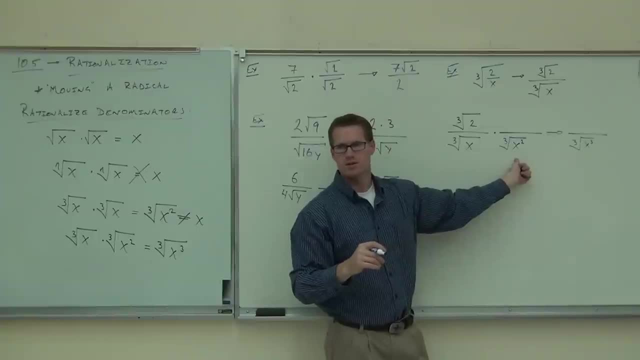 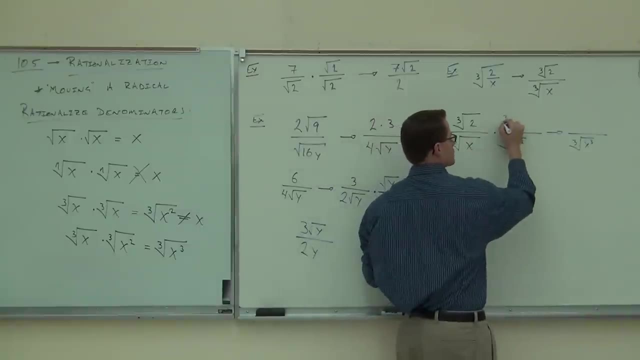 Now, whatever you have here, just like you're making equivalent fractions when you did add and subtracting, you're doing the same thing up here. You have to multiply the same exact thing, So this becomes cube root of x squared as well. 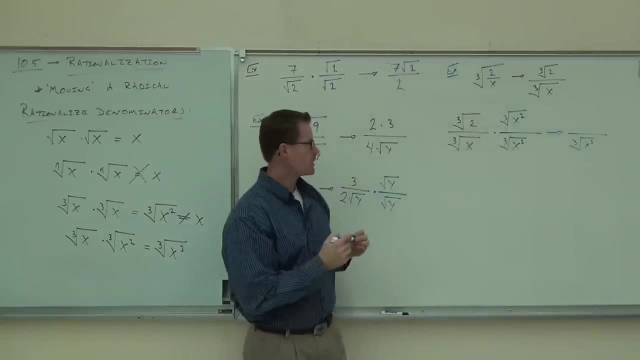 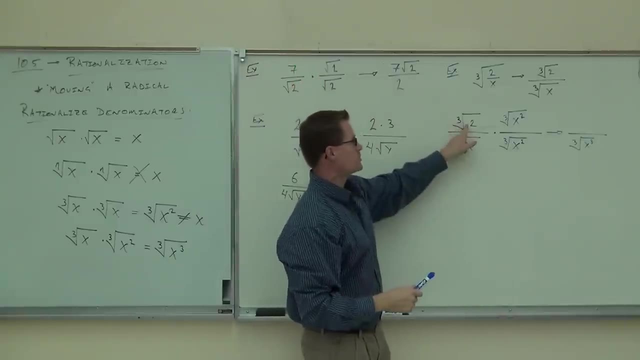 It's got to make a 1.. It's got to be 1.. I'm sure you're going to feel okay with this. Why do you have to add a square there? Do you understand why? Okay, Now I have a cube root. 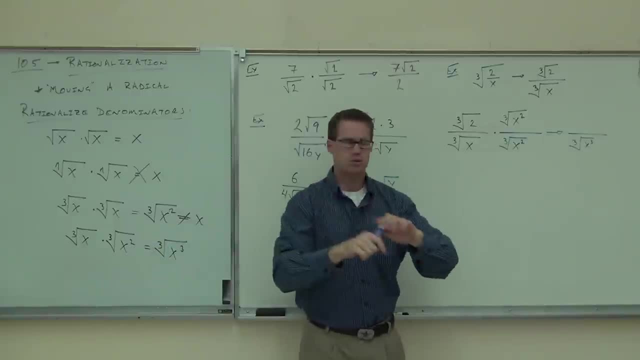 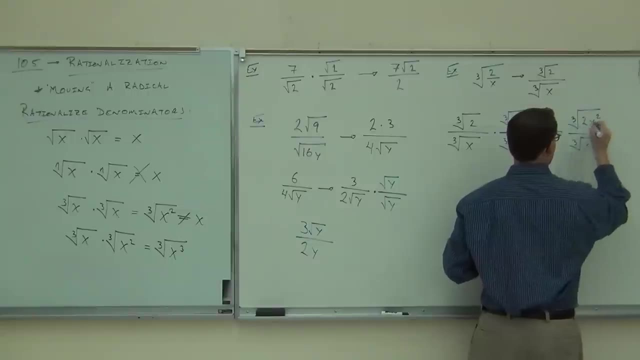 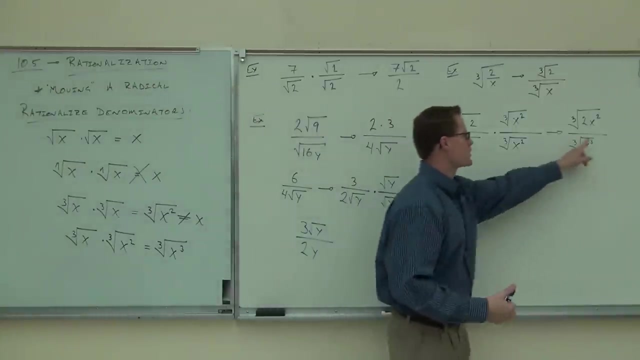 and a cube root. Can I make that one cube root? Sure, Let's do it. I've now got the cube root of 2x squared. Lastly, we're going to simplify whatever we can. You'll notice that I'm doing an extra step here that I didn't do on my square root. 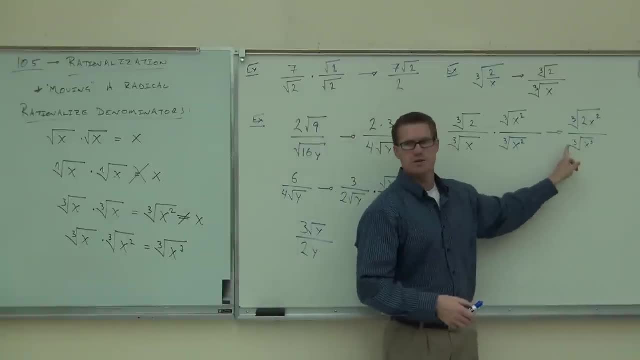 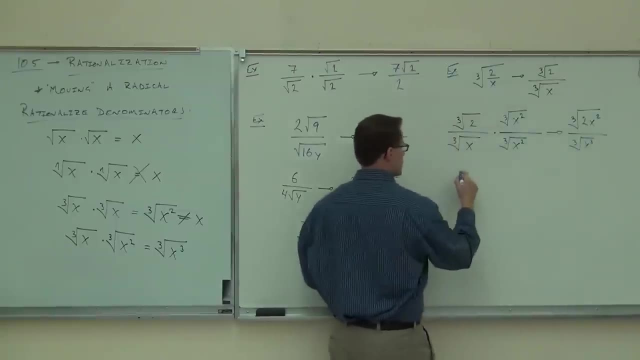 so you see what's happening. What is the cube root of x cubed? Can you tell me Square root of x? That's why we did that whole step, because we knew we wanted to match the power of the root. If we do that, we get a cube root of x squared. 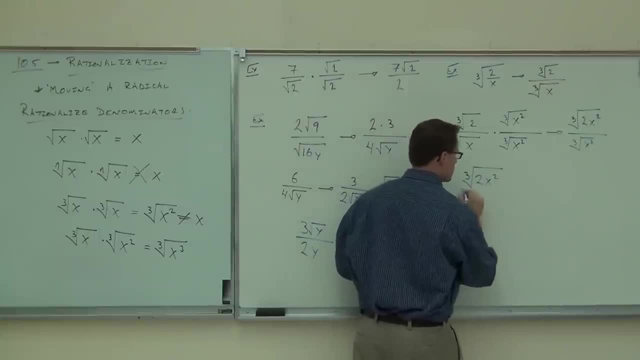 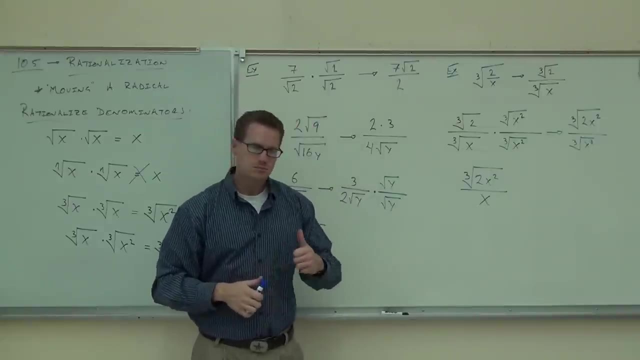 That's a cube root of 2x squared all over x. What are we successful at getting rid of? the root on the denominator of our fraction? A big one, Yeah. One more thing I want to show you before I let you go here. 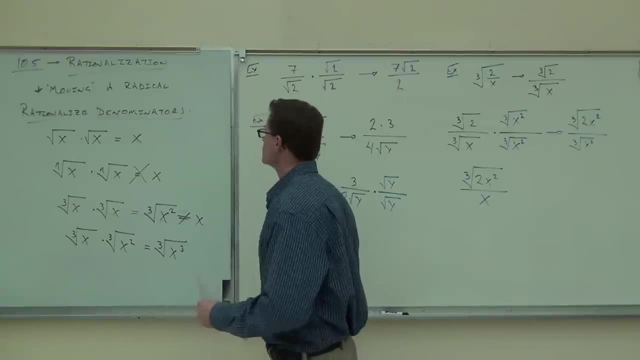 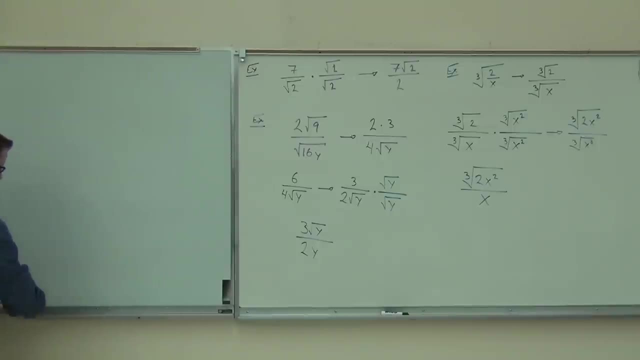 We'll start with examples of this next time, which you're going to do. If you're ever faced with двухamperes, That's a big one. That's a big one with doing a root like this. if you're ever faced with that, 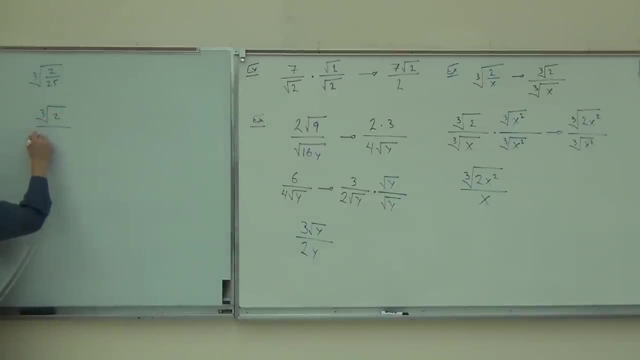 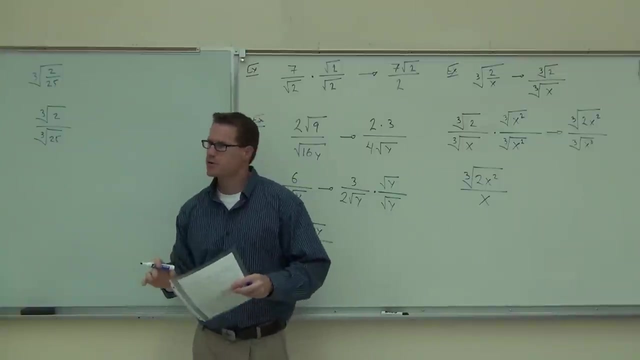 Of course you are going to break it up in the same manner: square root of 2 over the, I'm sorry, the cube root of 2 over the cube root of 25.. Now the cube root of 25, it's going to be very difficult. 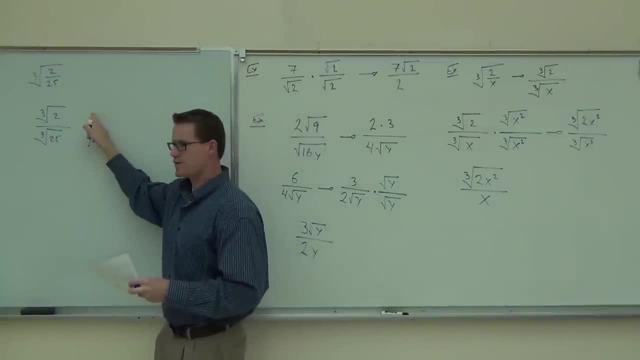 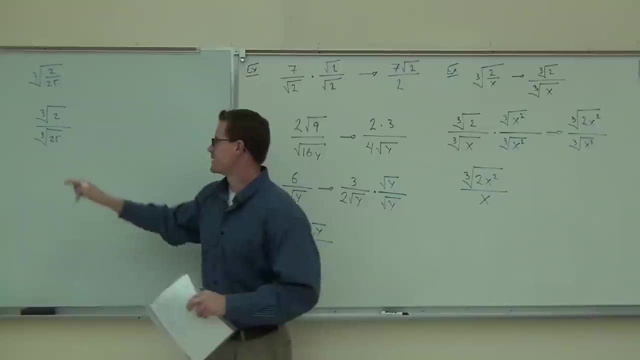 if you go ahead and you multiply this by the cube root of 25 squared over the cube root of 25 squared, It's a huge number. Instead, what I'd like you to do, see if you can make this a little bit better. 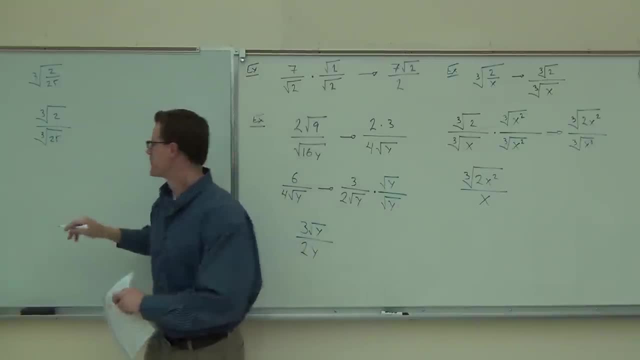 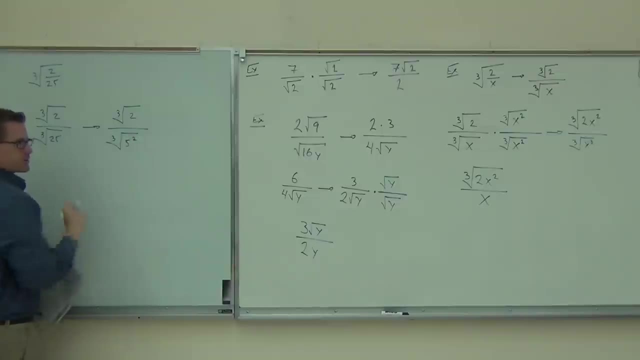 Watch. Instead of thinking about this as 25, maybe I think about this as the cube root of 2 over the cube root of 5 squared. Does that work for you? Is that still 25?? Then, instead of multiplying by the cube root of 25 squared. 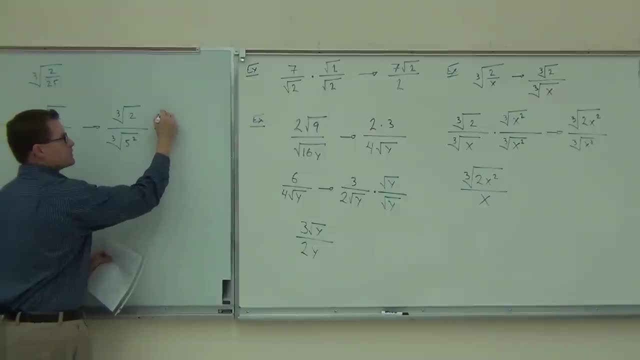 over the cube root of 25 squared. all I've got to do check this out. okay, what I want out of this is something over the cube root of 5 squared. I want 5 cubed. Do you see why? 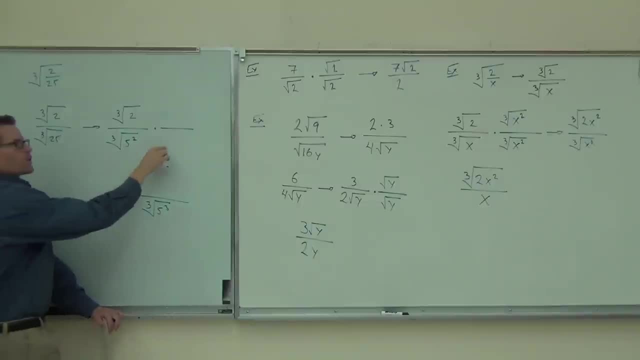 I want 5 cubed because I want the power to match the root. What do we need to multiply by in order to get 5 cubed? Yeah, just do that. That's a lot better. It's a lot easier. Instead of having 25 squared in there, you simply have 5.. 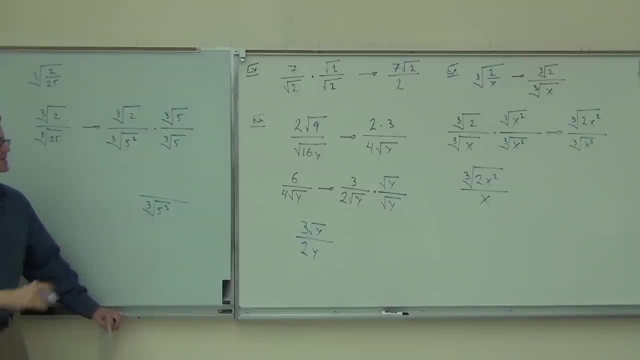 625 versus 5, okay, you want 5.. Does this make sense to you? Yes, So try to simplify that. first, maybe write that as a power, and then you have to multiply by something much smaller. This notice does make 5.. 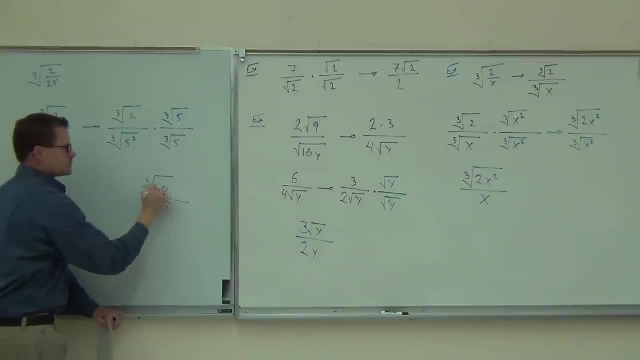 If you multiply by 5 cubed, this is going to make the cube root of 10, 2 times 5, that gives you 10.. Cube root- and the cube can't simplify out- You get a cube root of 10 over 5, and that's as far as you can go. 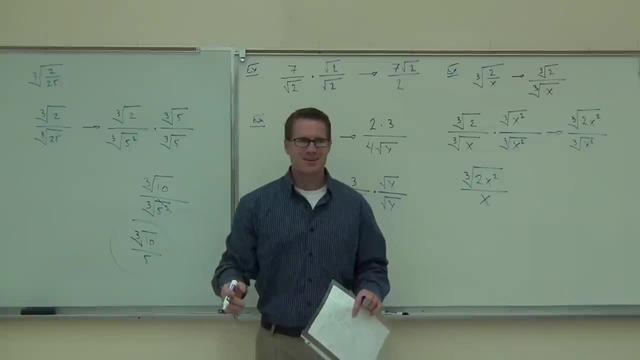 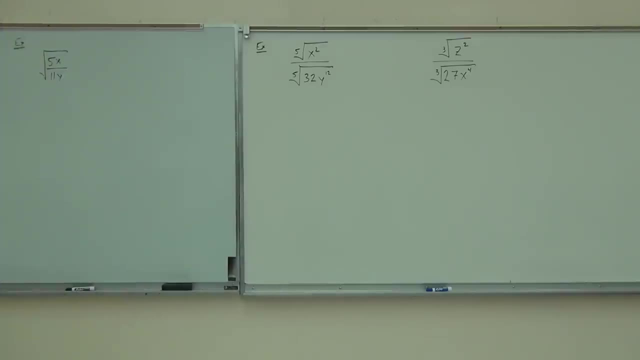 You can't simplify the 10 and the 5,. you're done, Do you follow? Yeah, I'm going to feel okay about this. so far, All right. So, if you remember from last time, we'll rationalize, which means remove the denominator's square. 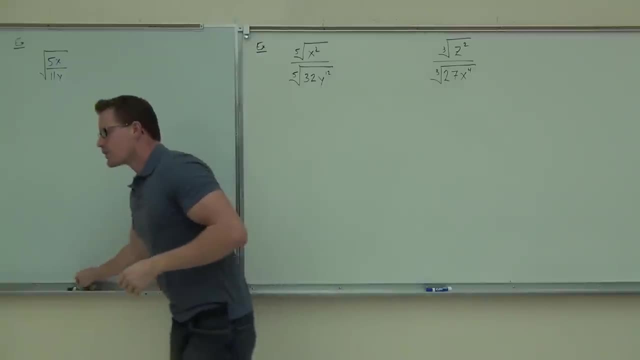 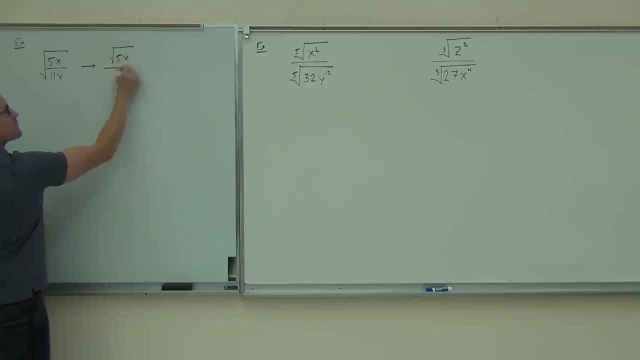 root or whatever root you have. So in our first example we're learning that. well, of course we do have a root on the bottom of our fraction because we know by the quotient rule we can separate this as the square root of 5x over the square root of 11y. 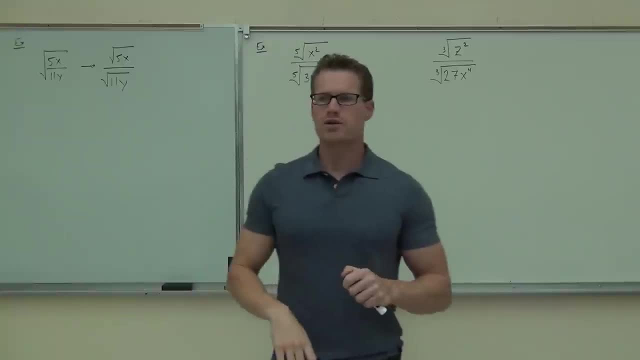 Now, if I ask you to rationalize the denominator, are we trying to remove the root on the top or the bottom of our fraction here? Okay, so we're trying to remove the square root of 11y. We also learned from last time. are we going to be able? 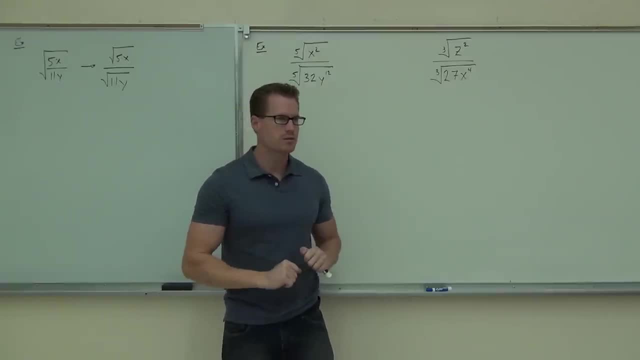 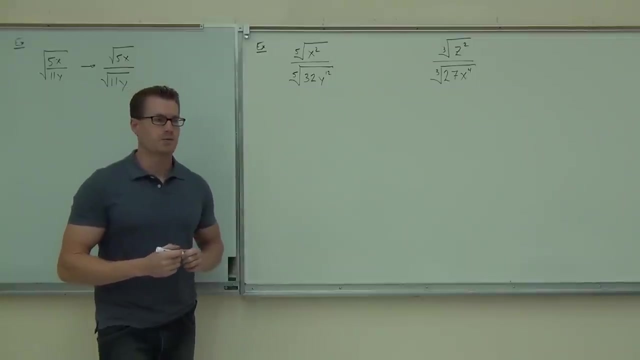 to eliminate roots altogether with this or just move them around. So we're trying to eliminate the square root of 11y. Can you tell me what I need to do in order to eliminate the square root of 11y? Well, we can't divide anything. 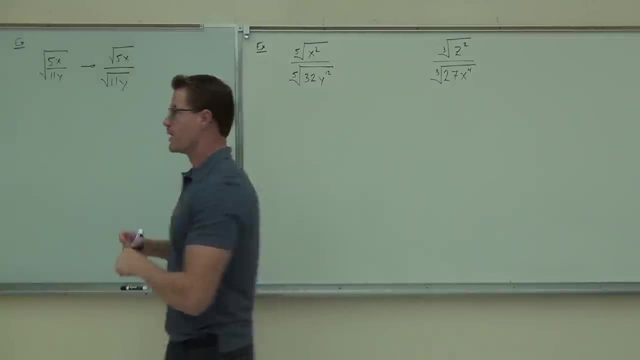 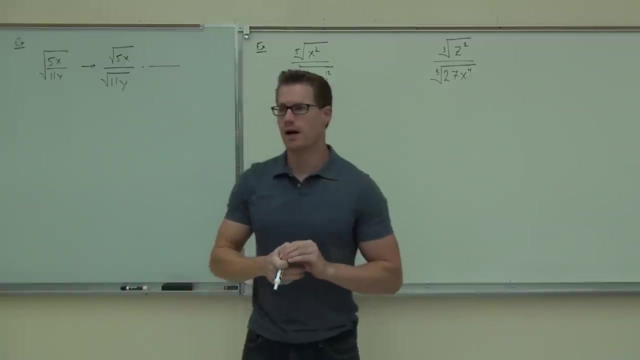 We're not going to be dividing, We are going to be multiplying. What specifically do I need to multiply by in order to get rid of the square root of 11y? What do you need to do? What do you know about square roots? 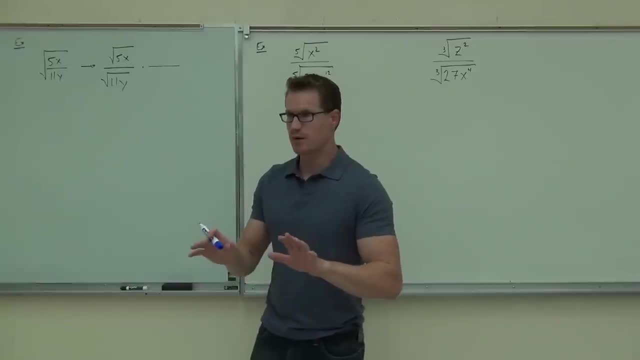 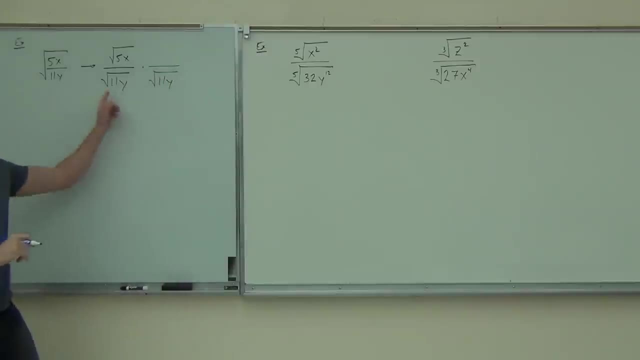 If I use the exact same one, The exact same one with square roots? Okay. So if I multiply by the square root of 11y, is that going to get rid of the root? Yeah for sure, Absolutely. Square root times itself gives you the radicand. 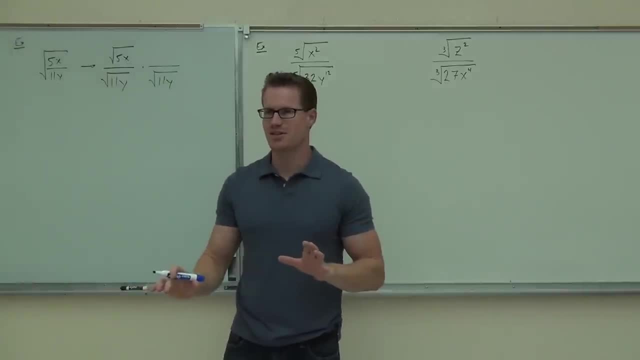 You guys need to be with it today. You look a little unfocused, to be honest with you. You're just kind of sitting there. I need you to participate and be with it today, even though it's early in the morning. This is our class. 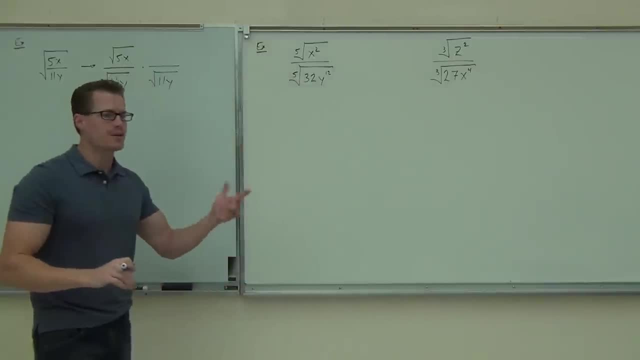 So When we have square root of 11y times square root of 11y, we know that that's going to eliminate that square root for us. Is this appropriate to do it just like that? Where else do I need the square root? 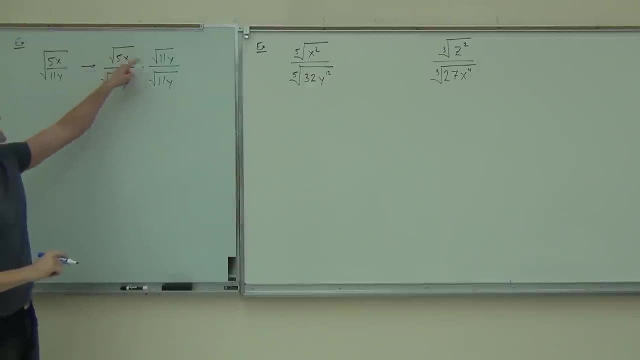 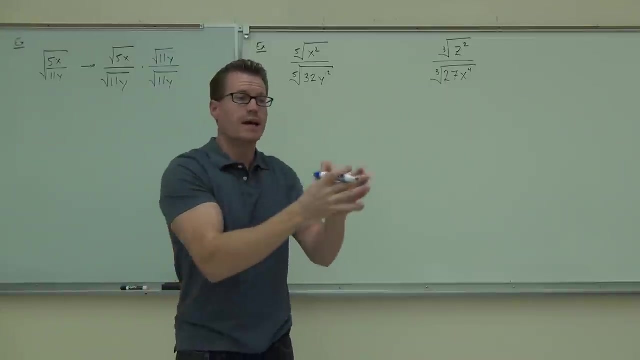 Now let's see what happens. Folks, square root of 5x times square root of 11y. can I make that under one square root? Sure, absolutely. If it's square root times the square root, I can do that. 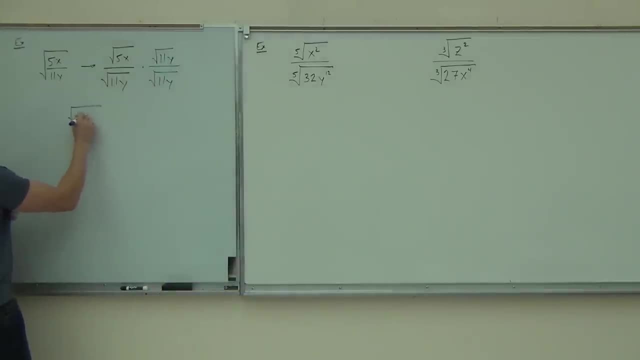 The product rule says: I can make this the square root of 55xy times the square root of 11y. Are you seeing where the 55xy comes from? That's cool, because we have two square roots. That's all right. 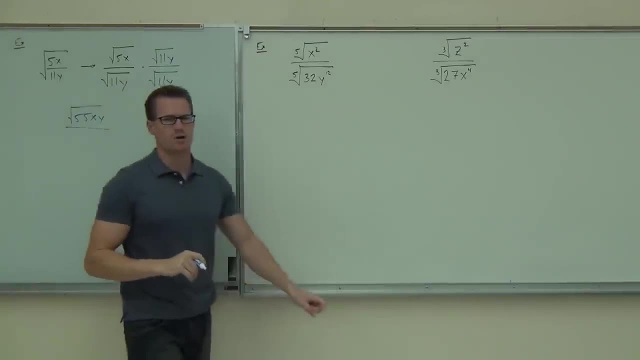 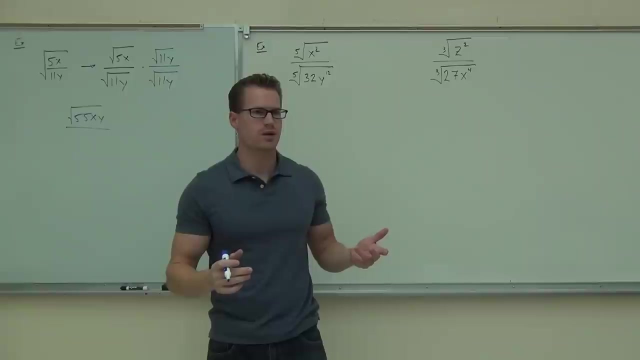 Now, how about the square root of 11y times, the square root of 11y? What is the square root of 11y times itself? How much does that give you? Yeah, Do you need to do the square root of 121y squared? 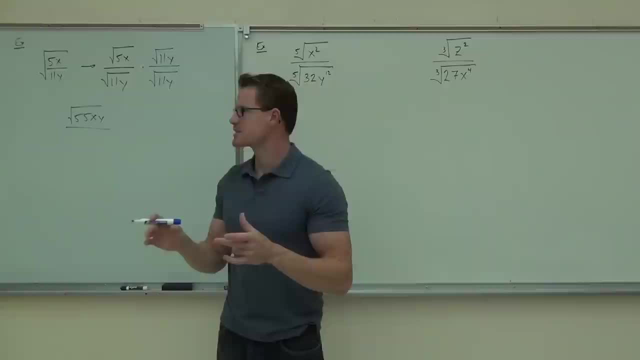 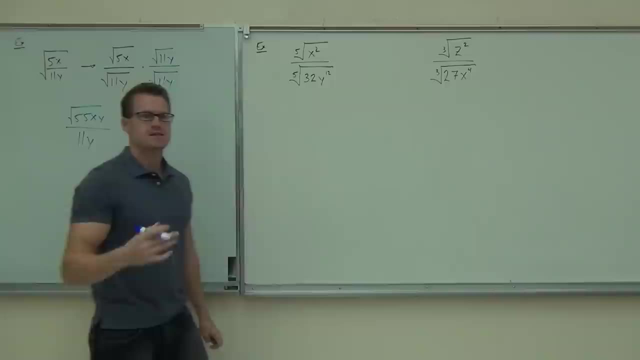 No, forget about it. You have a square root times itself. That's one of the main things I'm teaching here today is a square root times itself gives you the radicand, So here we'll get 11y, and that successfully rationalizes. 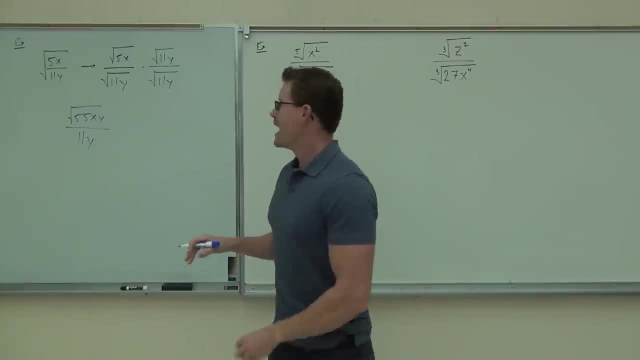 our denominator. We've removed the square root from the bottom of our fraction. Have we removed it all together? No, No, we can't do that. All we can do is move it around. We can only get rid of the square root if we have an equation. 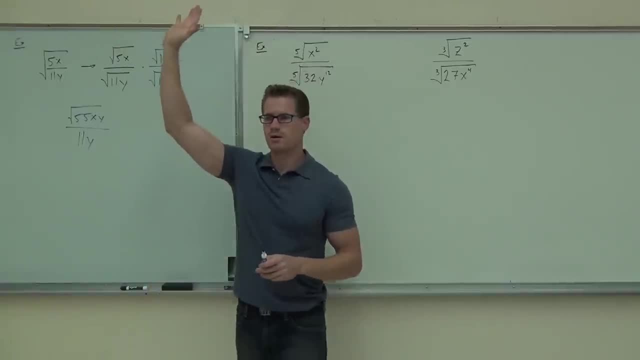 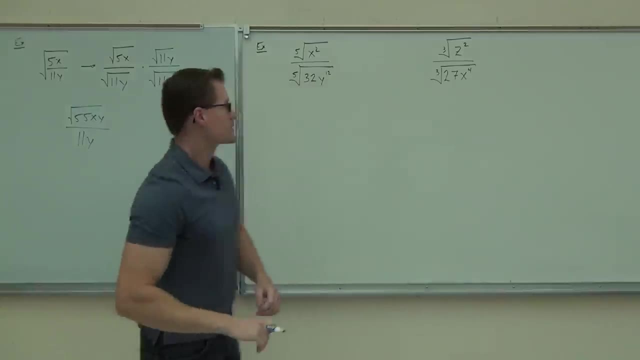 I'm going to show you that in the next section. How many people feel okay with this? so far? That's not a whole lot. Are you guys all right with this? People who are here and not walking the plate: Okay, next one. 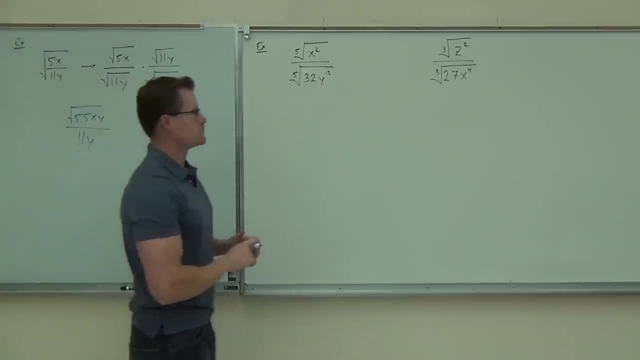 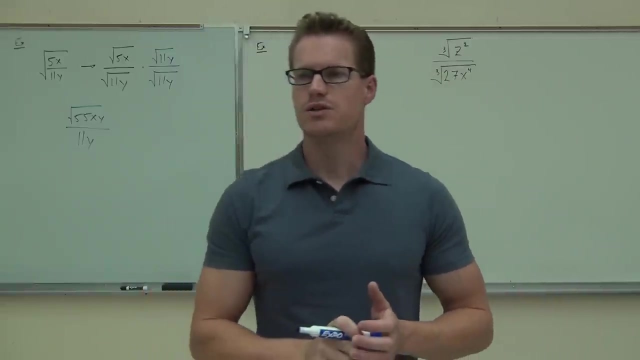 We've got the fifth root of x squared over the fifth root of 32y to the 12th. Oh my gosh, If I'm asking you to rationalize the denominator, let's start over. What does rationalize the denominator mean? 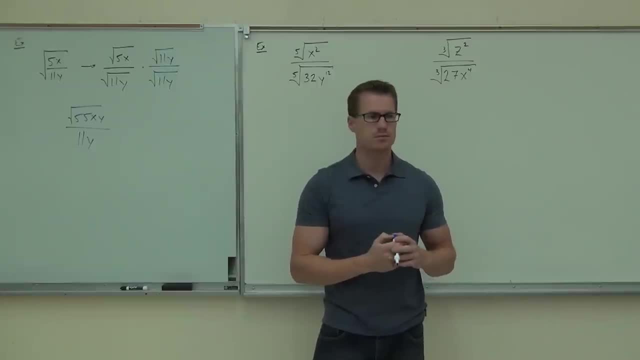 On the bottom. Okay, on the bottom. Sure, on the denominator, What root am I trying to get rid of here? Fifth root, Fifth root, Not a square root anymore. Hey, you know what? We learned something last time. 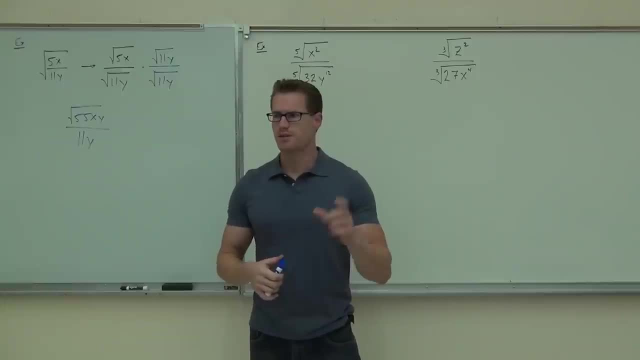 We learned that a square root times itself gives you the radicand. Does a fifth root times itself give you the radicand? No, That's something you have to know. Does a fifth root times itself give you the radicand? 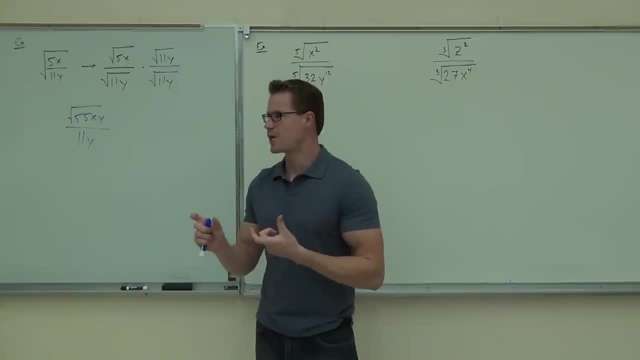 No, No. Now there's something weird that happens to those powers. right, We need to match up a power with a root in order to simplify it Here. that's nice, because a square root times itself gives you something squared. A square root simplifies something squared. 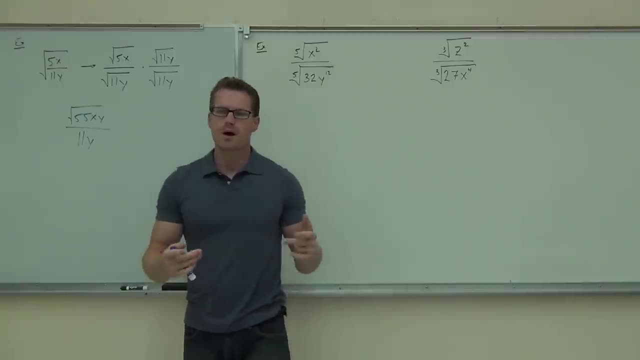 That's great. That's why that worked the way it did With a fifth root. what I would be getting is, if I multiply it by itself, I'd be getting a fifth root of something squared. And we know a fifth root really doesn't simplify something squared. 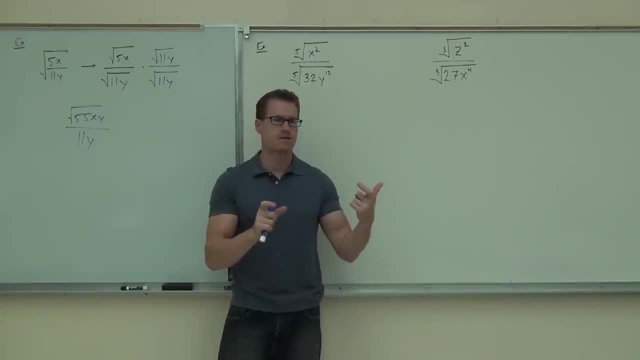 It has to have the power matching up with the root. Nigel, I don't know if you're okay with that. All right, So, in order to simplify this, when we have to multiply by something, to give us a fifth root in there. 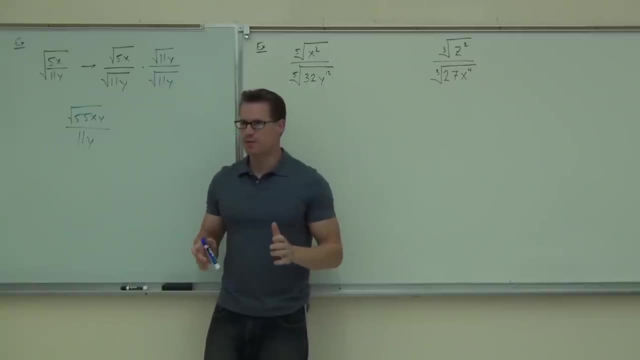 However, do you notice how we have 32y to the twelfth? I hope you do, because it's very little. We have a fifth root of 32y to the twelfth. One thing I told you about this when we first started was if you can simplify it, simplify it. 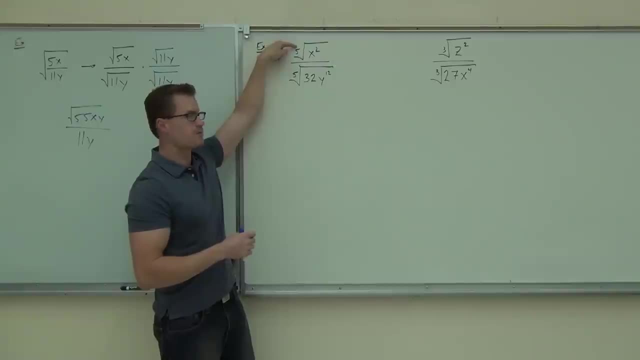 Can you simplify this one? Can you simplify this one? Absolutely do it. It's going to make your life so much easier. Absolutely do it. It's going to make your life so much easier because you're not going to have to simplify it later on. 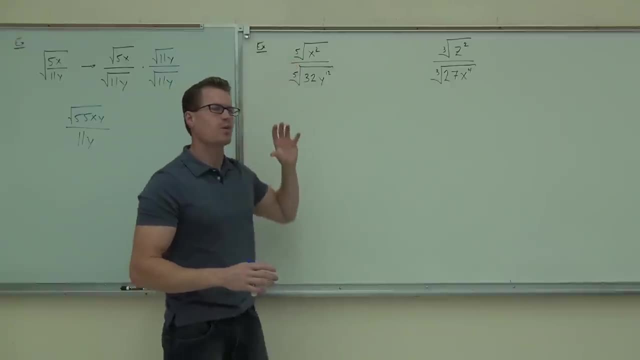 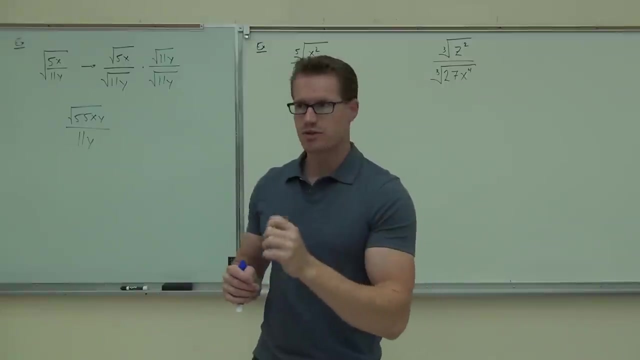 So what we're going to do now is, as soon as we see these problems, simplify whatever you can Now. now listen carefully. I know that some of these things seem contradictory to you because about three sections ago, I told you, whenever you see a root over a root, you combine them first. 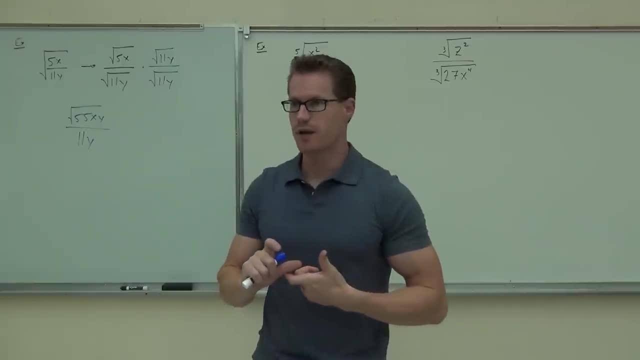 You remember me telling you that You do. You do when you're simplifying. When you're simplifying and you have a root over a root, you combine those things because you're going to be able to simplify. You're going to be able to simplify your like terms. 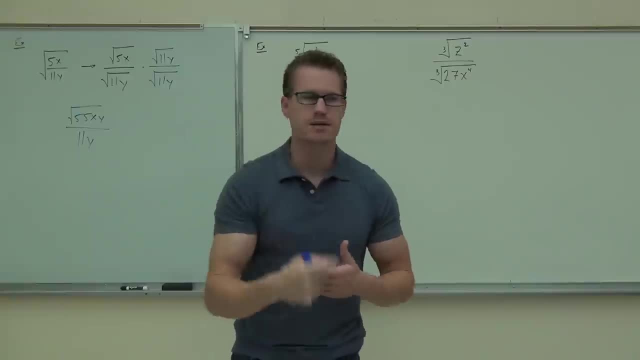 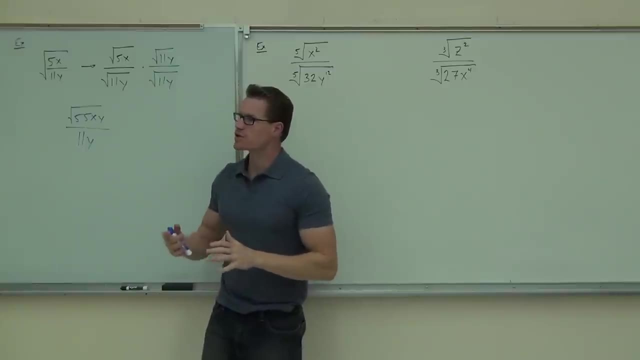 You remember that Your like x's and your like y's. Do I have any like x's, like y's or like numbers? Then that wouldn't do us any good. Okay, When we're rationalizing, we're doing something different than simplifying. 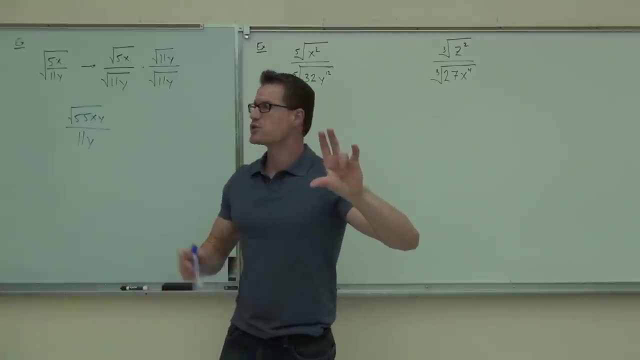 When we're rationalizing, we're moving around a root. When we're simplifying, sure, we're putting things together, crossing things out, and then we're simplifying. So there's a difference. Listen, there's a difference between simplifying and rationalizing. 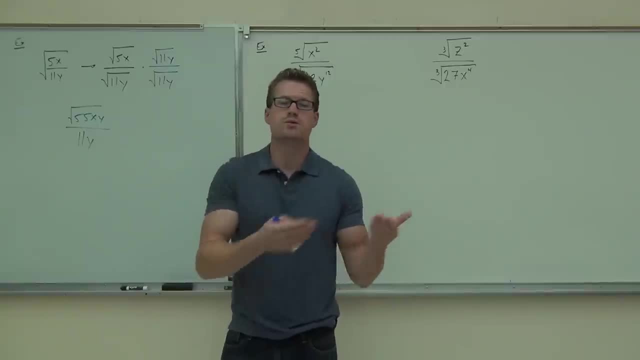 When you read one word, you know it. When you read another word, you do one thing. When you read another word, you do this thing. Okay, Rationalizing: you're going to be doing this process. You're going to simplify each one individually, then rationalize. 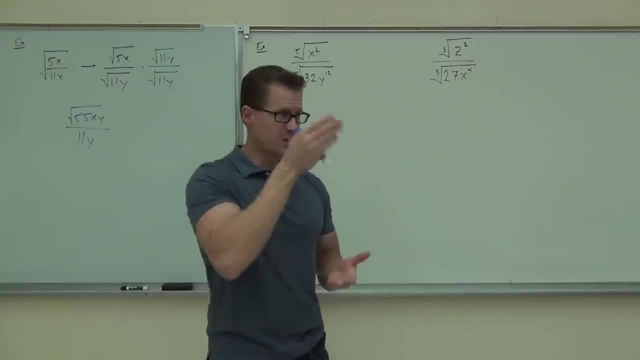 When you're simplifying, it's different. You do put them together, You simplify what you can and then you simplify that radical as a whole. Are you seeing the difference here? Okay, so yeah, it's a little bit, I don't want to say tricky. 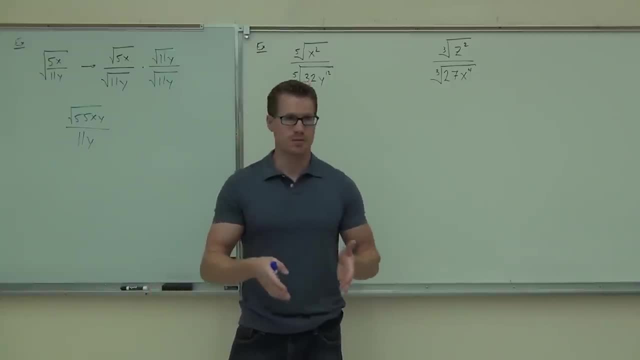 It's not tricky. Each thing has its own little process, but that gets confusing to some people, And so I want to make you aware that we're doing several things in this chapter. You need to be paying attention up here, Okay. 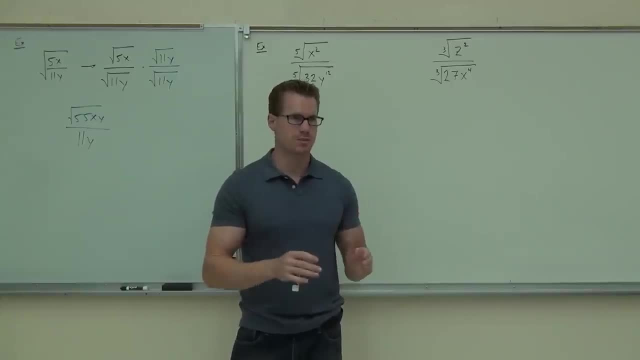 Okay, We're doing several things in this chapter that look very similar, very similar. If you're not really with it and you're just going: oh, I can do that right now. but then you learn something else that looks similar, you go, I can do that right now. 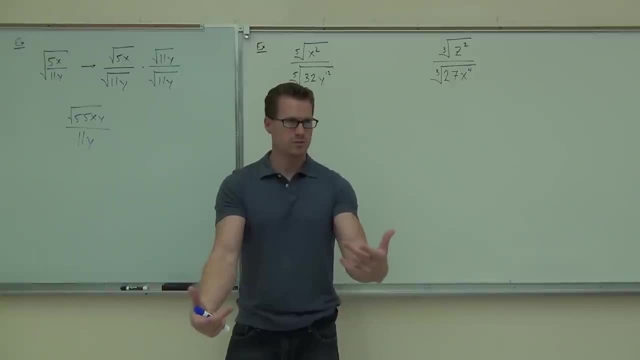 And I ask you, with those questions next to each other and one thing you do, or one question you do one thing on, another question you do another thing on. it's going to get pretty confusing, right, if you really don't know it. 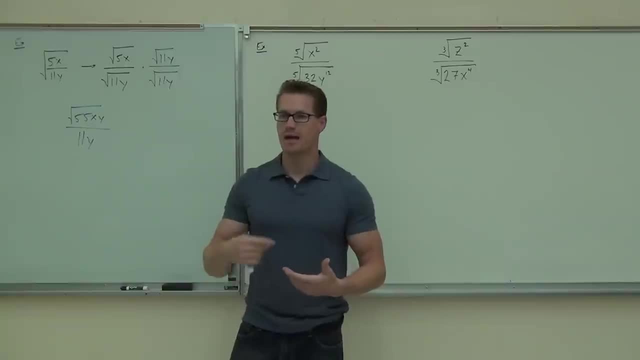 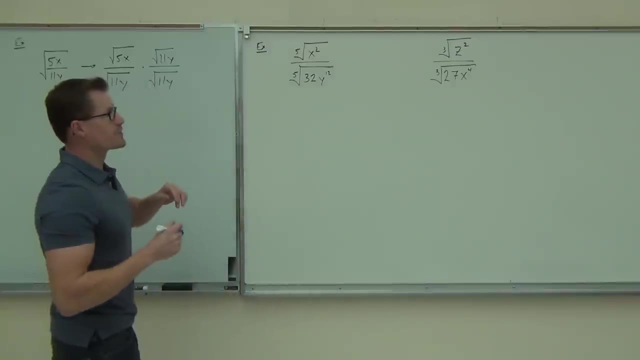 So right now is the time to start spiraling this information, going back and start studying for your test now. I know it's in two weeks. Start studying, I know it's in two weeks, Okay. So with this example, yes, we're rationalizing, but we need to simplify first. 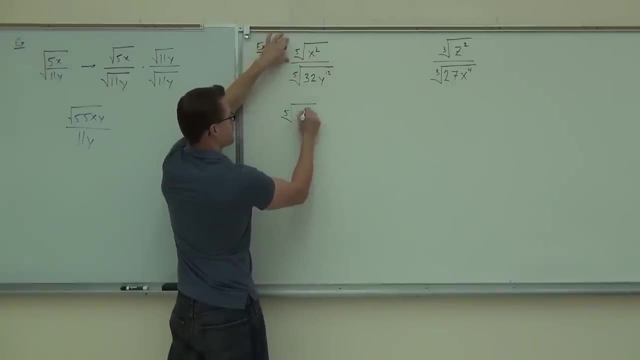 Now our numerator. yeah, we can't really simplify that Denominator, though yeah, we can simplify the 32y squared. Do you know what the fifth root of 32 is? Yeah, because two times five times gives you 32.. 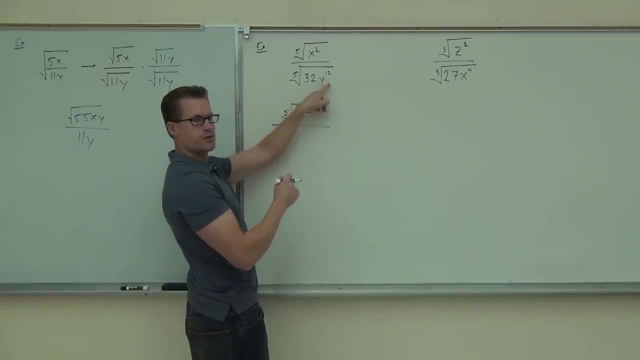 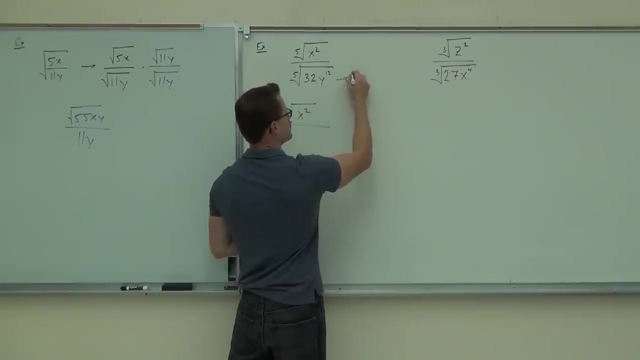 How about the y to the 12th? Can you simplify y to the 12th? y squared, y squared comes up. Why, no? Why is y squared on the outside and y squared inside? Okay, How am I going to break that up so that I can simplify it? 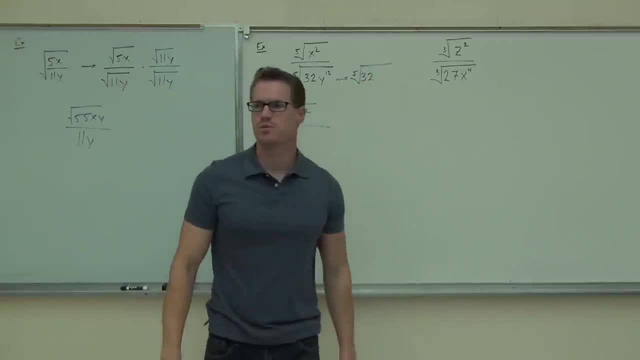 Of course, the 32,. I'm going to leave that. Let's break up y to the 12th and go through this process. y to the 12th. we should know how to do this pretty well. What am I going to write? y to the 12th as. 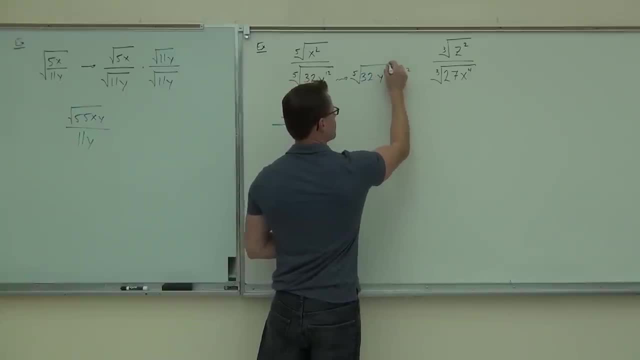 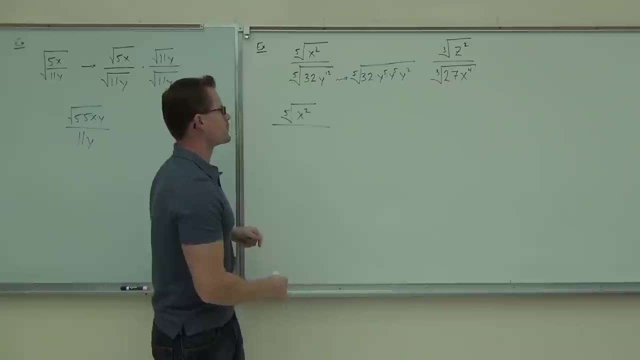 y, y to the fifth. Oh, we know the fifth power of y is going to simplify with the fifth root of y. That's why we're doing y to the fifth there. So in our expression here we'll have remember, would you? 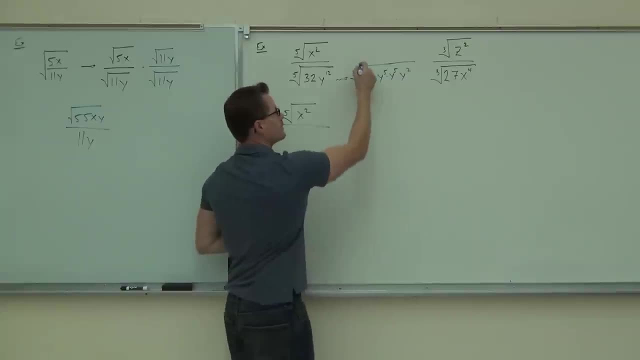 does this look familiar, by the way? I hope so. We've done that a lot. This gives you the two. This gives you a y. This gives you a y. We cannot simplify the y squared. You get a fifth root of y squared. 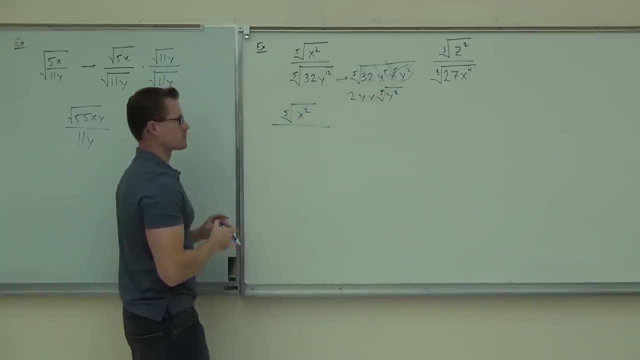 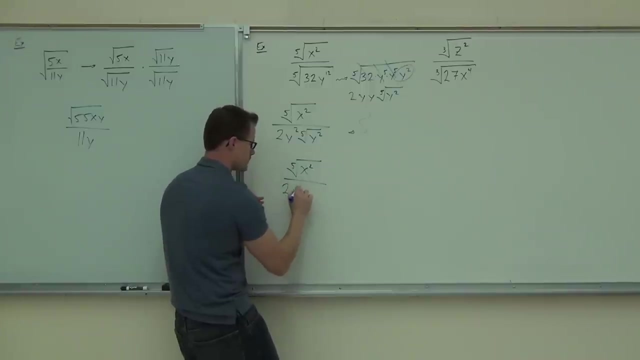 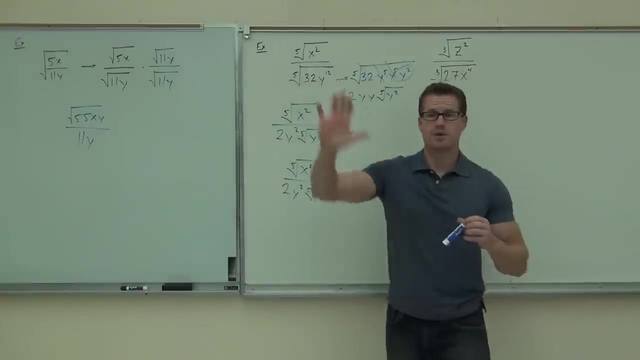 Don't lose that fifth root. So in our expression here we'll get two y squared, fifth root of y squared. I'm just going to rewrite this right here so I can use our rationalization later. Okay, Rich, do you feel all right getting down that far? 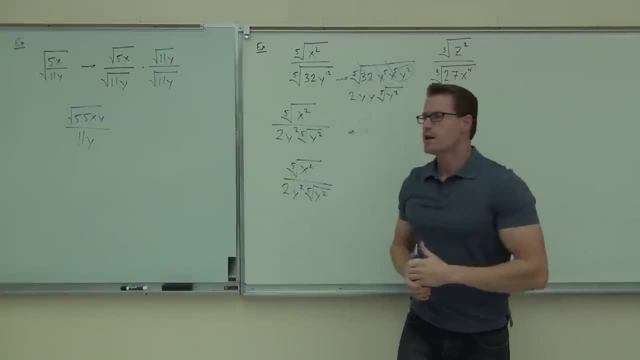 Good Guys on the left-hand side of the room, are you okay with this? Okay, good, Now we're going to rationalize. Can you please tell me now- well, now- that this looks a whole lot better, since we don't have a huge fifth root over here. 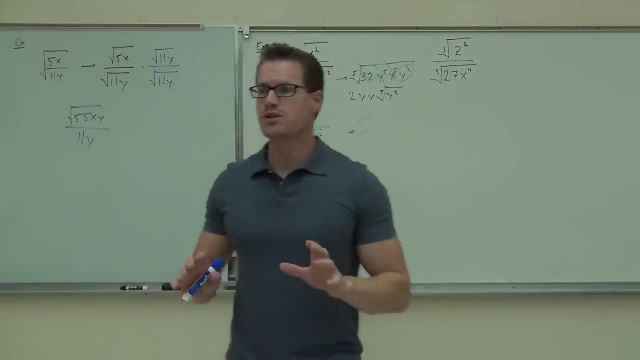 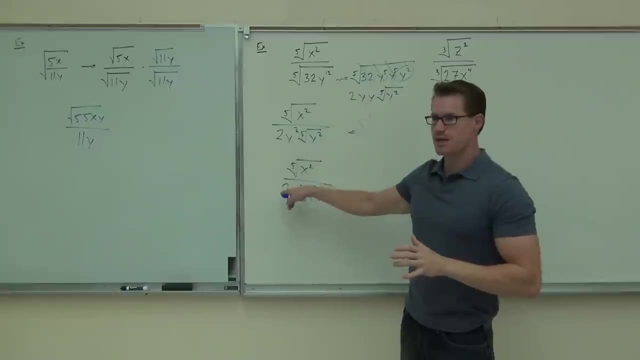 we just have to do this. We just have a much nicer fifth root. What exactly are we trying to eliminate here? Fifth root of y squared? Are we trying to eliminate the two y squared? No, This is why we did this: to make it easier on what we need to rationalize, so we don't have something so big. 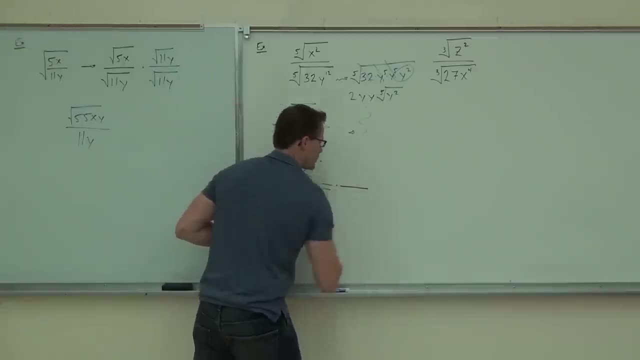 So if I'm going to rationalize the denominator here, it means I need to multiply appropriately. Now here's the deal. I need you to notice that if I multiply, I don't need to multiply by this at all. It's not in a root. 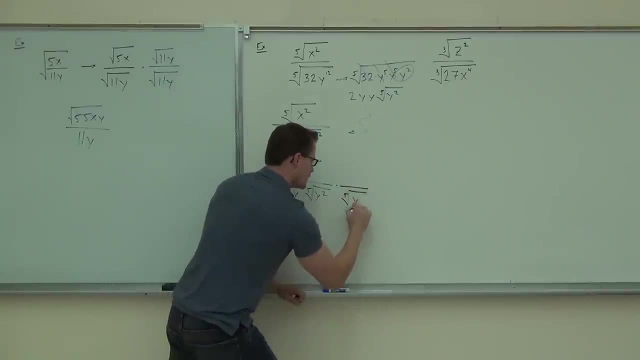 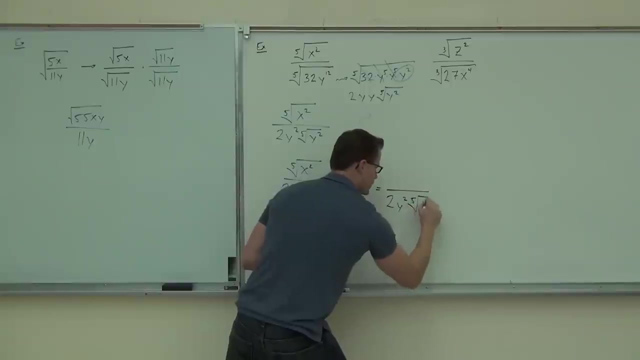 That's great. We don't need a lump. But if I multiply it by the fifth root of y, squared just like this, what's that going to give you? You're still going to have this two y squared, for sure, But inside of our radical you'd have a fifth root y to the fourth. 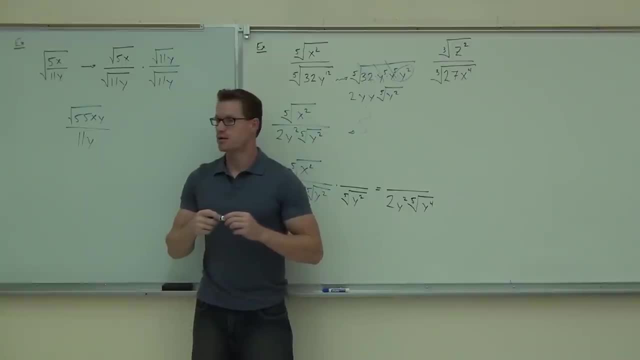 Are you agreeing with me? Yeah, Is that going to simplify it? Yeah. Are you with me here today? Yeah, I'm not getting hardly anything from you guys. I need more than this. Is that going to simplify it? No, 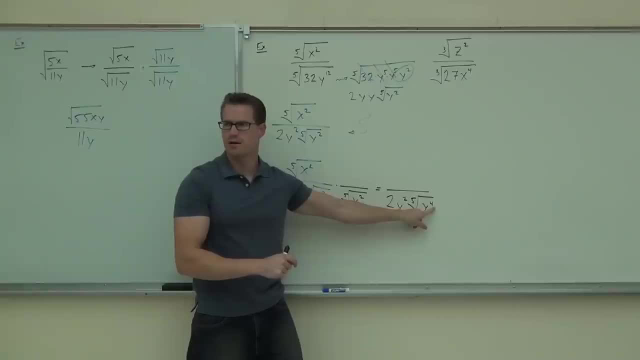 Okay, So what do you want that to be? so that it will simplify Y to the fifth. Yeah, we want that. If we want this, this piece is wrong. What does this need to be in order to simplify that Y cubed? 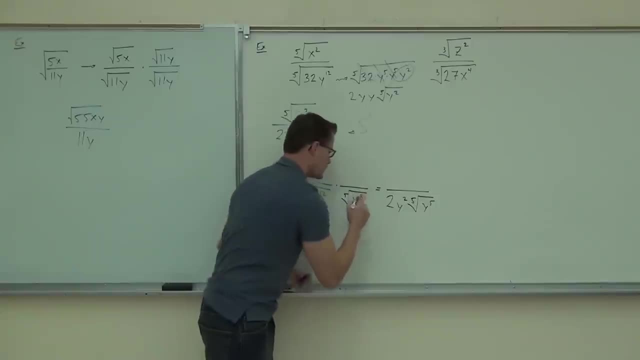 Okay, that's right. So y cubed. here we're going to be getting y to the fifth power. So on the right-hand side of the room, does this work when I just multiply it by itself for this? No. 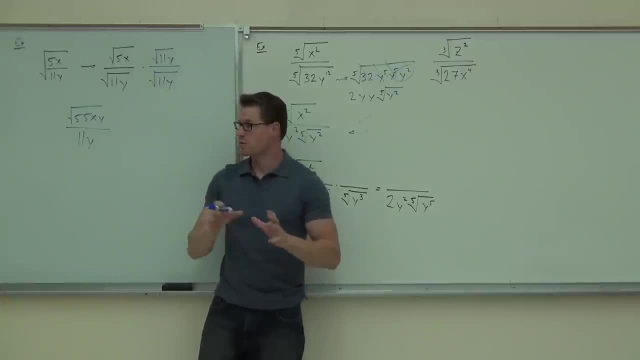 Okay, Does that work? No, You've got to be a little smarter than that, right, You've got to be a little smarter than the problem. You can't just do the same thing here that we did here, because you've got a different. 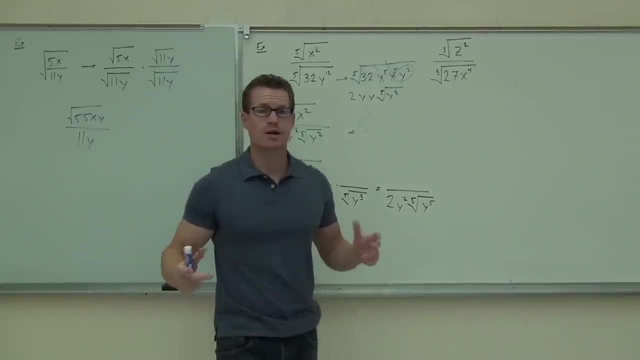 root. Square roots are great because you can multiply them by themselves and we eliminate the roots. However, when you get with the fifth root, you still have to match up the power with the root. So we've got to look at this one, figure out what we need to multiply in order to get. 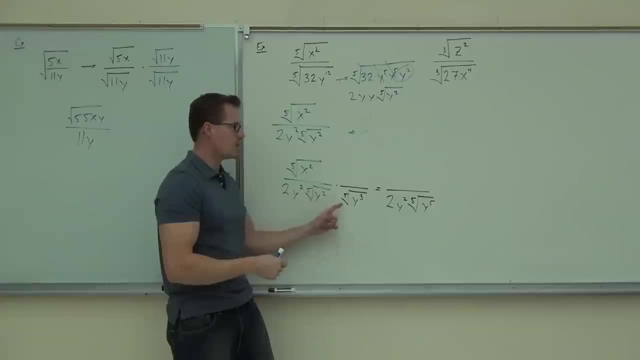 a fifth power in there. That's the way we're going to be able to simplify this expression. Same thing has to happen on the numerator, So we've got to look at this one, figure out what we need to multiply in order to get. 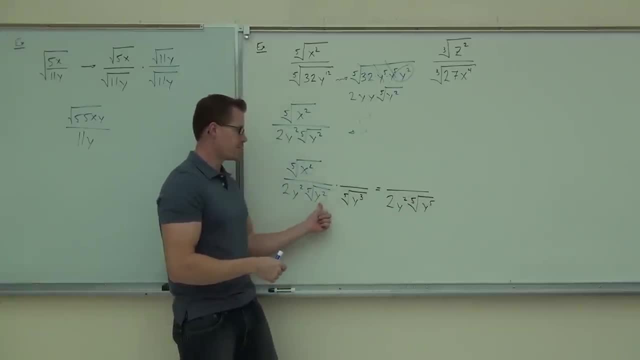 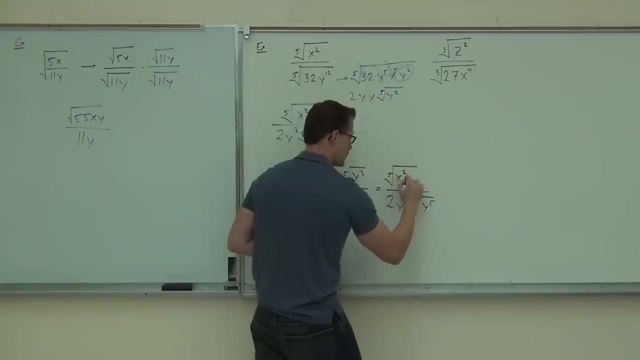 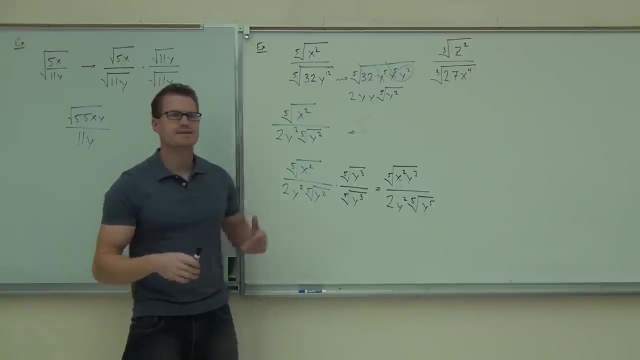 a fifth power in there. That's the way we're going to be able to simplify this expression. We'll be getting a fifth root of X squared, Y cubed. Last thing we're going to do is make sure that we have the same exact power and root. 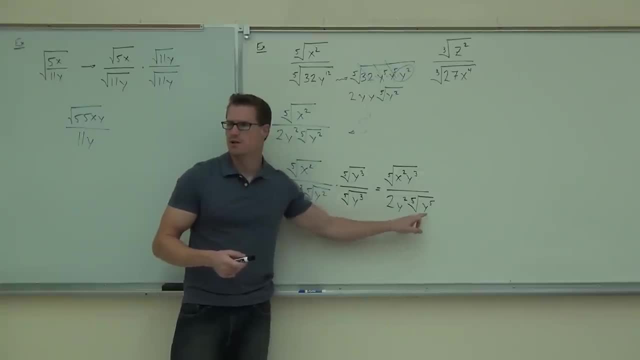 We'll simplify that. How much is this going to give us, ladies and gentlemen? Y Good. So let's see what we have. Fifth root: x squared, y cubed. We still have a 2y squared. That hasn't changed since this part. 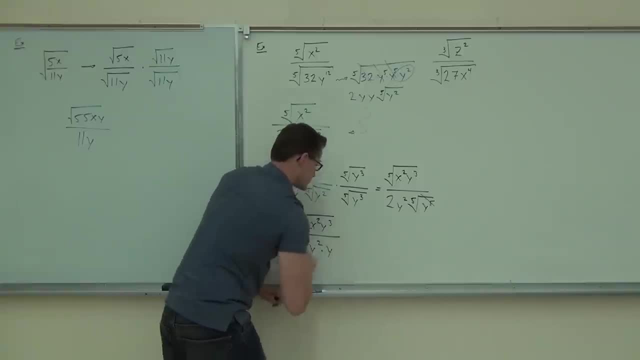 But this right here is going to give us a y. Of course we can write that just a little bit better. We'll have a fifth root of x squared y cubed And we'll have 2y cubed. Did we do it? 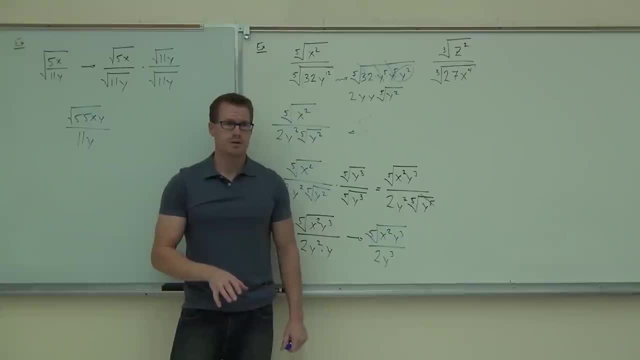 Did we successfully get rid of the fifth root? Yes, Not altogether, but on the denominator absolutely. How many people feel okay with this example? Good, All right, That's good, That's better. Why don't you try that one? 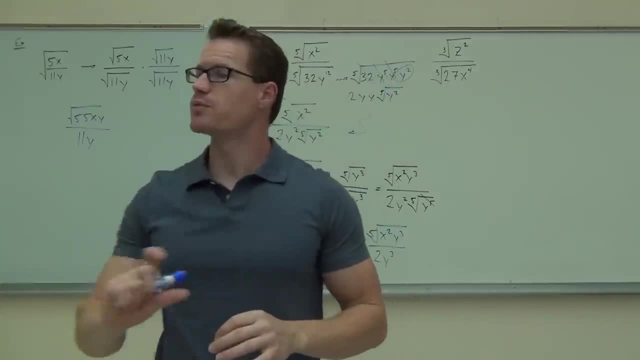 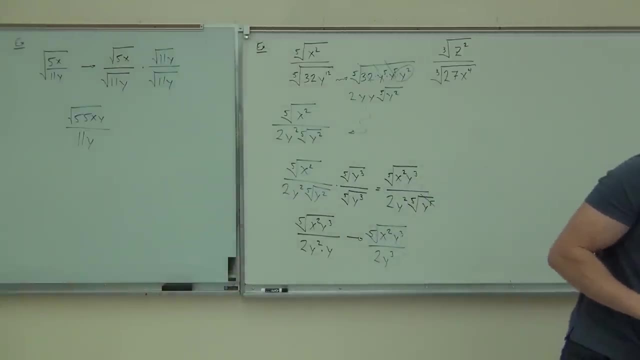 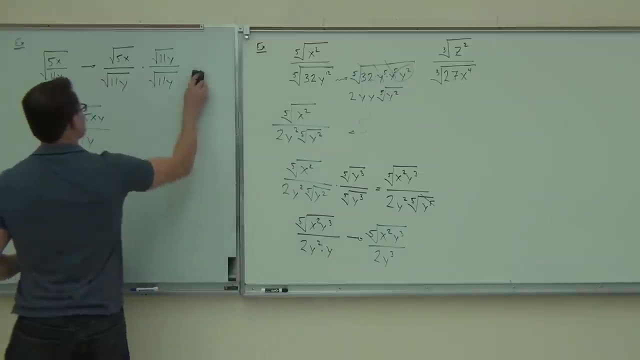 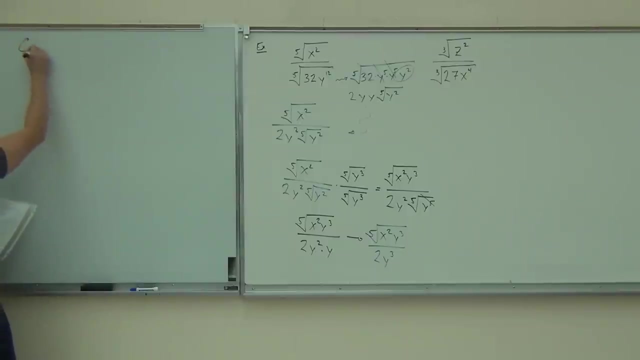 It's very, very similar. Do the same thing that we just did. I want you to simplify the roots first. Simplify them first, Then rationalize what you need to. I'm going to write down the root of x squared, y squared and y cubed. 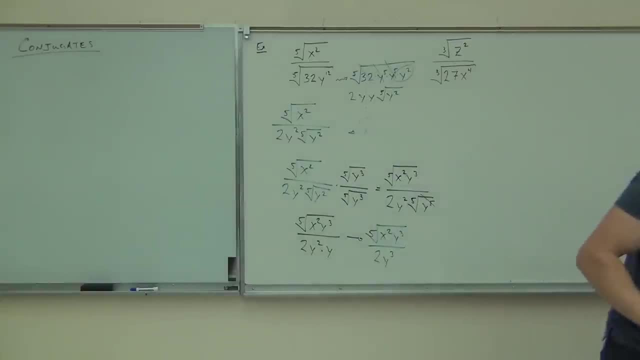 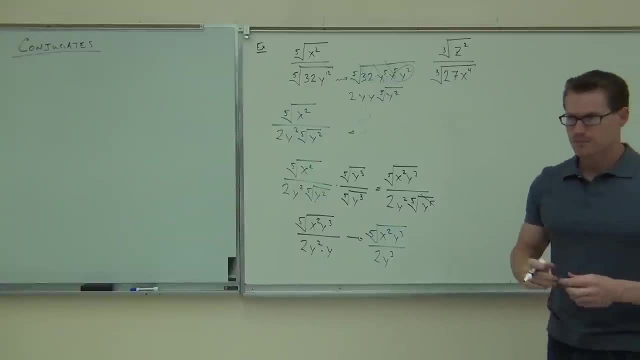 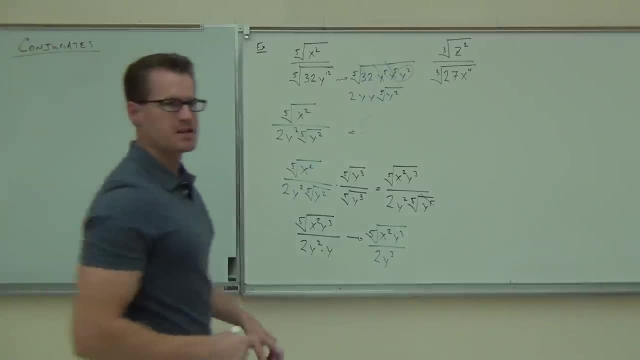 And then I'm going to write down the root of x- squared y- cubed. And then I'm going to write down the root of x- squared y- cubed. Okay, keep working. I'm going to give you the step-by-step. 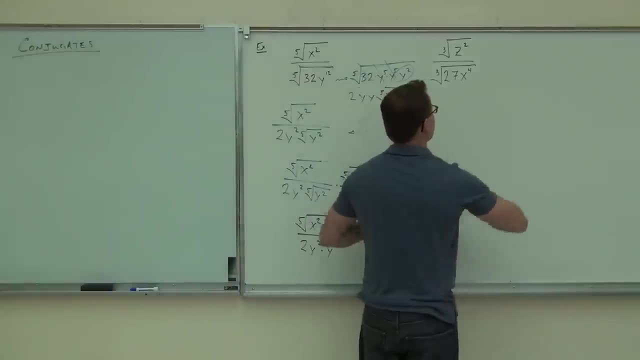 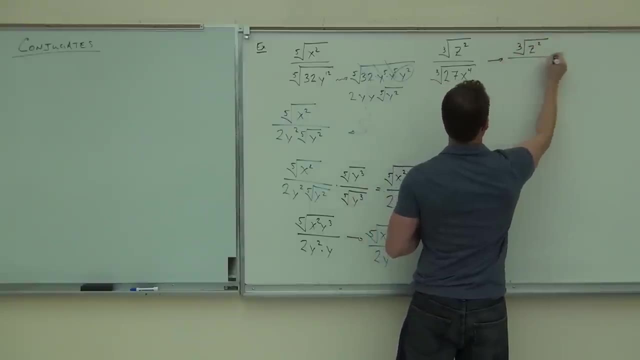 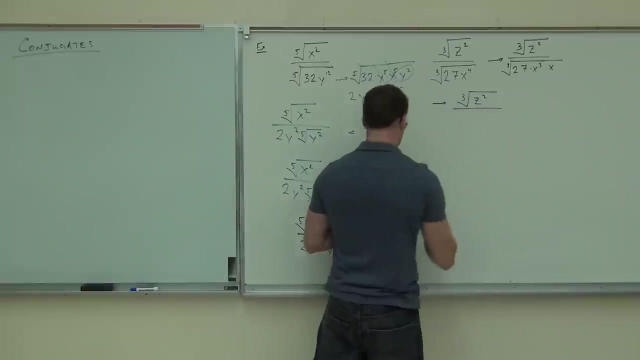 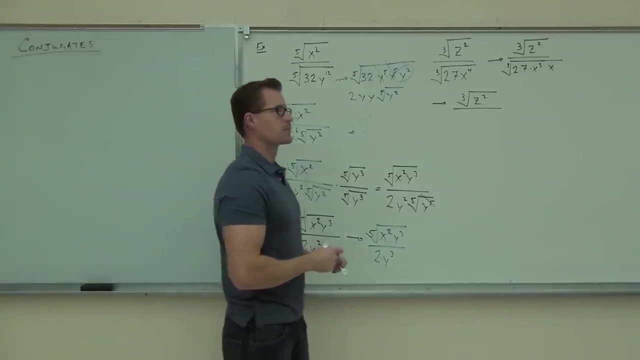 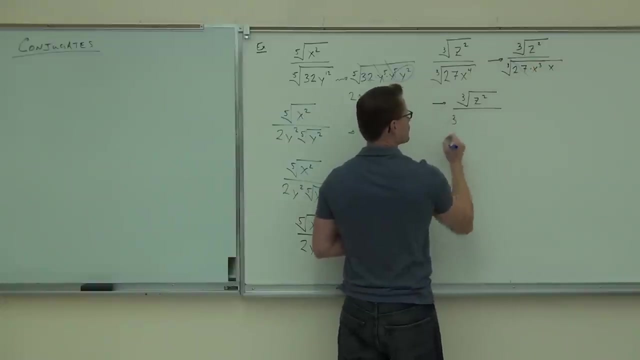 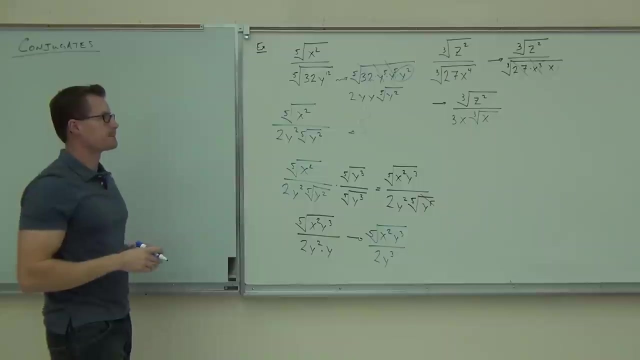 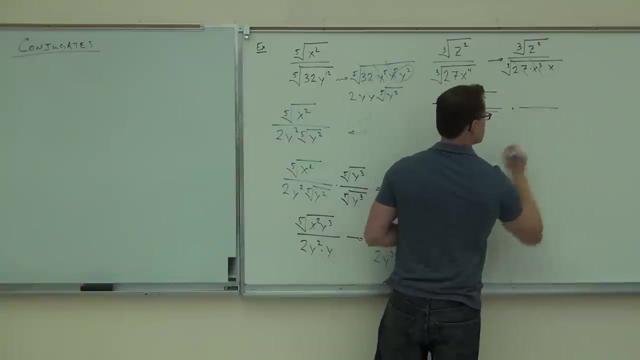 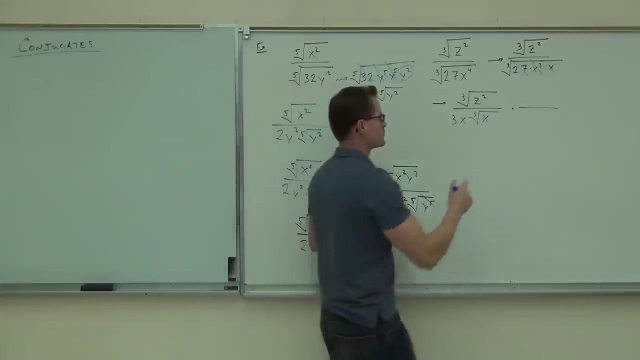 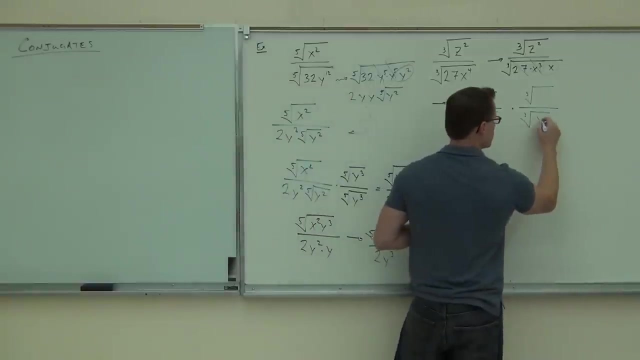 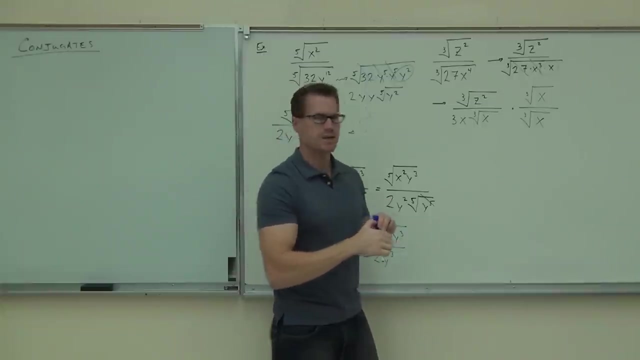 I'm going to give you a new step about every 10 seconds. That way, we can check and see what we're doing. Thank you, Thank you. What's that need to be to work? X squared. This needs to be an X cubed. 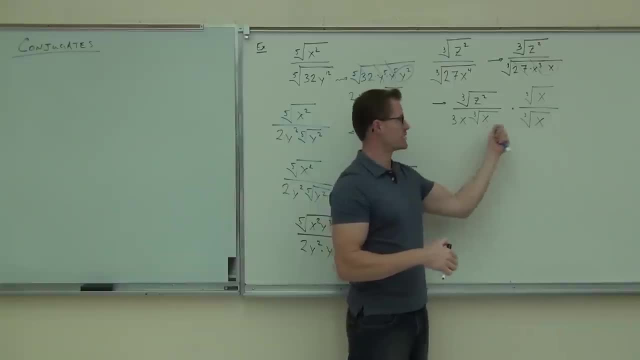 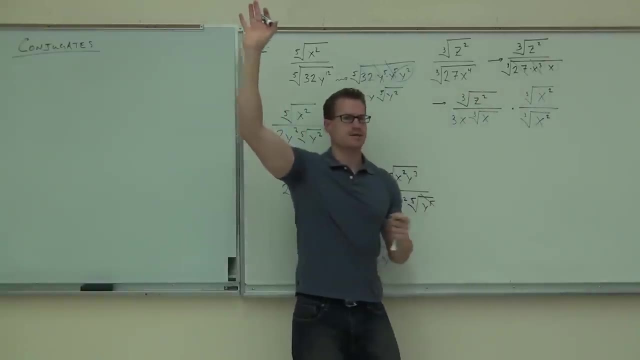 On the X squared, Okay, because we want the X cubed. So we can't just do this. That's not going to simplify What we have to do. is that? How many of you have made it that far? That's fantastic. 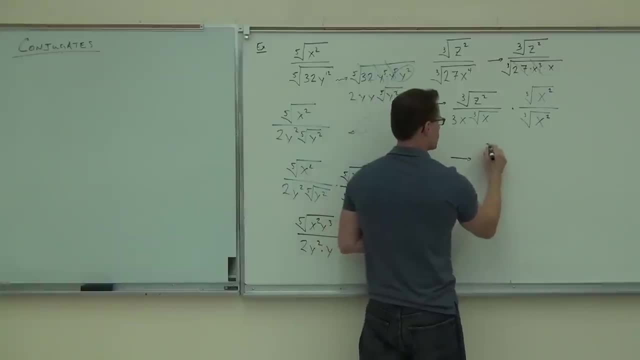 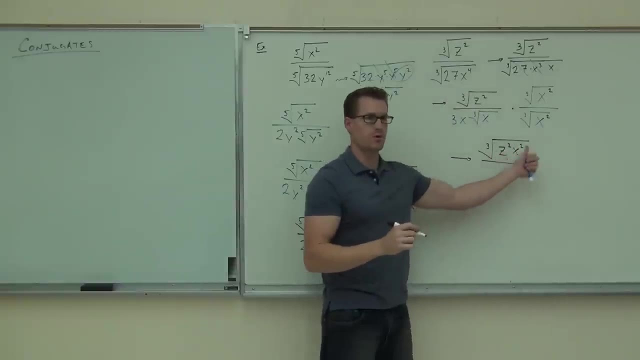 That's very good. By the way, this doesn't have to be in any particular order. If you wrote the X squared first and the Z squared, that's fine. Okay, it's commuted. Q root of X cubed. 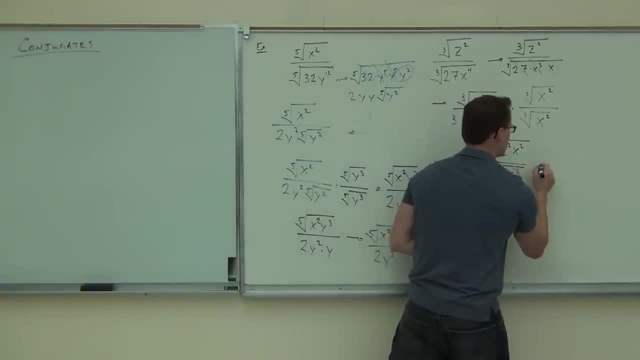 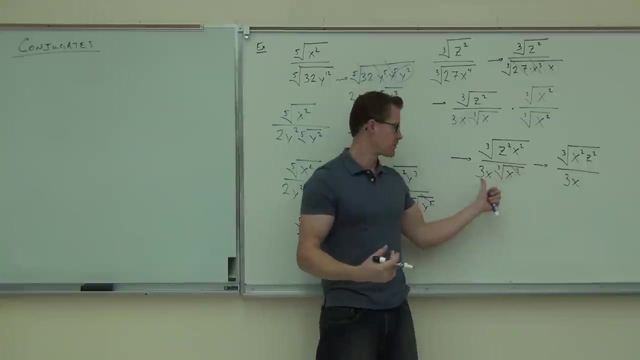 Absolutely. We've got X times X squared. We know that's going to simplify. Be careful, though, This doesn't go away completely. This actually gives you an X. So you have three X's. So you have three X's here. 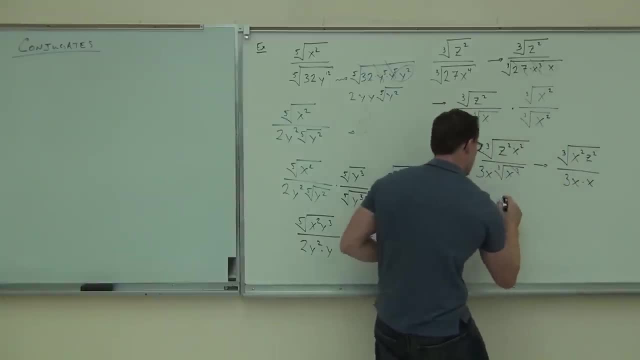 This is: gave you an X, Three X squared. Did you get three X squared? Awesome, All right, Do you feel okay about this? Okay, Now, the last thing we're going to talk about in this section is that word up there. 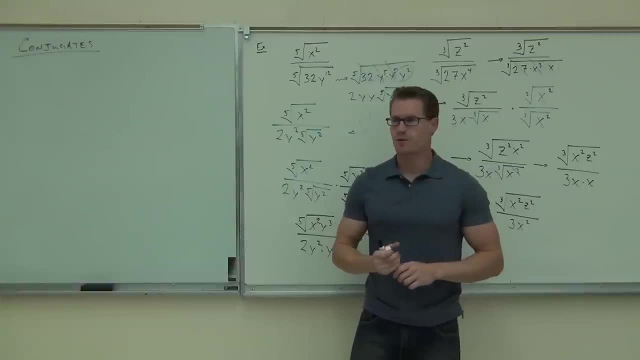 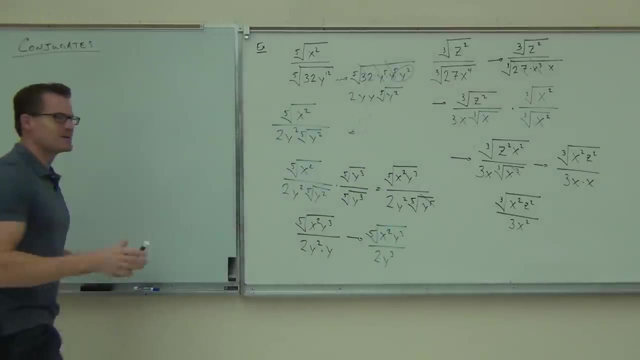 That word says conjugates. Can you say conjugates, Conjugates Or, if you want to be fancy, conjugates, Yeah, Move it. No, I'm just kidding, It's conjugates. Here's what a conjugate means in general. 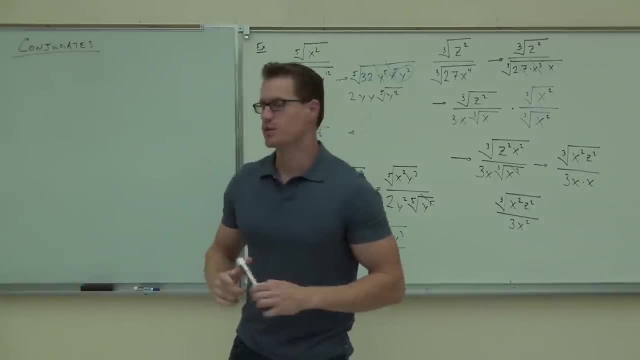 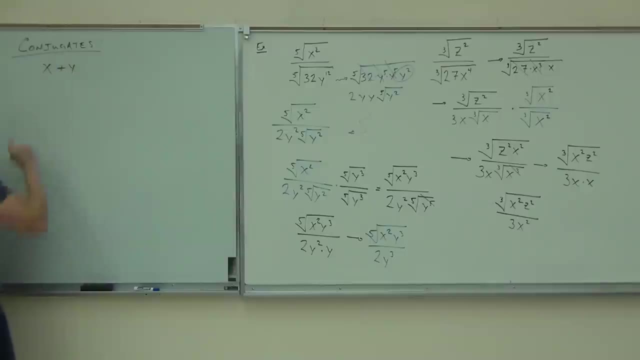 Now we're going to use a specific form of conjugates in our radicals. Here's what a conjugate is. for us, though, If you have X plus Y, a conjugate is a very easy idea. It's a very simple idea. 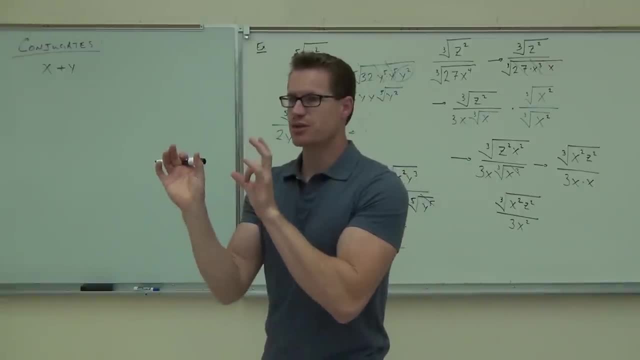 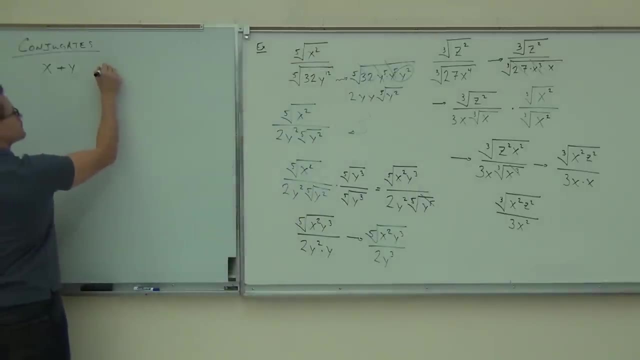 It says that take the same exact expressions but you change the sign in the middle. That's what a conjugate does. So if you have X plus Y, the conjugate would be: what do you think? X minus Y? That's it. 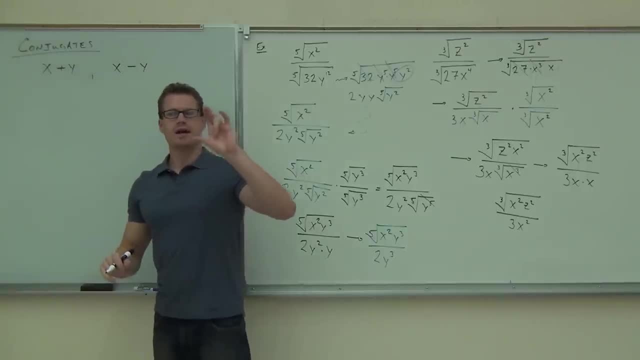 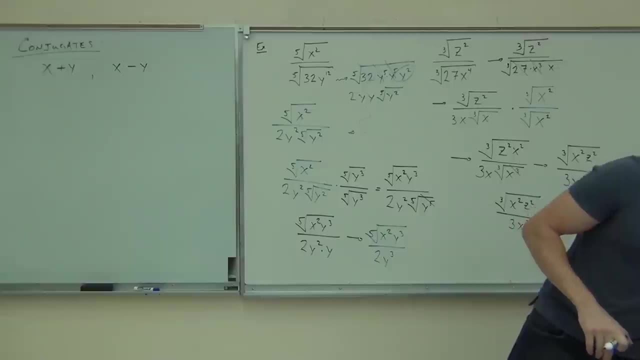 That's a conjugate, And if you had X minus Y, the conjugate would be X plus Y. All it says is: you change the sign in the middle. These two things are conjugates. Now why are we going to be using conjugates? 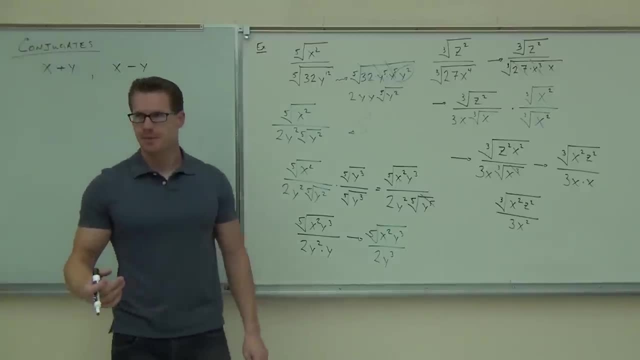 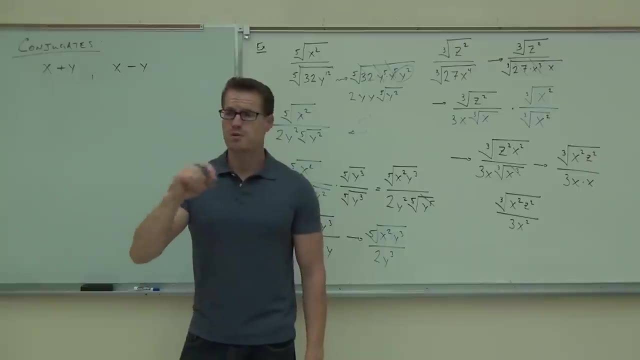 Here's the cool thing about conjugates: When you multiply them together you get something like a difference of squares. Do you remember that Doing that X plus Y times X minus Y? Recognize that if you were to distribute that, if you did X plus Y times X minus Y, 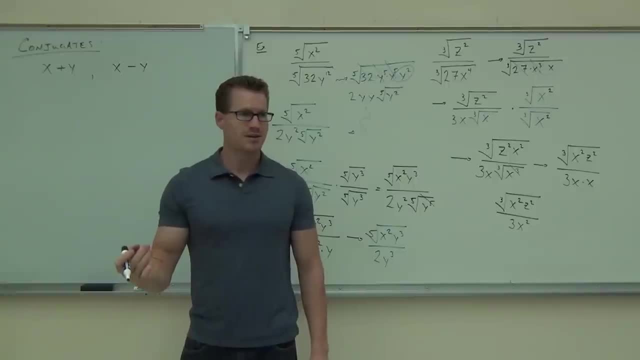 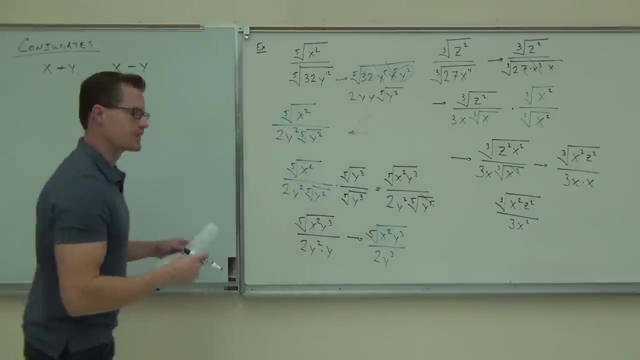 the middle terms would simplify out of your expression. You with me. That's kind of cool, That's actually really neat. That happens every single time. That's why we use conjugates, Because when we're faced with something like this and I ask you to rationalize the denominator- 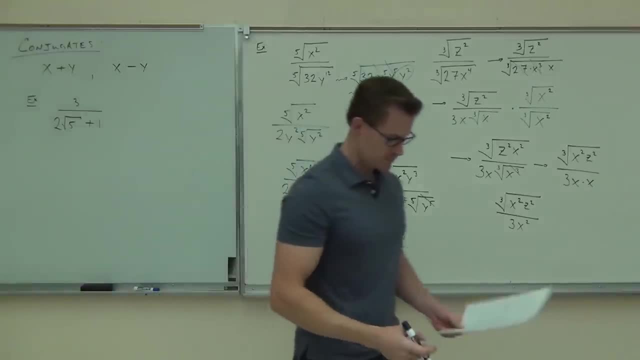 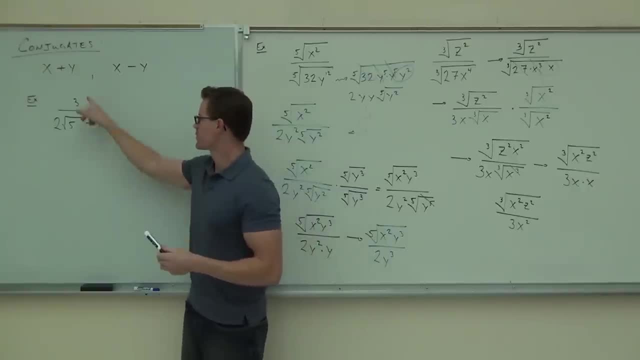 on the numerator right, But I would have to distribute. Do you see that I would have to distribute that if I multiplied by the square root of 5? I have to distribute that Here. it would be great. You would get 2 times 5. 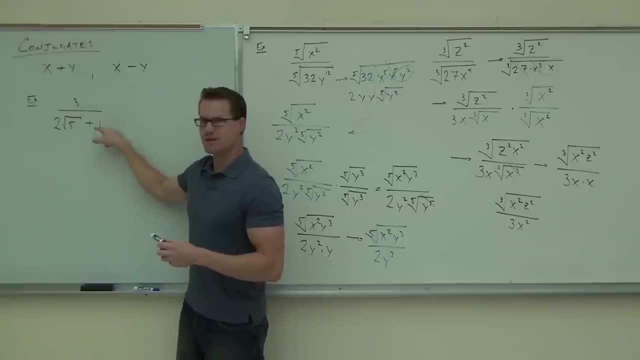 but here you get the square root of 5. And so you'd still have that square root somewhere on the denominator. That's not appropriate if you tried to rationalize it on it. Do you see the problem here? So I can't just multiply by the square root. 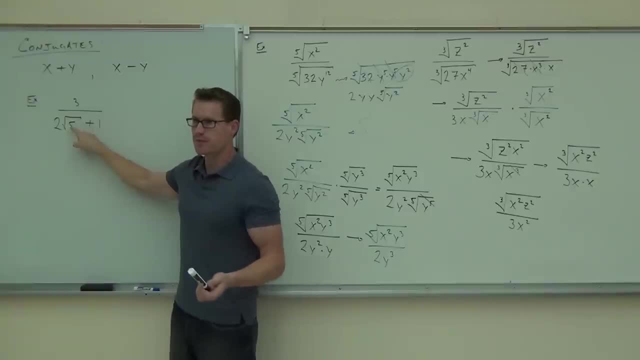 of 5 over the square root of 5.. That's not happening for me. What I want to do is apply the weather prep. have to do is somehow eliminate this root altogether. The idea is I want to use a conjugate. What I know is that the conjugate will eliminate those middle terms that still have the root. 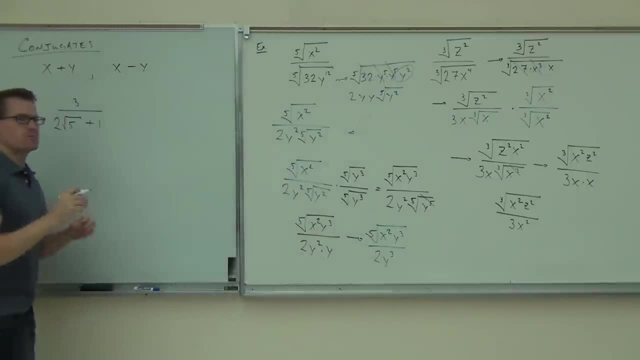 in it. We're going to see this right now. So, to rationalize, you're going to be multiplying by the conjugate And of course this means on the numerator and denominator. You see, we're still multiplying by 1.. We're still multiplying by 1.. 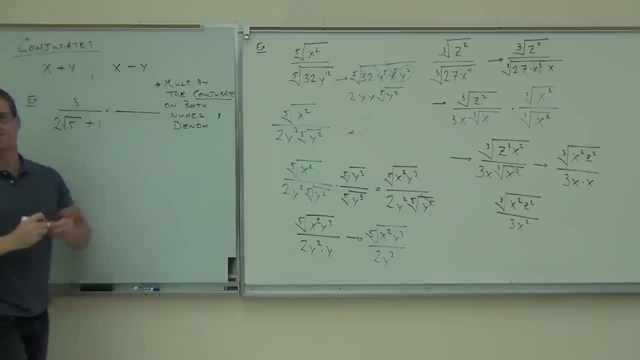 But now it's going to be a more advanced thing for us- Not really advanced, just the thing we need. It looks more advanced, So let's go ahead and see this: If we're trying to rationalize the denominator, which means get rid of all the roots on the bottom of our 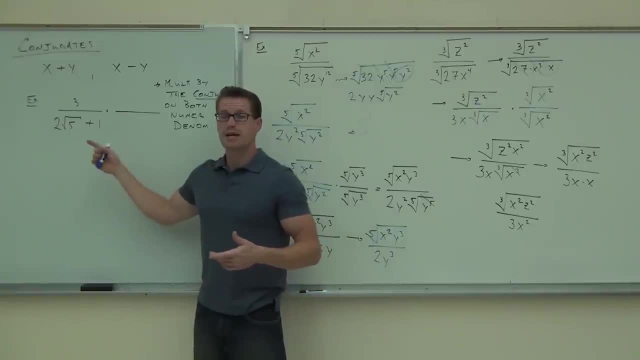 fraction. well, we're going to have to multiply by the conjugate. Can you tell me, if we look up here, what's the conjugate of this expression right here? Root 5 minus 1.. What was that? Root 5 minus 1.. 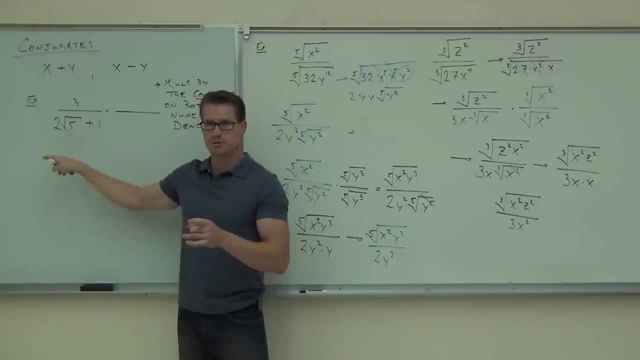 Root 5 minus 1.. Root 5 minus 1.. What about the 2?? Root 5 minus 1.. Still need the 2.. Still need the 2.. The conjugate takes the entire thing, the entire expression. 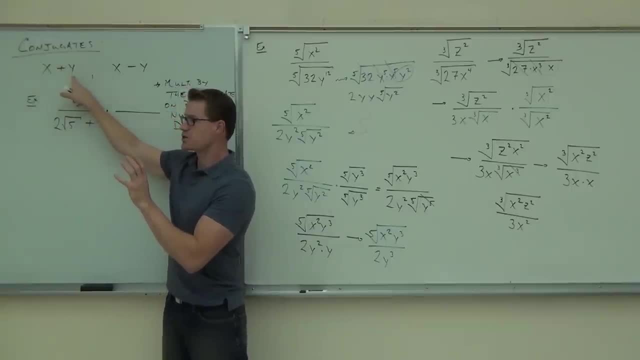 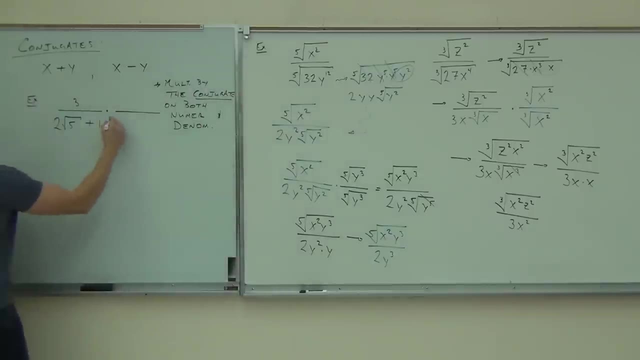 It says the conjugate is: if it's this plus this, we're going to change it to this minus this. So let's all focus again. What is the conjugate of this? How does it start? 2., 2. And then what? 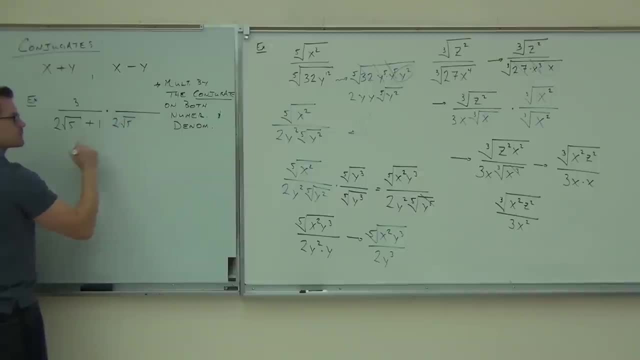 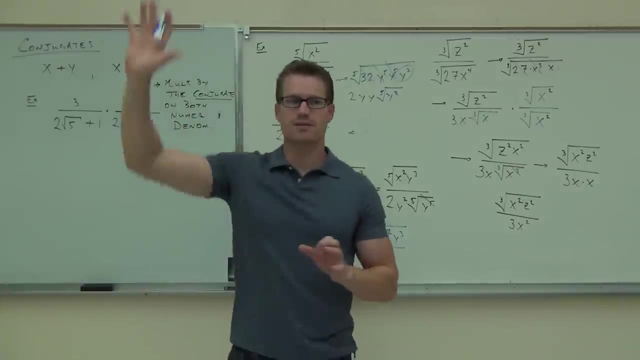 5. 5.. And then what? Minus 1., Minus 1. That's the conjugate. That's exactly right. It looks identical, except for the sign in the middle. Raise your hand if you understand the conjugate. 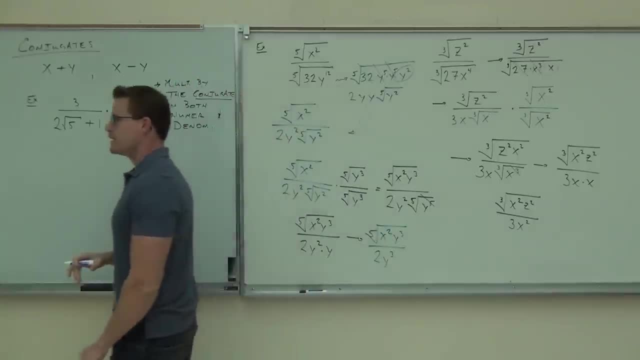 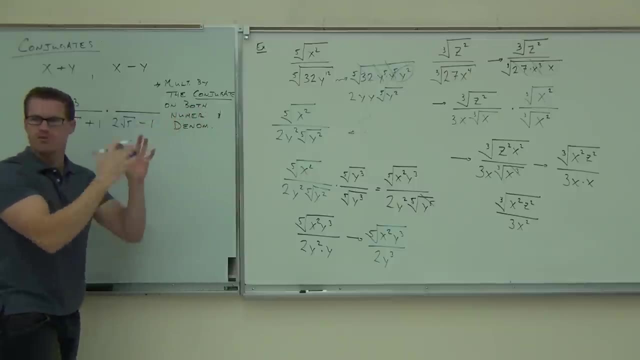 Good, That's fantastic. Now for us, a conjugate has to go on both the numerator and denominator. You see, if we just do this, we've changed the denominator and now the value of my fraction would be different. Now the question: is the top going to be plus or minus? What do 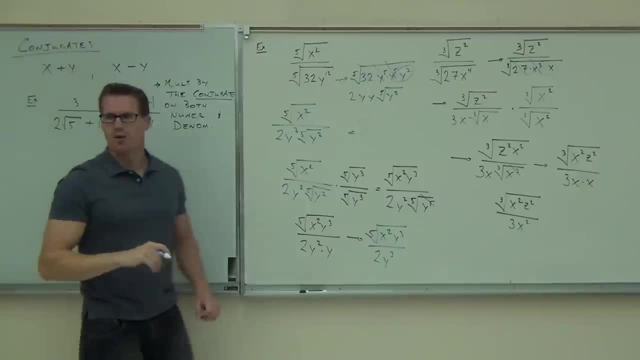 you think Minus, Minus, Of course, Yeah, minus. If it was plus, you know what? That wouldn't make the 1 anymore, would it? I'd have something different That wouldn't make 1.. That would be a different. 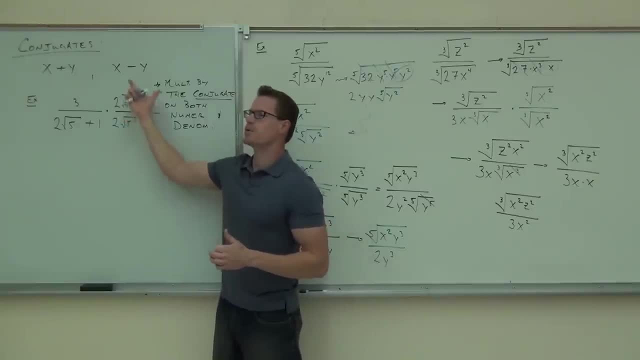 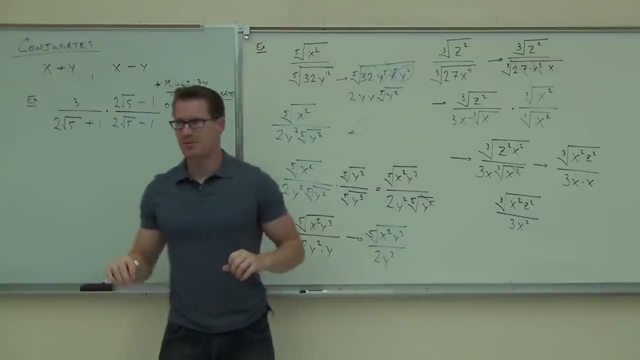 expression. So whatever you have here, whatever your conjugate is, you have a conjugate. You're going to have it in both spots. This is actually being multiplied by 1.. That's why we're not changing the value, We're just changing the way it looks. Are you OK with this? so far? 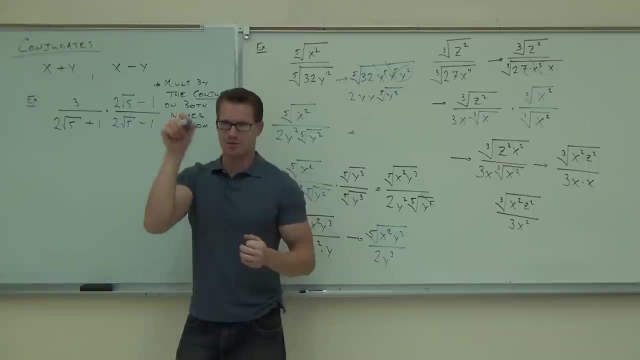 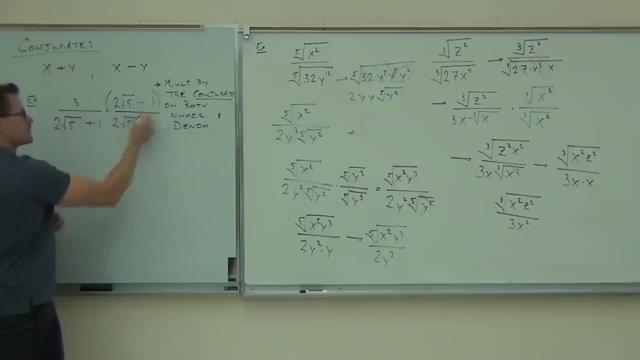 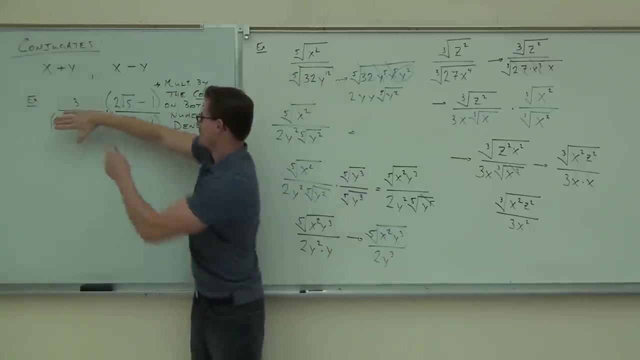 Yeah, Now remember all that stuff we did with distribution. We foiled out all those radicals. You know why we did that. Oh boy, Oh boy. Does it look familiar If you ignore the bottom. can you do that? 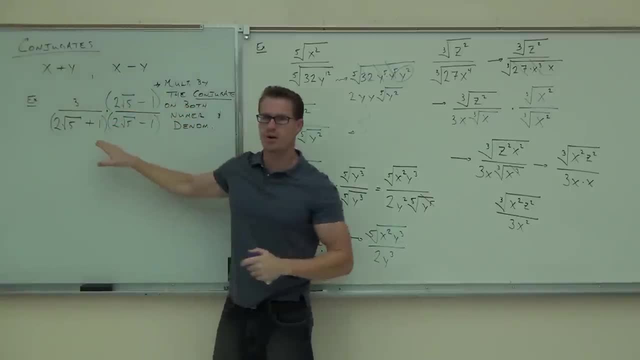 No, If you ignore the top, can you do that? Mm-hmm. That's why I had to do all that stuff. Listen, it gets kind of nasty on those problems on your homework that you've been doing right. You have a lot of things going on. Be careful. 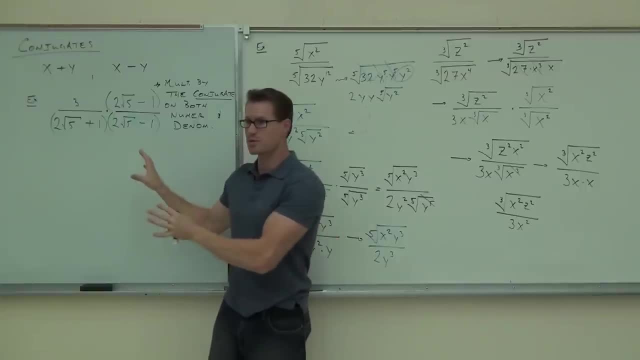 on this stuff. You've got to be rock solid on the distribution in order to get these problems correct, So be careful, Don't go too fast. Write out all the steps. Are you ready to do this? Yeah, Firstly, are you OK making it this far? 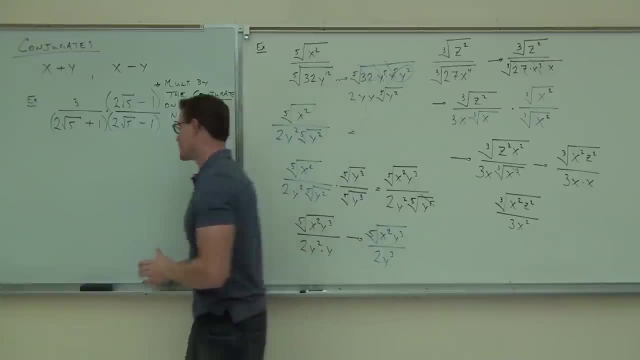 Yeah, We're going to see exactly what happens when we distribute. now, what happens with those roots? Let's deal with the top first. That's the easy part. Deal with the numerator first. If I deal with the numerator, let's be very careful on this. We do 3 times 2. 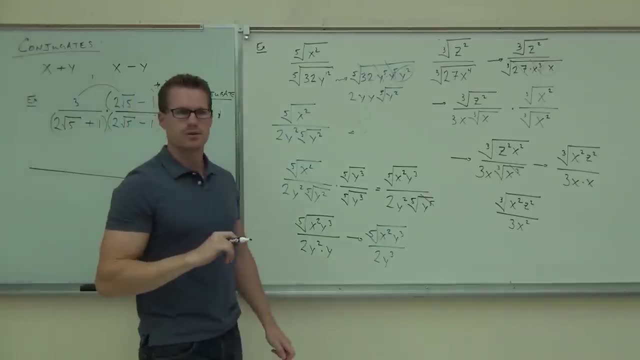 root 5.. How much is 3 times 2 root 5? 6 root 5. Not 6 root 30? No, Or 6 root 15, you mean 30. I don't know how you do that. 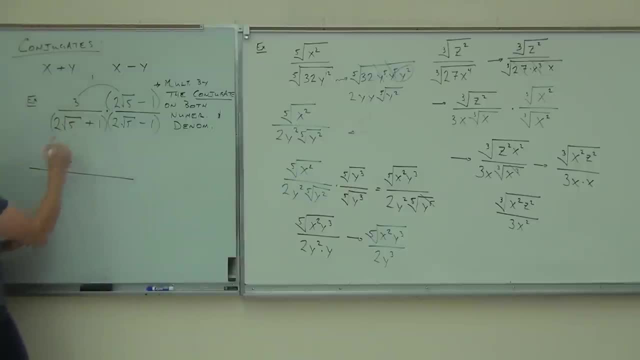 No, it's not that one. No, it's definitely not that. Sure, we get the 6 root, 5. And then minus how much, ladies and gentlemen, 3.. Good Numerator is nice in this problem, You're done. 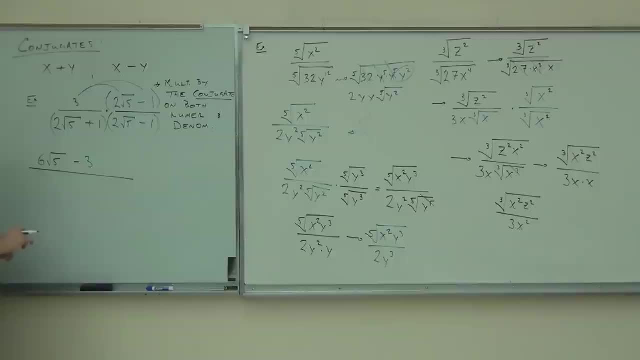 That's it. Denominator takes a little bit more work. Denominator, you are still going to FOIL. We're going to write out everything when we FOIL this. This is the trickier part. So when we FOIL, of course we get 2 root 5 times 2 root, 5.. Are you with me? so far? You? 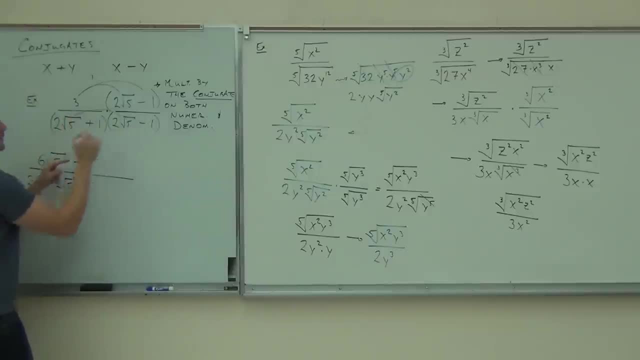 see where those things come from. I hope We're going to get- do you see it plus or minus here? Minus, Minus 2 root 5 times 1.. Minus 2 root 5 times 1.. Then we're going to get plus 1 times 2 root 5.. That's an awkward. 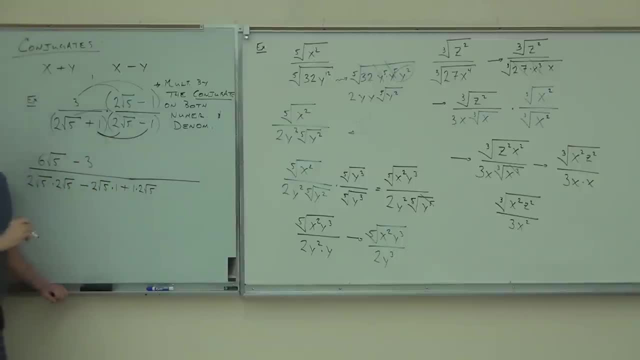 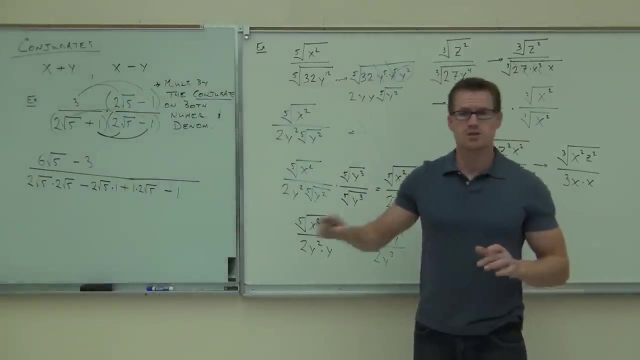 line, isn't it? And then, lastly, we'll get how much Minus 1. Minus 1.. I need to take a closer look at that. You've got 5 seconds to look that over. Can you do that on your own? 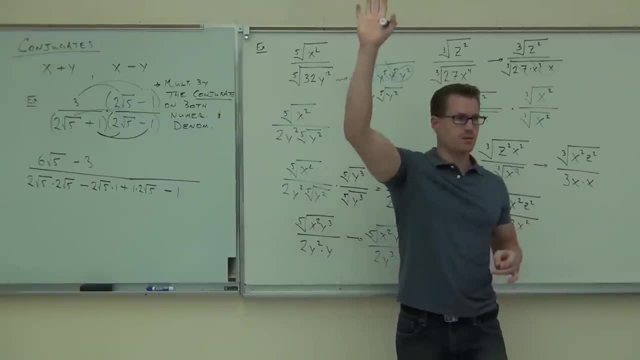 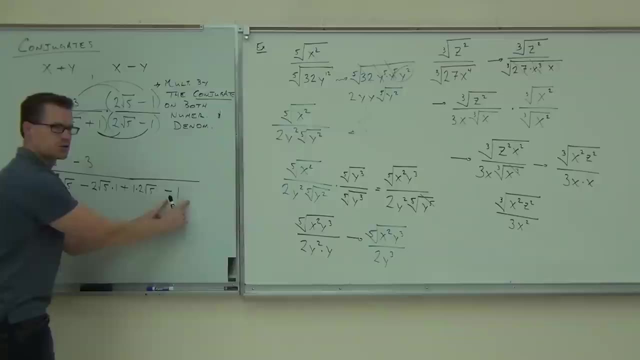 Yes, Raise your hand if you can. Good, It's just our distribution. We really haven't done much math, We've just distributed. We should have 1,, 2,, 3, 4 terms, because we're multiplying 2 terms times 2 terms We have. 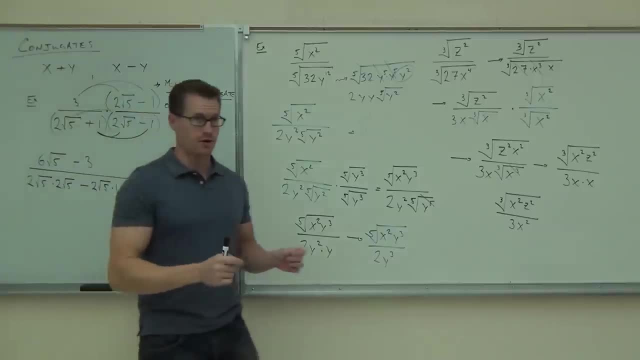 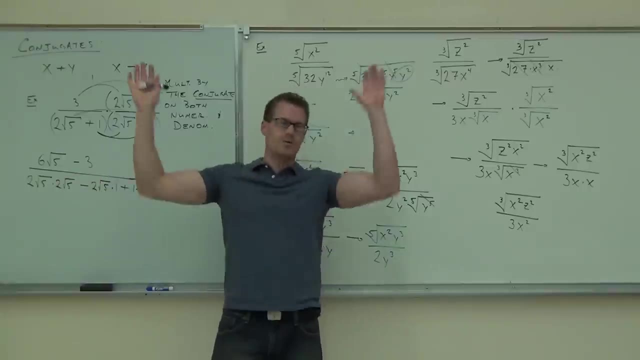 that Now is the part where we get to simplify this. Are you ready for it? I'm going slowly. I'm making sure you understand this, because it's kind of an important concept and people lose it right here, Not like wow, but like they lose their track. 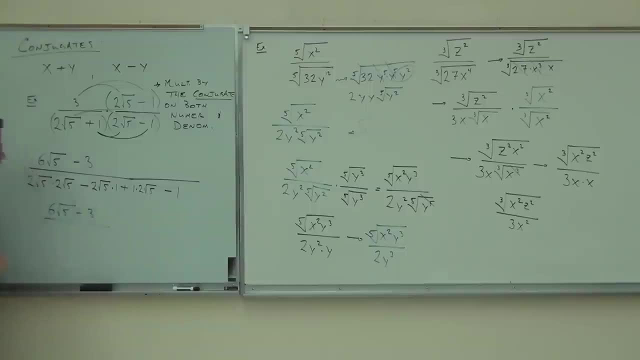 So 6 root 5 minus 3, sure, This one especially is where people get lost a little bit. You've got 2 root 5 times 2 root 5.. What can you multiply together and get out of this? Firstly, 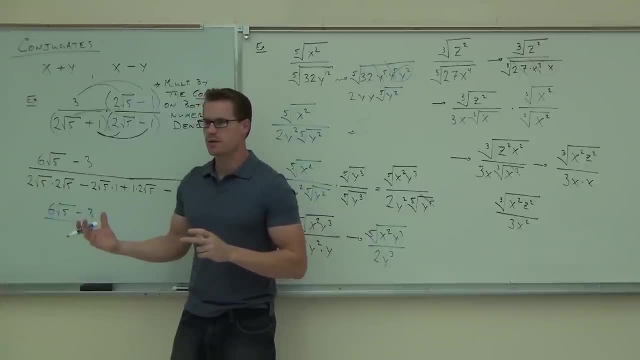 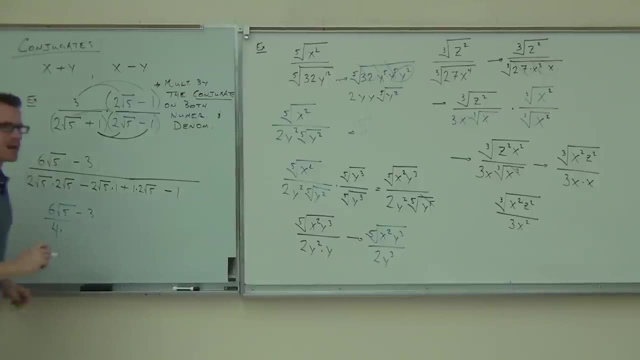 what about the 2 and the 2?? Can you multiply those things? You're good, Yeah, you're going to get how much? 4. Definitely 4.. Now here's the deal. There's got to be a difference in your head between. 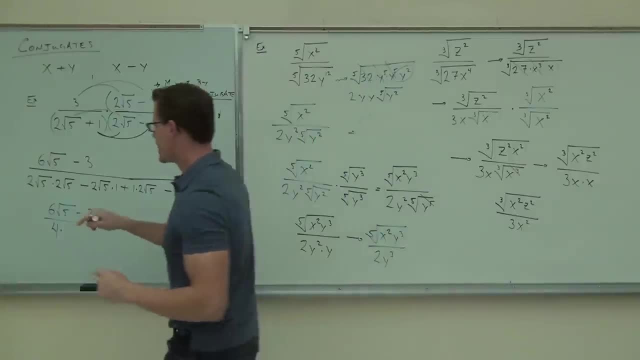 adding roots and multiplying roots. You see, if we were to add this, watch carefully on the board, please. Everybody's eyes should be on the board right now. If I were to add this, this would be 4 root 5.. 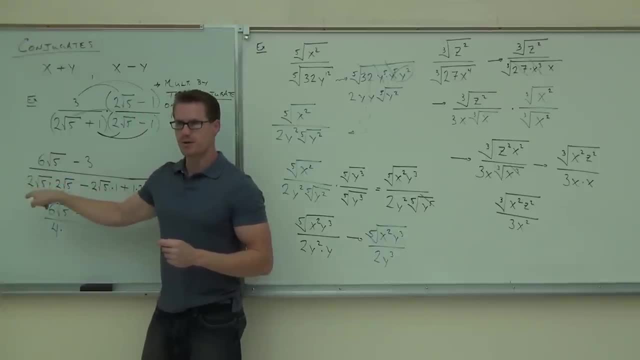 Yeah, Yeah, 4 root 5.. Are you with me? That would be 4 root 5.. Do you agree? Yes, If I'm multiplying it, are you still going to give me 4 root 5?? No, 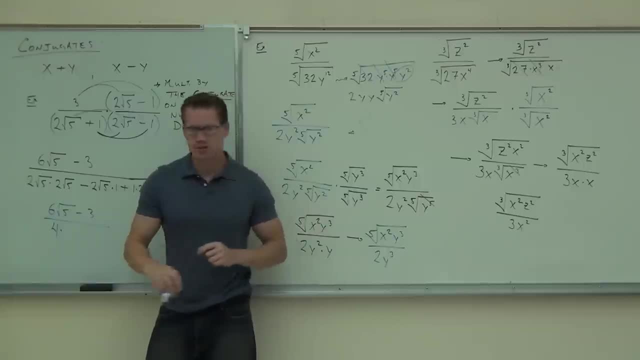 No, because multiplication is different than addition. Multiplication says: sure, I multiply these 2's and I get 4.. I multiply the root 5's. How much is root 5 times root 5? 5. It's not root 5 anymore, is it? That would be added. I'm multiplying here, it gives. 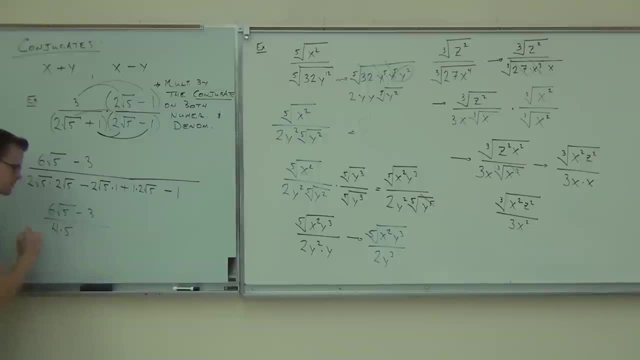 me, 5.. No more root, 5.. You see the difference, Yeah, Okay, so multiplication and addition have to be different in your heads. Now here's the cool part. Okay, check this out: How much is minus 2 root 5 times 1?? 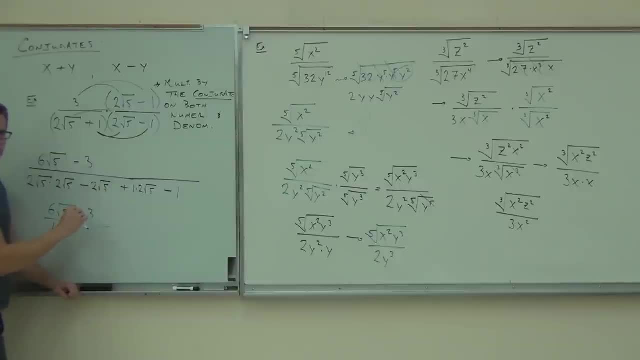 Minus 2 root 5.. So that's pretty much gone, right, And 1 times something is pretty much gone, because when you multiply by 1, you get that same expression. What's minus 2 root 5 plus 2 root. 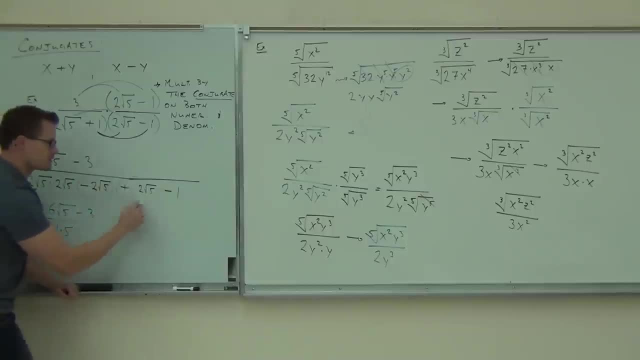 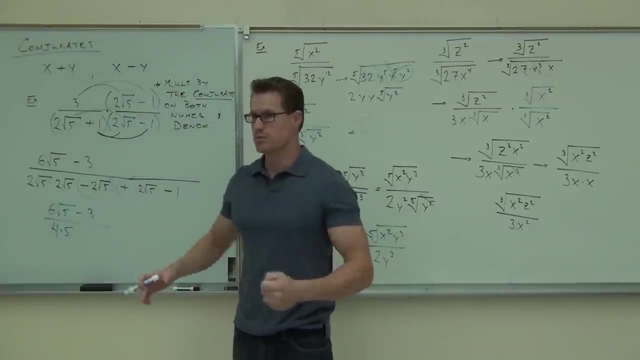 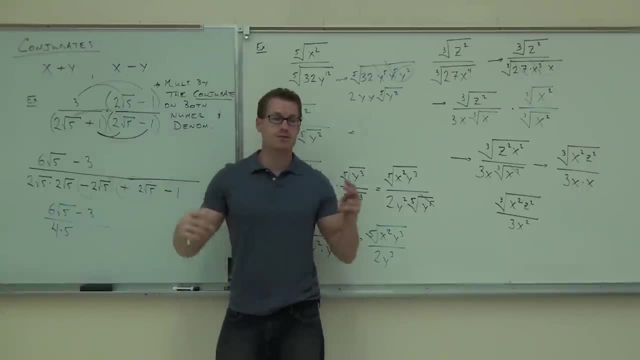 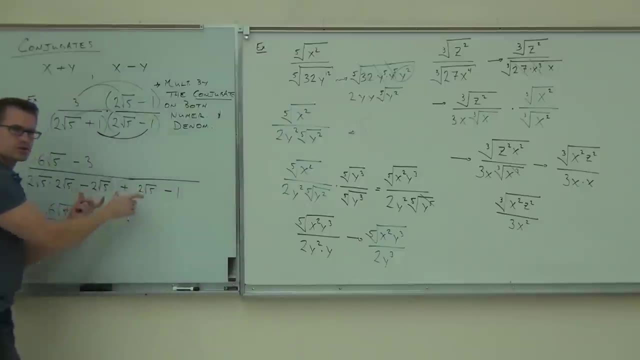 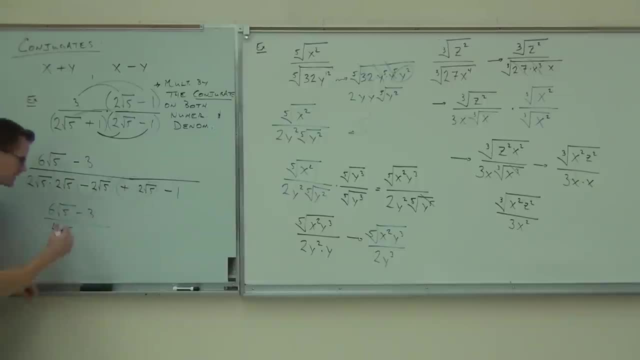 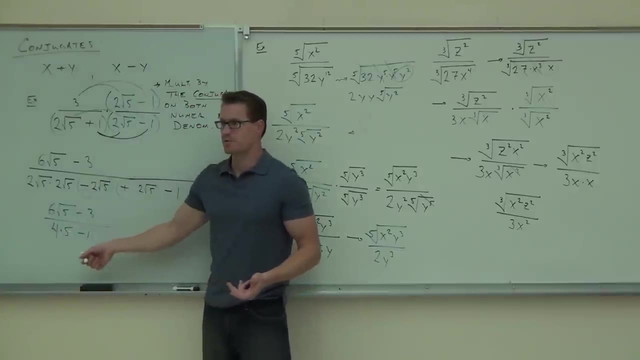 That's great. that's why this whole thing works. Lastly, we still have a minus one, but notice how there is no root. All you gotta do now is multiply and add some numbers and you'll be done on this problem. How many of you feel okay with this so far? 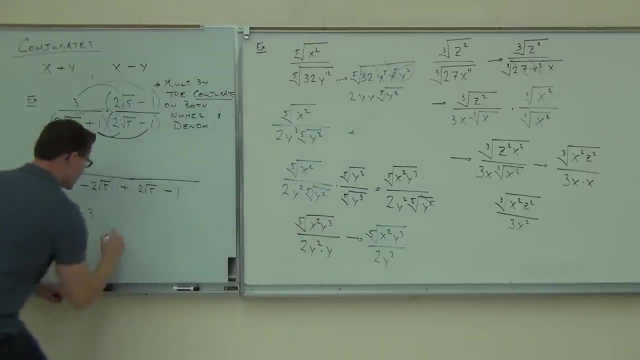 That's why the conjugate works the way it does. it simplifies out the middle terms. So we'll do one more step. Six root five minus three over. that gives you Twenty-five Minus one, Nineteen, You're done. 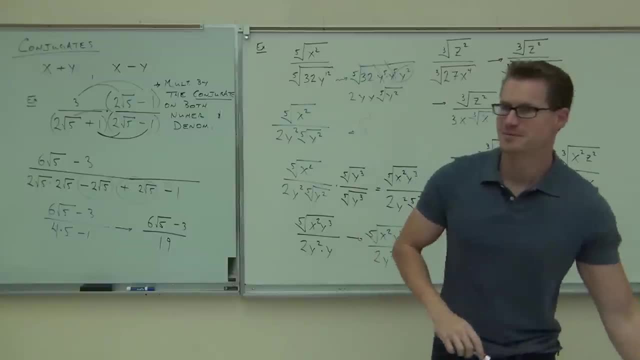 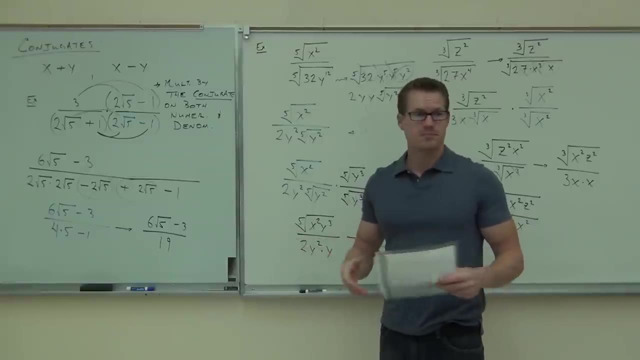 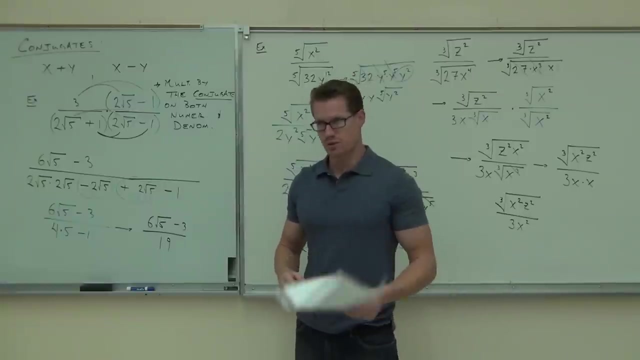 No more root full number. Kind of cool, Is it that? Are they always gonna be square roots or is it a cube root? That's a good question. The answer is yes. These problems will all be square roots. You see, the problem is, if you have a cube root, 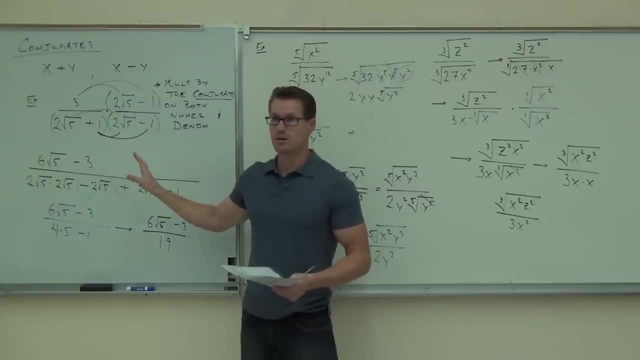 this does not work at all. If you have any other type of root. that doesn't work at all, Because you can't multiply a cube root times itself and get the radicand Here. the only reason why this works is because you can do that with a square root. 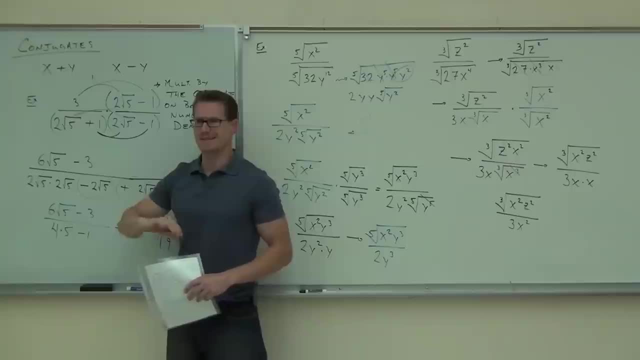 You can say, oh, this is always gonna give you five, That's a cube root, that doesn't happen anymore and you're stuck, you can't do it, Are you with me? So yeah, these are all gonna be square roots. 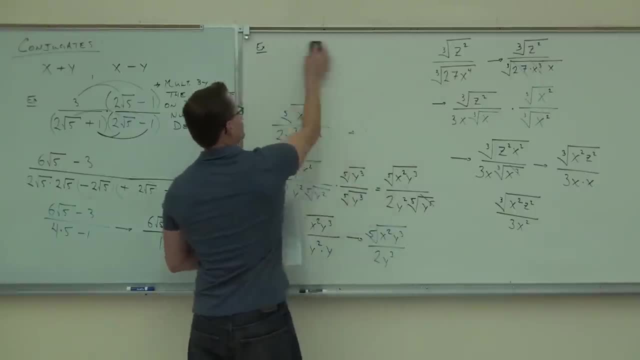 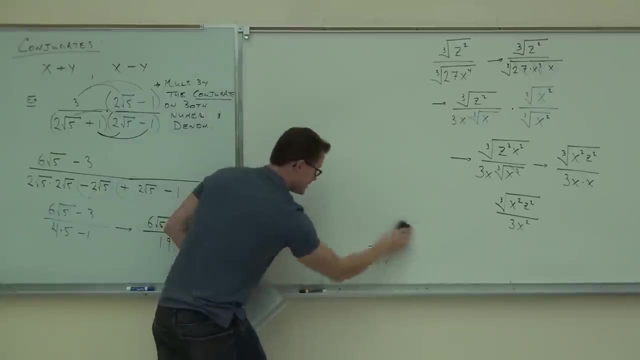 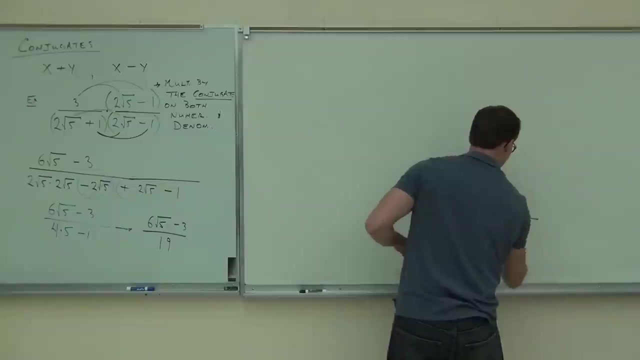 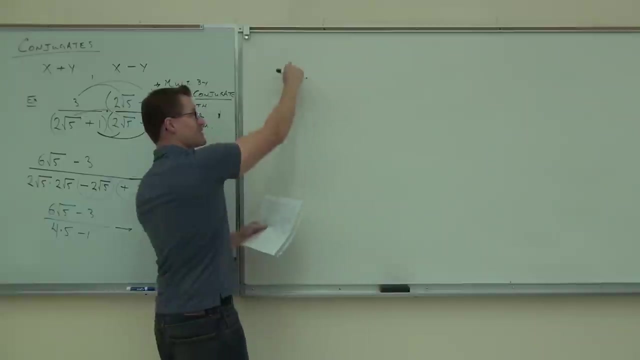 It's kinda nice. actually, None of this type looking stuff and this type of problem. You should be thanking me right now. You're welcome. You are gonna have a problem just like this one. well, not the blank part. 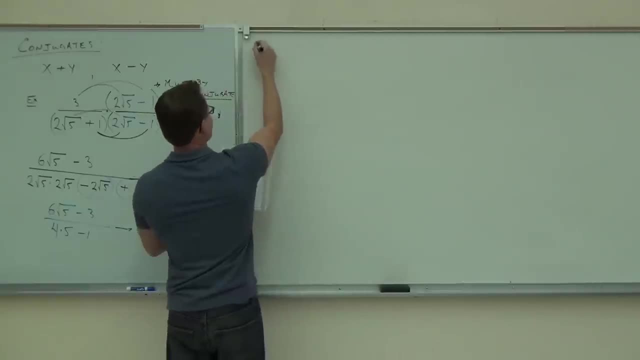 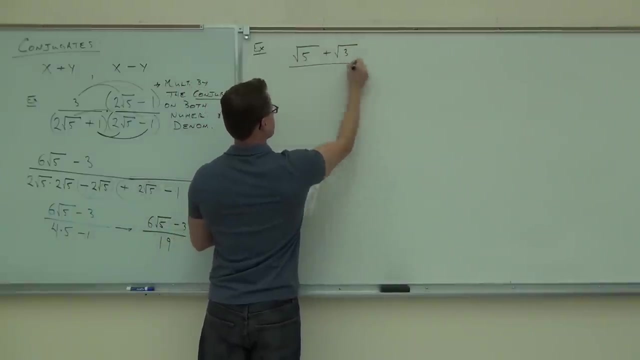 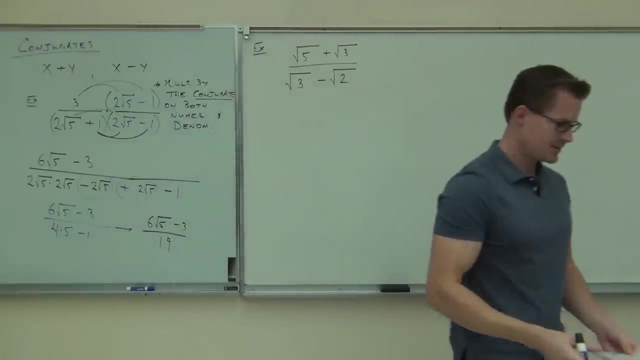 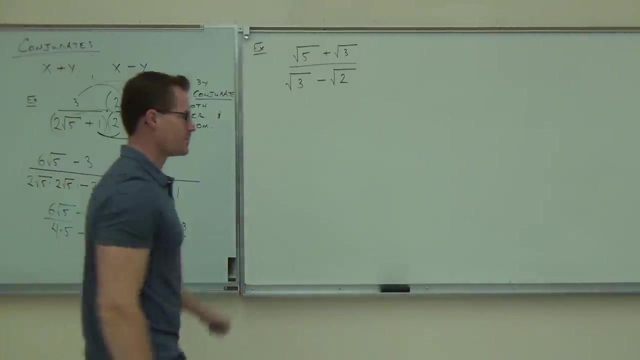 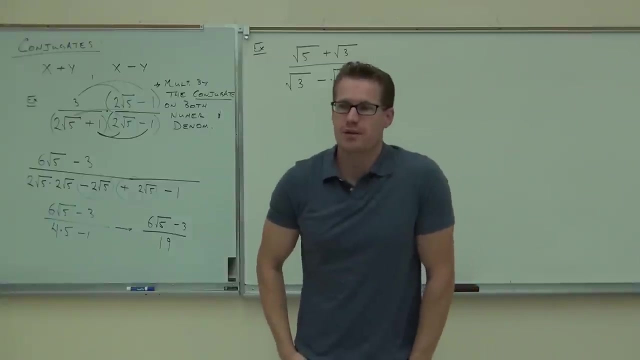 but the thing I'm gonna write in on your test. Let me think, if I think up what that means. Ooh, Phew, Now that's a problem. That's a problem. Now you gotta read it carefully. You gotta know whether I'm asking you. 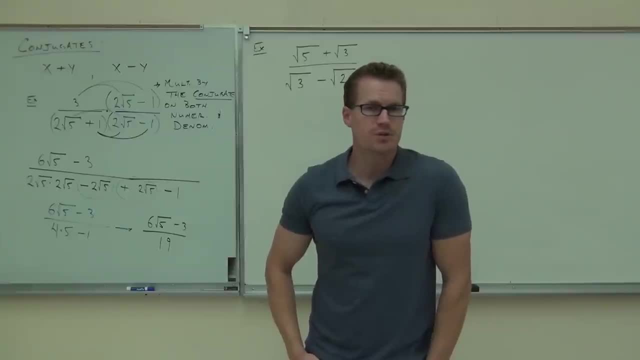 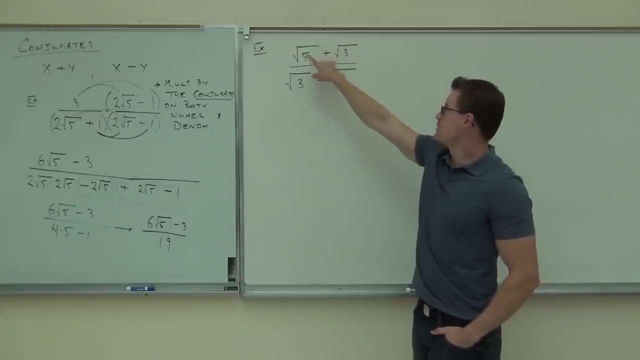 to rationalize the numerator. If I were asking you to rationalize the numerator, that would mean trying to get rid of these roots. True, You'd be multiplying by the square root of 5 minus the square root of 3 over the square root of 5 minus the square root of 3. to rationalize the numerator: 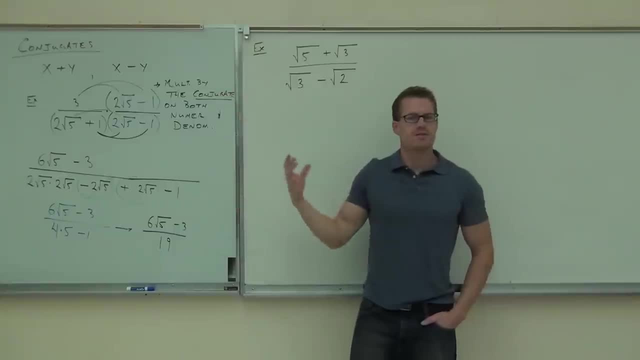 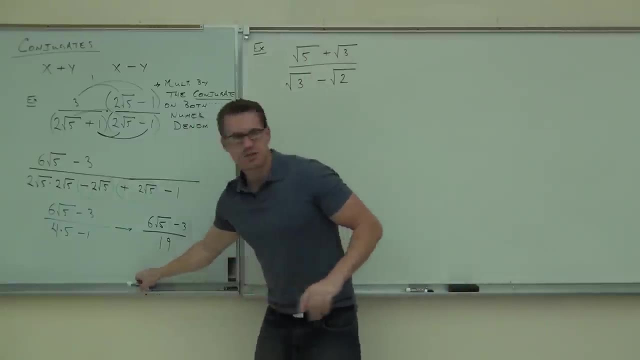 If I'm asking you, like I am, this has all been denominators. If I'm asking you to rationalize the denominator, which is what this question is, I can't multiply by these two things. Can you tell me what I do- so I'm on the left-hand side of the room over here- what I do need to multiply by. 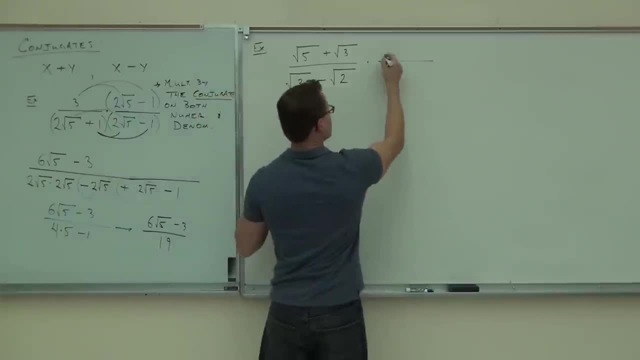 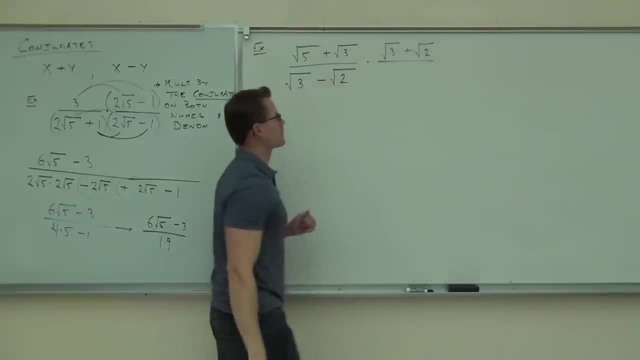 Don't all talk at once. Square root of 3 plus the square root of 2.. Square root of 3.. And you said: what now? Plus the square root of 2.. Yeah, That's going to rationalize the denominator. 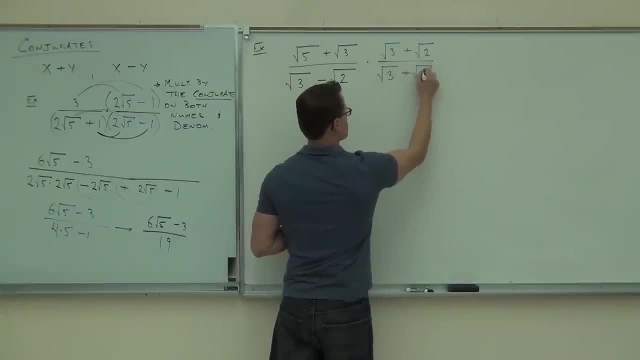 Square root of 3 plus the square root of 2.. Where am I getting those things? Is that magic? I wish Kind of cool if I had magic. I try to use the force all the time, like Luke Skywalker. That never works either. 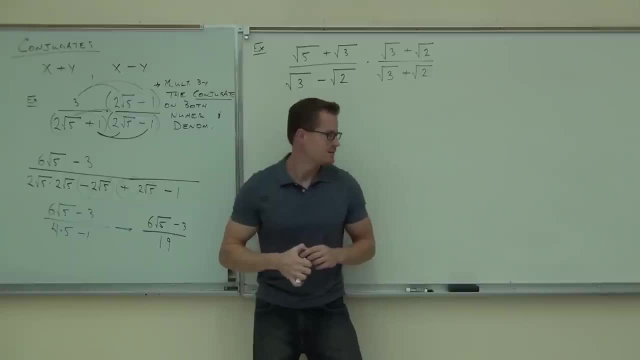 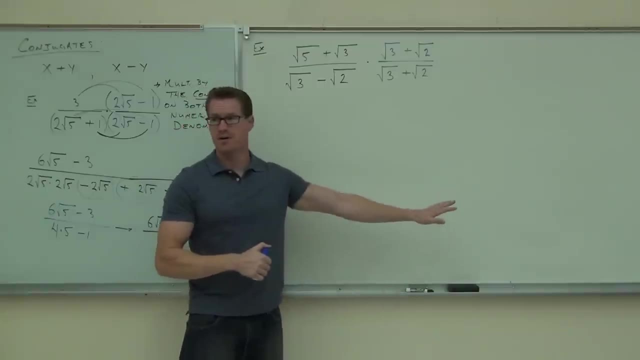 No, I tried it in my last class. Get the razor- Ah, It never works, Never, Not once. One time I made it move, I think, But I could have just been getting dizzy Anyhow. so we're looking at this expression, trying to rationalize this thing. 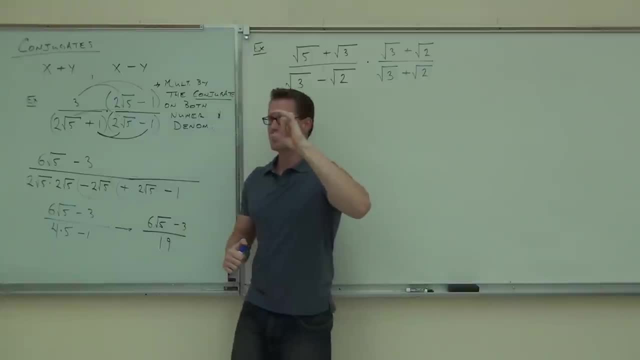 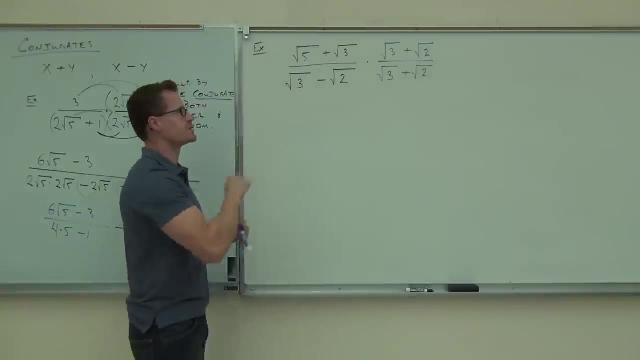 We get exactly the same roots. The only difference is the sign in the middle is opposite. That's it. All right, let's get in the conjugate here. So multiply by the conjugate of whatever you're trying to rationalize. here is the denominator. 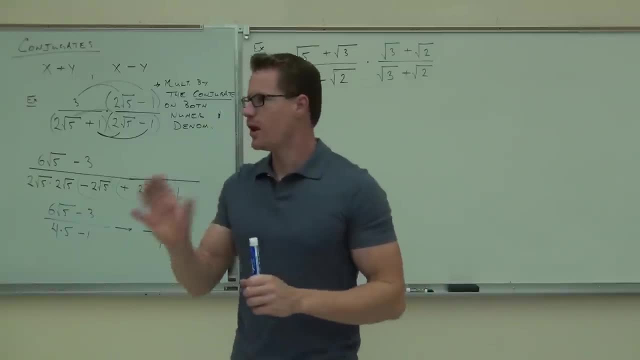 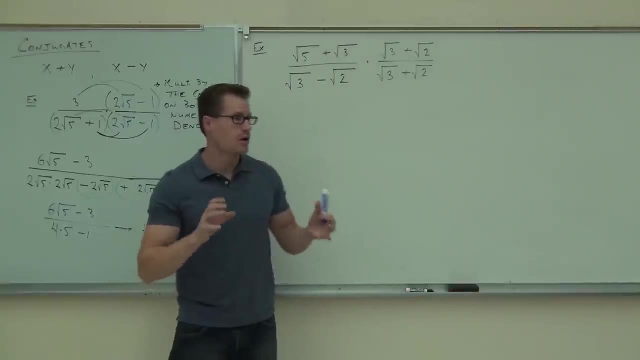 Now the next part. this is the hard part for people because you have a lot of roots going on A lot of stuff. If you're not good at it, you're going to make some mistakes. If we're doing this in our head, chances are a lot higher that we're going to be making those mistakes. 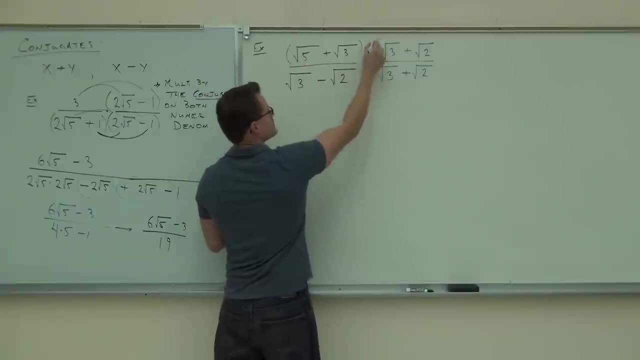 So we do understand that we're multiplying right, Which means we've got some parentheses everywhere And we are going to have a whole lot of distribution going on. Okay, Let's go nice and slow. Let's see exactly what we get. 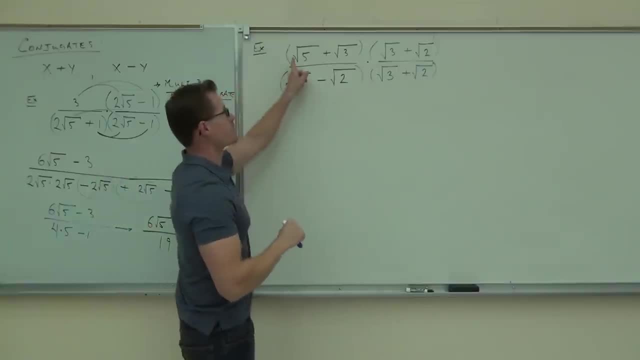 Let's go right side of the room. Tell me the first couple things I'm going to get with my numerator. I'm going to have a really long expression here. What's the first thing I'm going to get, please? Square root of what? 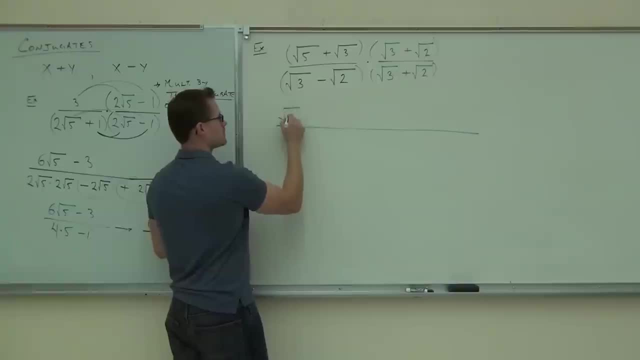 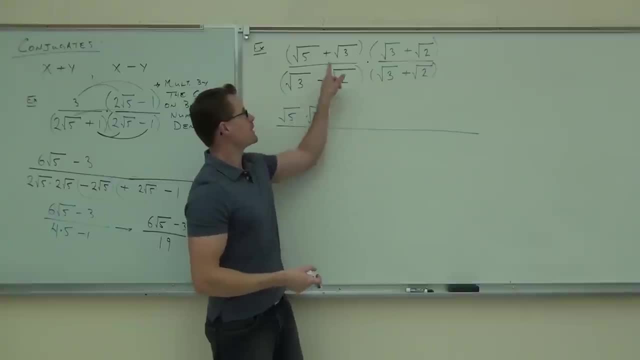 Because the thing about it is, if I give you this and I give you like three instead of the square root of three, you're going to have something a lot different. I want you to write it out: Go slowly, Don't do this stuff in your head. 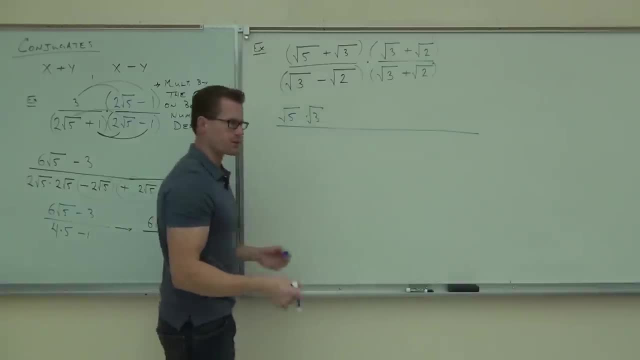 Write out every little part of it and then do the math. We're still learning this stuff. Okay, Let's keep going. Right side of the room, I'm going to have you do the entire numerator, And left side, I'll have you do the denominator. 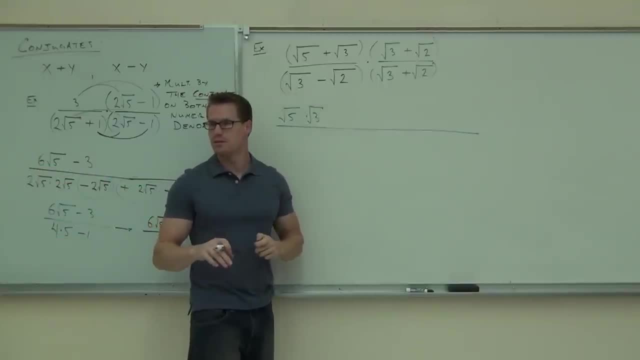 So, right side, keep going. What's the next thing that I need, please? Square root of five, Square root of five plus Oh, plus, Okay, That's important. And then what? Square root of five times square root of two? 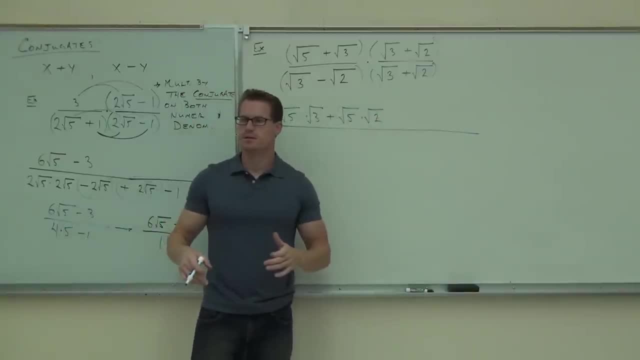 Okay, Cool, Let's keep going. What's the next thing? I need Plus, Plus, Plus, All right. Square root of three times square root of three. Okay, And somebody else. let's finish this off. What's the last thing? 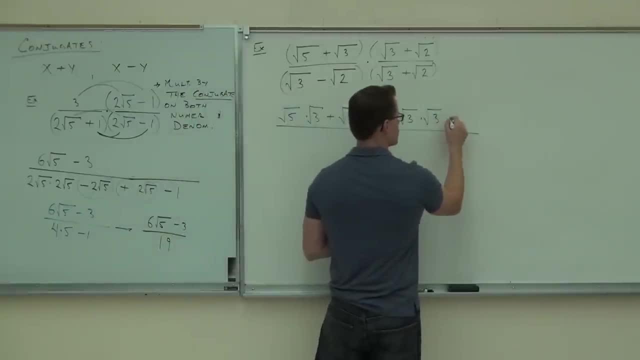 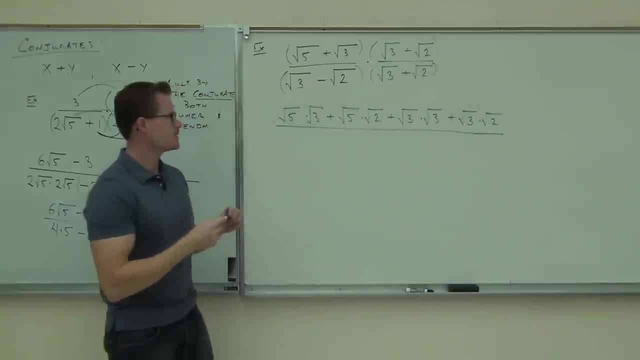 Square root of three times square root of two. Perfect, You say plus Yes, Square root of three times square root of two. Okay, All right, Let's show our hands how many people feel can't get that far. Good, That's our basic distribution. 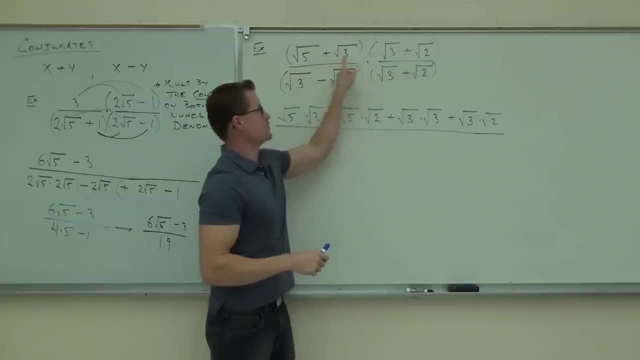 We have root five, root three. We have root five, root two, Root three, root three, Root three, root two. We have those expressions right here. We've just foiled that out. We should have four terms: One, two, three, four terms. 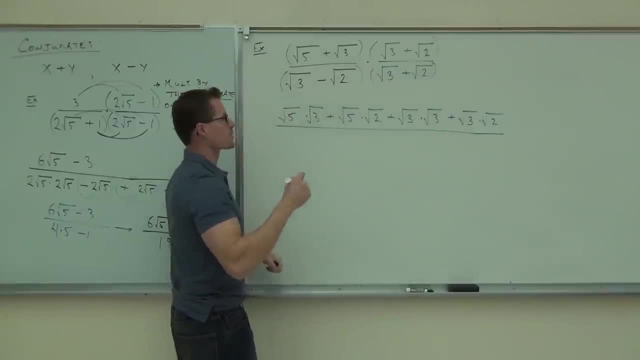 We're good to go Left side of the room. let's do the denominator the same way. What's the first thing we're going to get, please? Square root of three times square root of two. Square root of three times what? 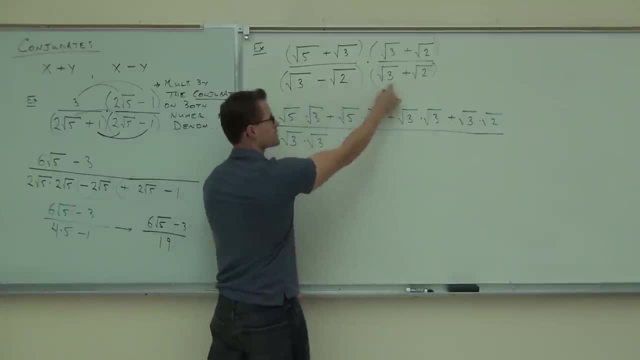 Square root of three. Perfect, Yeah, it's the vector right here. times here. What's the next thing we're going to get somebody else? Minus, Yeah, Minus, what. Square root of two times square root of three. Well, you can do it backwards, I suppose. 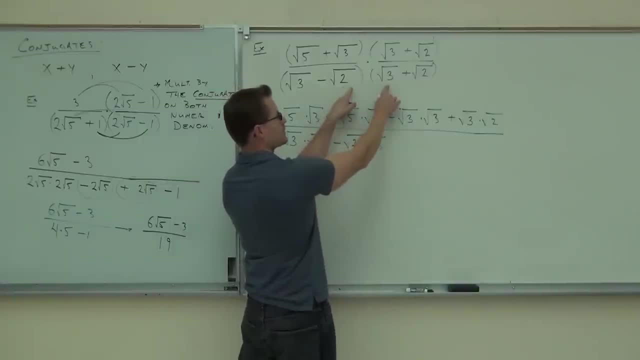 It just depends on which way we're going. Hugo, were you talking about this one or this one, This one, This one? Yeah, Then you're okay, Absolutely. I'm guessing most of you want that one first, Okay, okay. 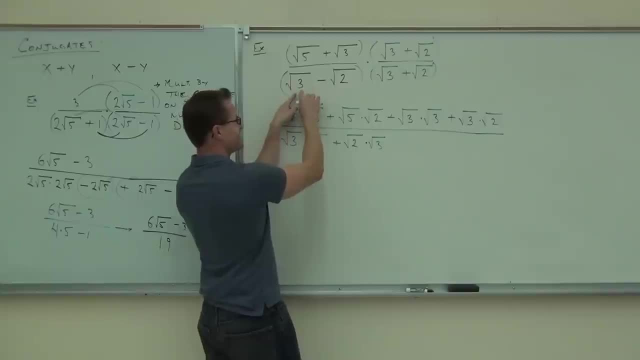 So you're like: wait a second? no, Yeah, we did this one. If you want to do this one first, then yes, you're going to get a plus, And what's this one going to be Minus? 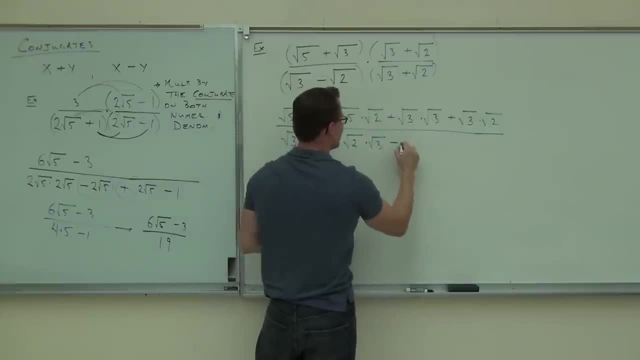 Minus, Minus. I thought it was going to be minus. Okay, you probably also don't like that, do you? You probably like that. And then this one is going to be root two times root three. Are we all better? 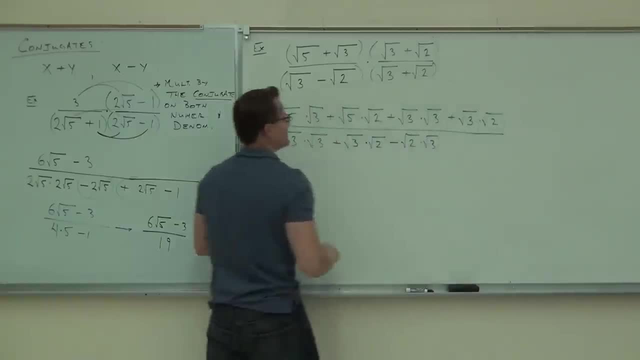 Yeah, Okay, you have your nice blanket on now. Oh my, Thank you, Mm-hmm. You're welcome, Hugo. you were right, You're fine. Well, you get all four terms. You have the right signs and the right expressions. 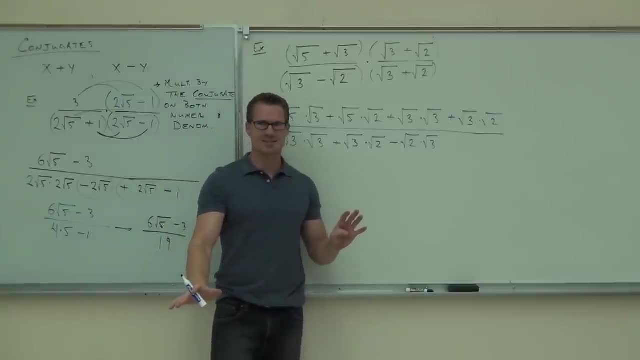 Now let's work on. there's only one choice for the last one. Okay, You can't mess this one up. What's our sign next? Minus, Minus, Yeah, and then what? Square root of two. Square root of two. 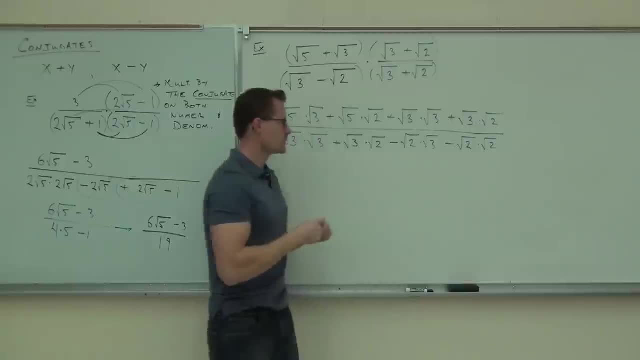 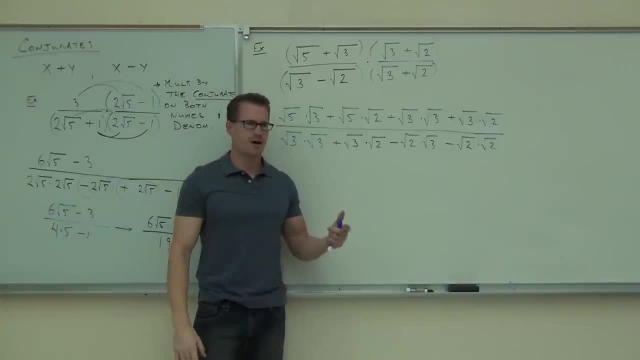 Good, We've just distributed, have all our terms out. Now is the part where you've got to simplify. well, actually, multiply whatever roots. you can Remember that if you don't have roots here, if I were to change that problem to not a 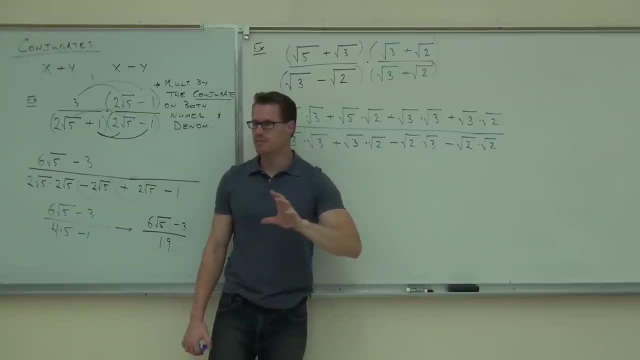 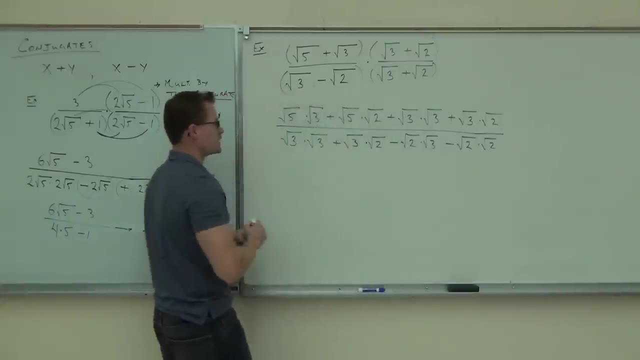 root three, but a three, a lot of this stuff would not be the same. You see what I'm talking about. Yep, A much different answer, But here we have all roots times, all roots. That's great. This is going to give you the square root of what 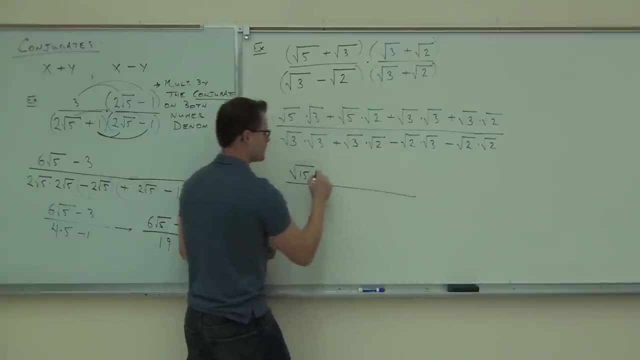 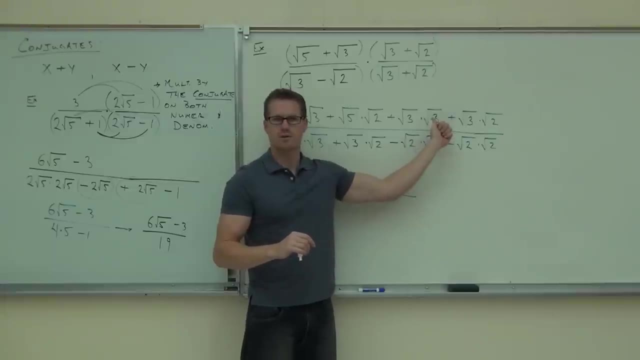 Square root of what Plus the square root of ten plus. oh, how about this? what's the square root of three times the square root of three? What's that going to give you? Three, Three, How much? Three, Three, absolutely. 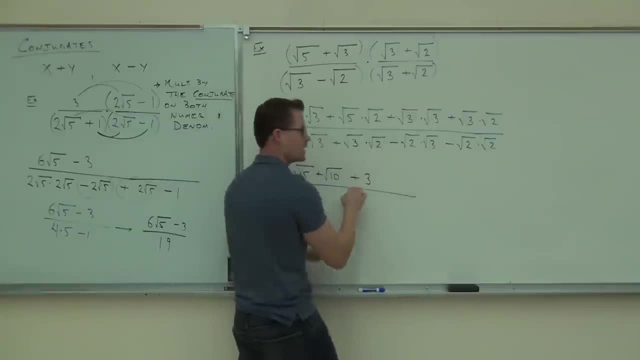 That's going to be the square root of nine or three. We know the square root times itself gives you the radicand Notice: no square root around that thing. And then plus how much Square root of six, Root 15,, root 10, three. 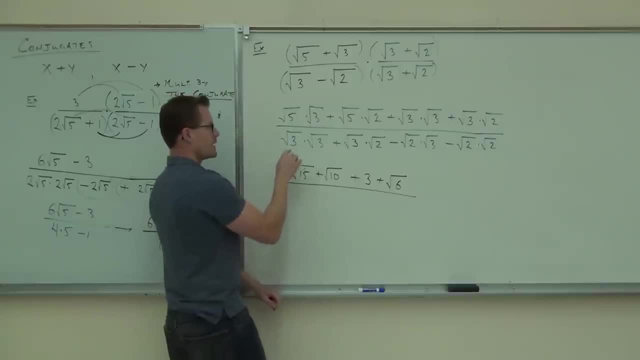 Root six. yes, no, Okay on the denominator, we have the square root of three times the square root of three. How much does that give you? 83.. Perfect, We have the square root of Six And we have, minus, the square root of six. 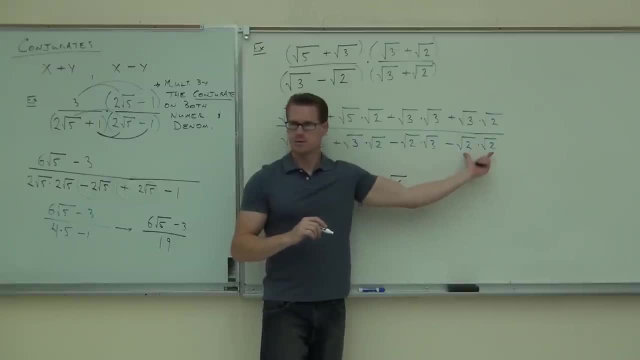 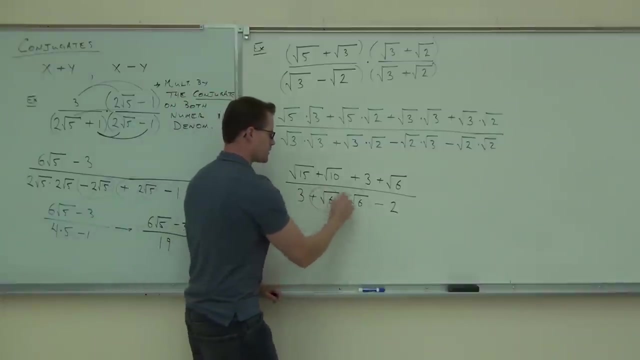 And then, lastly, we have: how much is that? Two, Two, Two. So minus two, not minus four, not minus anything else besides two, Not the square root of two. we have two, You still okay. Okay, This, that gone. 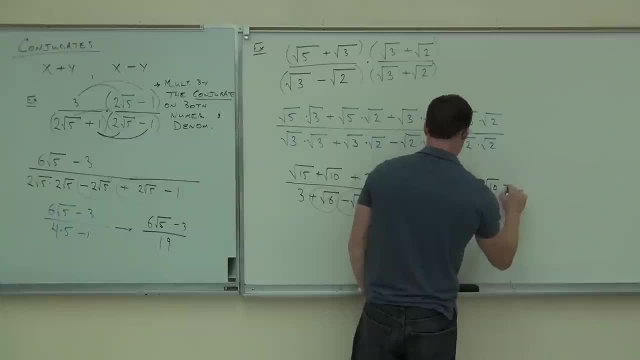 Square root of 15 plus square root of 10 plus three plus oops, plus square root of six. all over. what's our denominator going to give you One Interesting right One. Do you actually need to show the one? 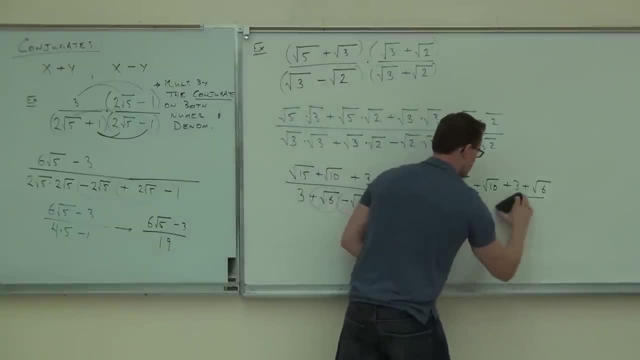 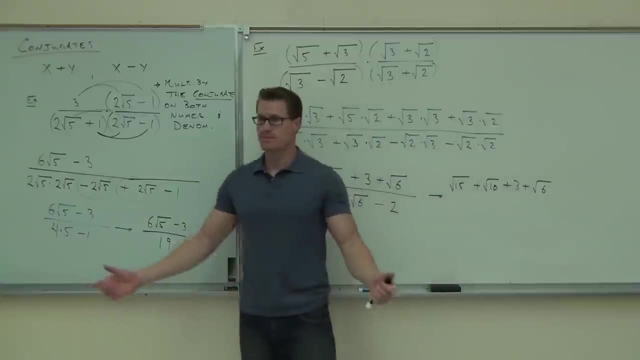 No, No, Anything divided by one is Six. No, Okay That expression. can you simplify any of this? No, That's a root 15, root 10, root, you're done. That's it As far as you can go. 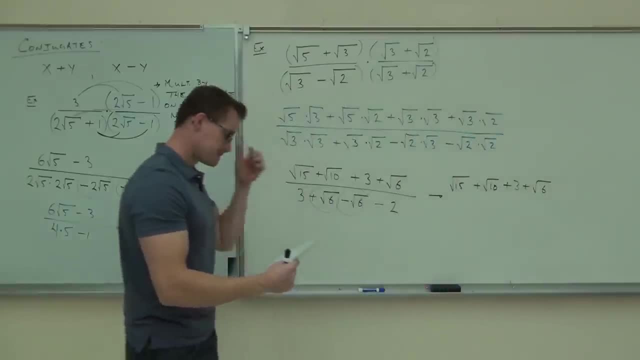 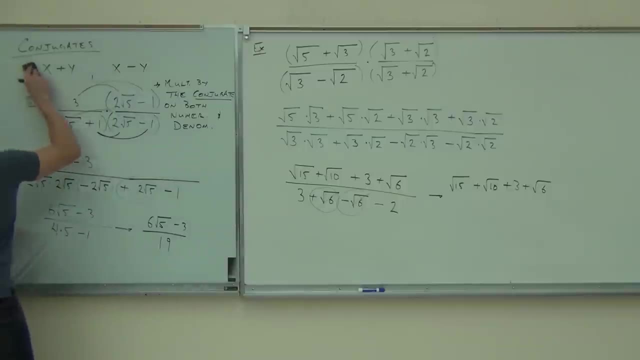 It doesn't matter what order you're on right, It doesn't matter. Okay, let's try a couple more examples and then we will be done with our section here. Do you feel okay with the idea of a conjugate? Yes, 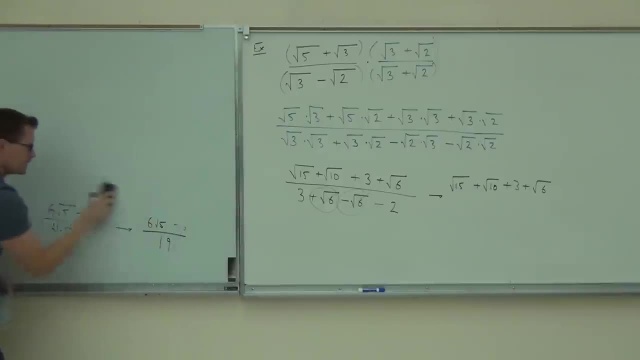 Conjugate has those same expressions, just a different sign in the middle of it. Okay, we're going to do one more together. I'll give you one more on your own. I'll talk about I'm not going to show you an example of, but I'll talk about how. 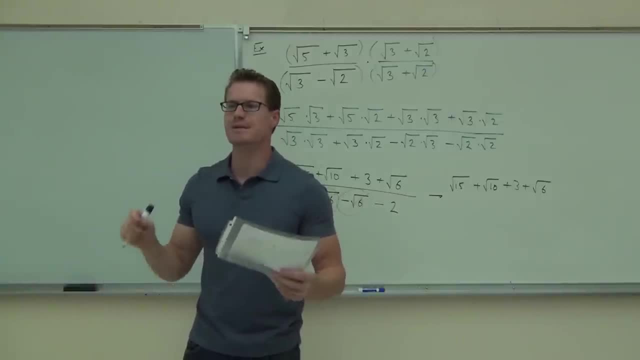 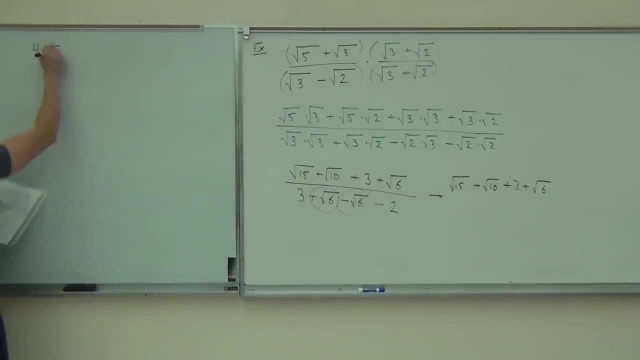 to rationalize a numerator. show you what that would look like. but you're going to see you do exactly the same thing, just with the top four fractions: Four root x over two minus root x. Okay, ladies and gentlemen, now I am going to tell you. 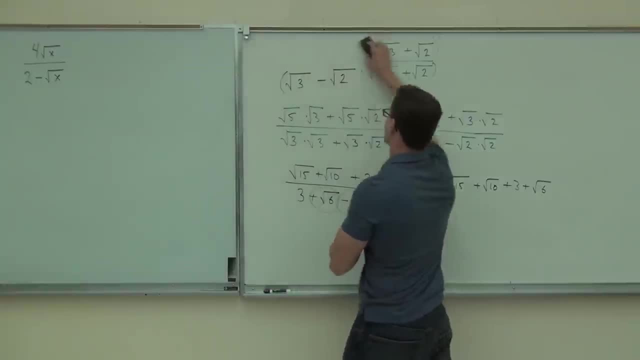 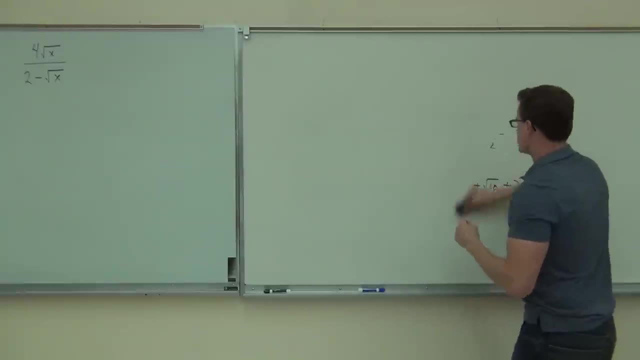 that we are rationalizing the denominator here, the denominator. We have not rationalized numerators yet. we're not going to, in this example, rationalizing the denominator. So my question is: do I want to get rid of the root x on the top? 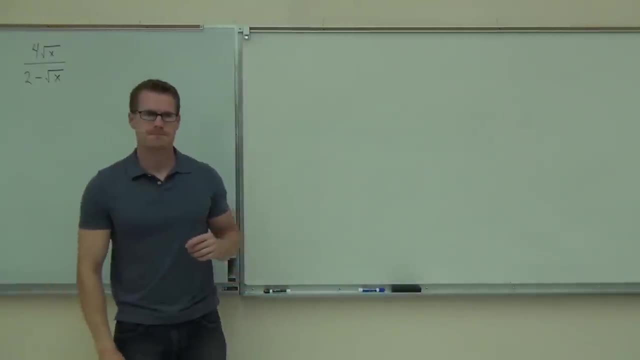 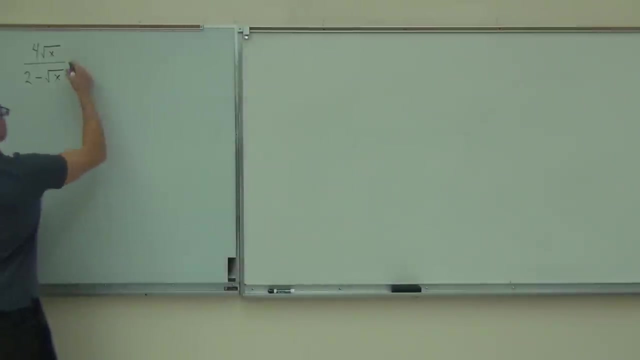 or the minus root x on the bottom. What do you think? This one, This one, Yes, Yes. In order to do that, I'm going to have to multiply by something. What we just learned is that it's not going to be enough to multiply just by root x. 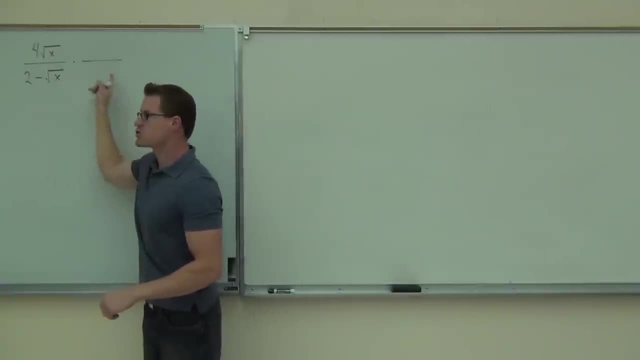 If I multiply by just root x, what's going to happen is I'm going to have to distribute that I'm going to get two root x on this problem. That's not going to get rid of the square root, where I want to get rid of the square root. 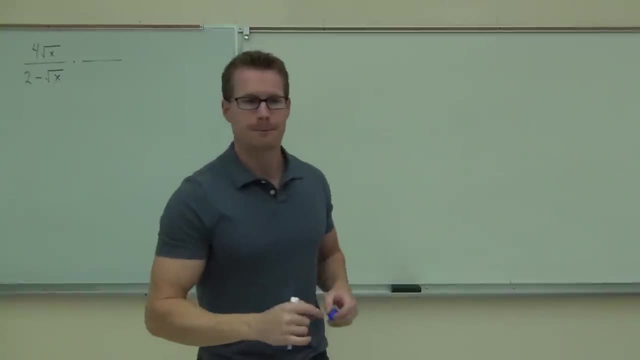 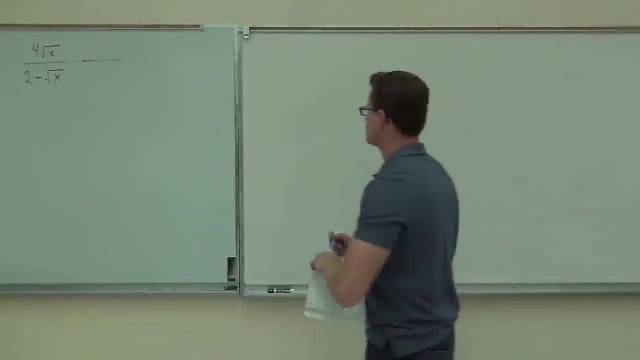 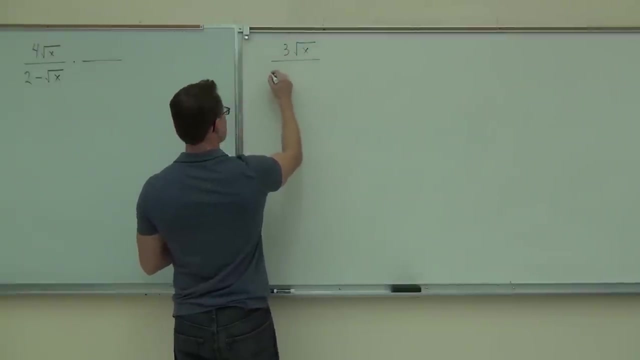 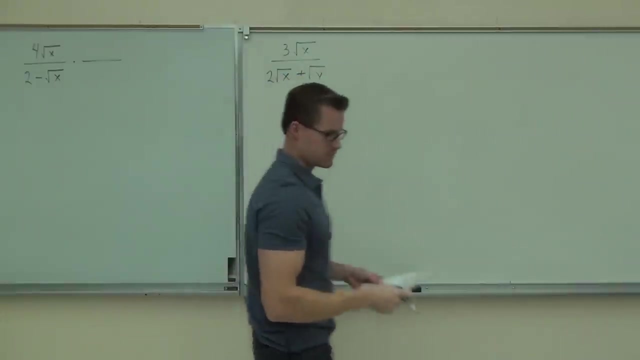 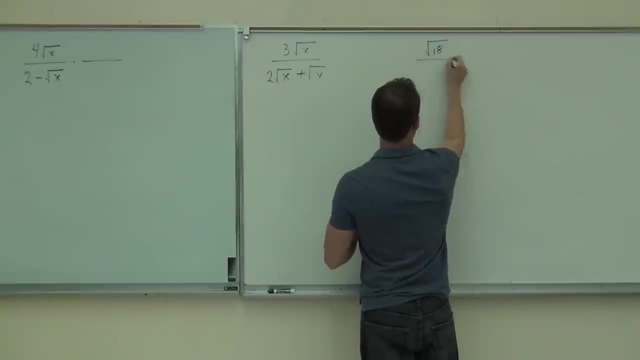 Instead, I'm going to multiply by the conjugate. I want you to do that now. That's how we're going to do it. All right, Thank you, All right, gw, chopped up. I've been back here a few times. 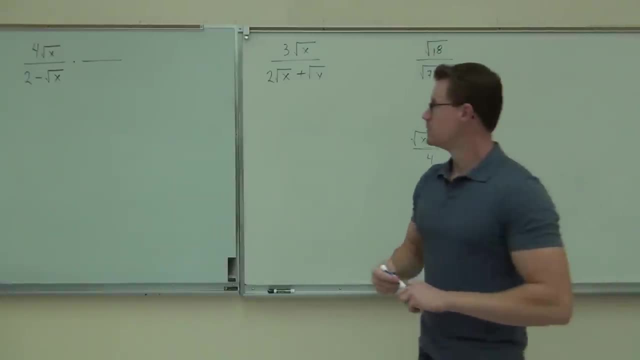 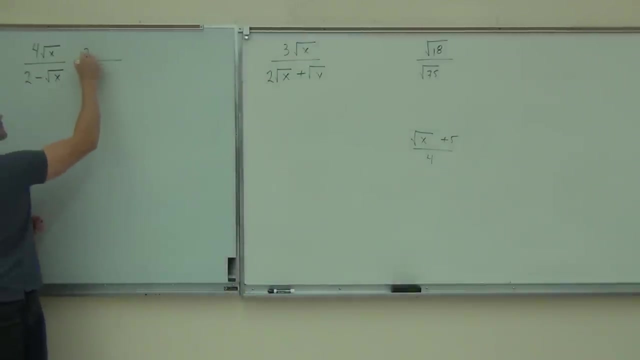 I know you do. Oh my, what conjugate are we talking about? What's going to be right here, folks? Would you give me a little head nod if that's on your paper right now? Yes, Awesome, Alright. What's the next step that you have to do? 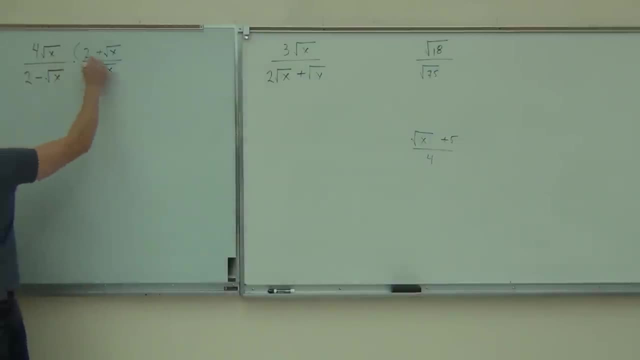 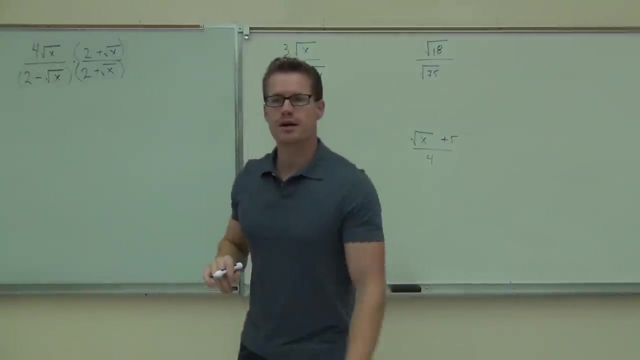 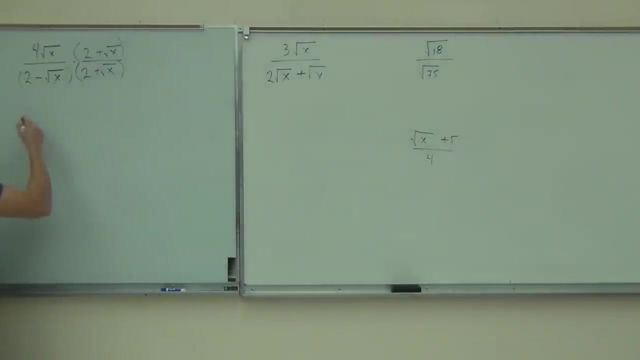 Distribute Lots of distribution, absolutely. We have this and you're going to have to distribute that. If you haven't done so, I'll give you a few seconds to distribute. right now We're not doing any math in our head, we're just writing it out. 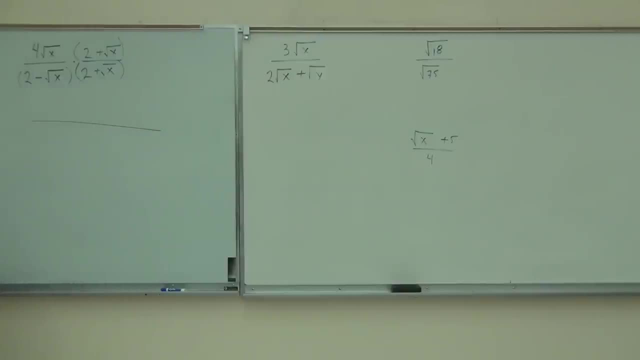 Did you get that for your numerator? if you've written it out already, Yes, No, Okay, Denometer, we're still writing that out, This one. We're going to make that 8 in a little bit. I'm just writing it out right now. 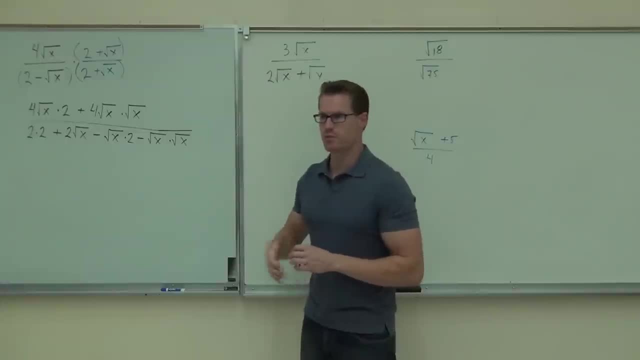 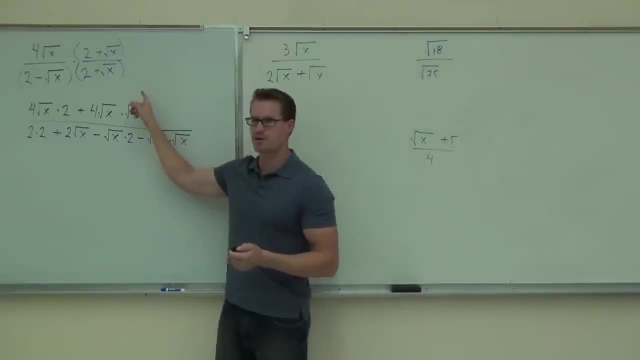 Hey, by the way, if you're trying to rationalize and you end with a root where you're not supposed to have one, did you do the right thing? No, You should probably go back and fix that Right. So if you're rationalizing denominators and you end up with a square root on the bottom, 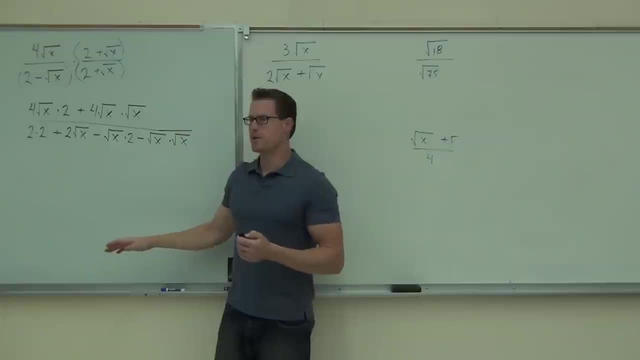 of your fraction. you probably need to go back and fix that problem, Don't just leave it. Go back and fix that. Then did you get this part as well? Yeah, How many people got that part? Alright, How much is 4 root x times 2?? 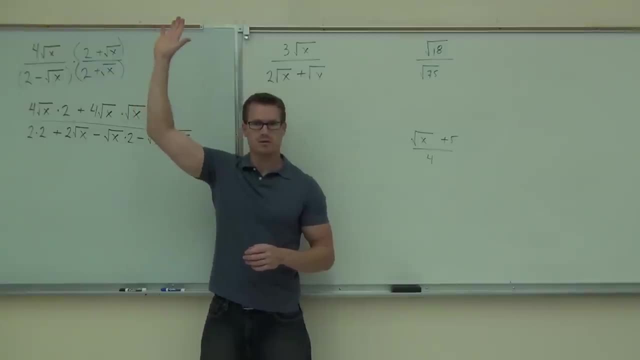 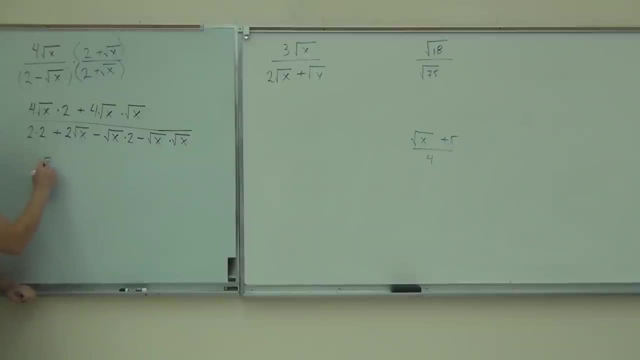 8 root x times 2.. What's that going to give you 8 root x Plus, how much is 4 root x times root x? How much is that going to give you 4 root x? Good, Any roots. 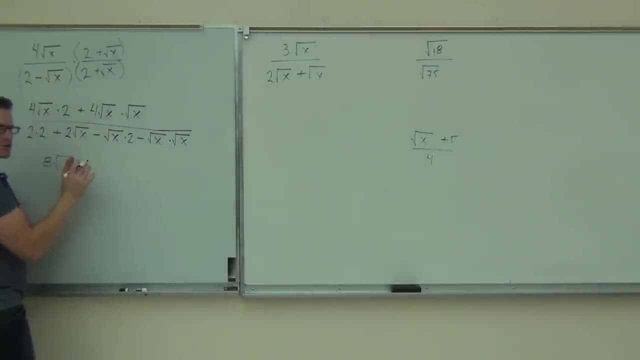 No, No, Square root times itself is going to get rid of that radical. You're going to get the radicand, So this gives you x, So we get 4x. Well, that's kind of nice. That already looks a little bit better. 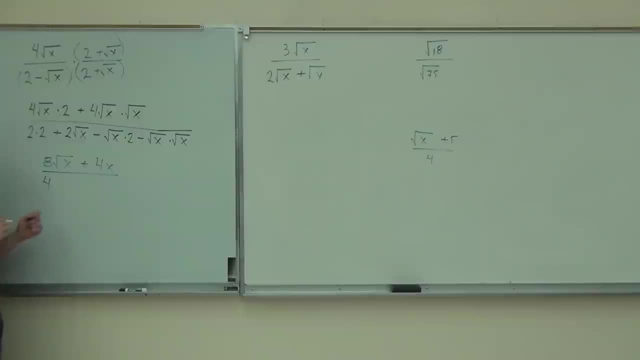 On the denominator, we're going to get 4.. That's not bad. How about this? Are these the same expressions: 2, root x and root x times 2, that means the same thing: One's plus, one's minus. 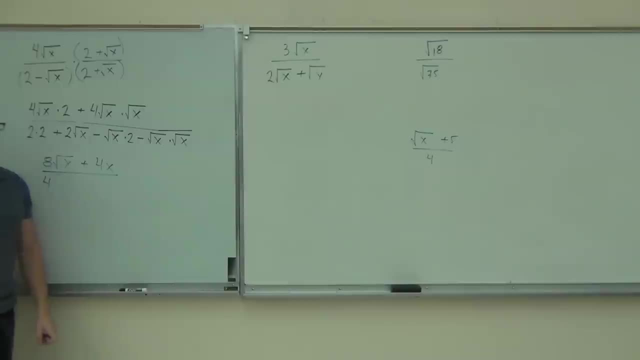 These things are gone. That simplifies to 0.. How about root x times? how much is root x times root x? So we're going to get what here? Or minus x? We have 8 root x plus 4x over 4 minus x. 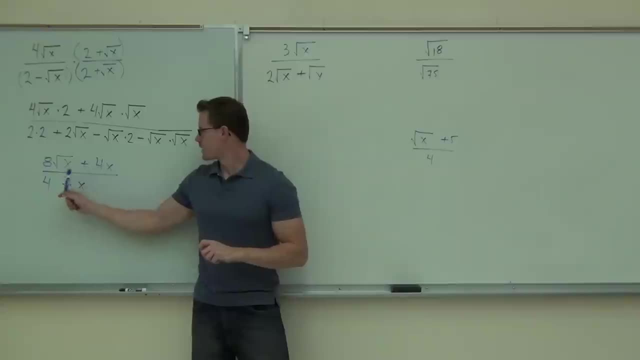 One quick question: Can I simplify The 4 and the 4?? No, How about the x and the x? No, Definitely not. These are being added, These are being subtracted. There's no way I can simplify any of this stuff. 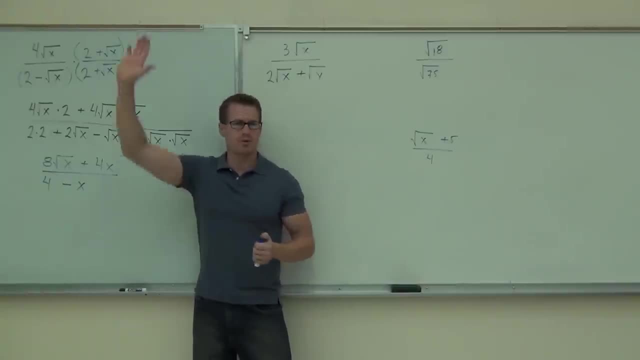 That's your answer. You're done. How many of you feel okay with this? so far, Good deal. Try this one. Try this one on your own. We'll talk about these ones in just a bit. what I want you to do on those: 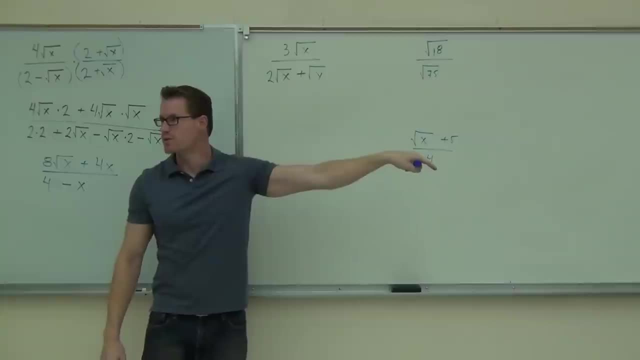 Okay, So do that on your own. Multiply by the appropriate conjugate, Distribute, Simplify, Go slowly, Show all the work like we just showed. Okay, The last one we're going to do is multiply by the appropriate conjugate. 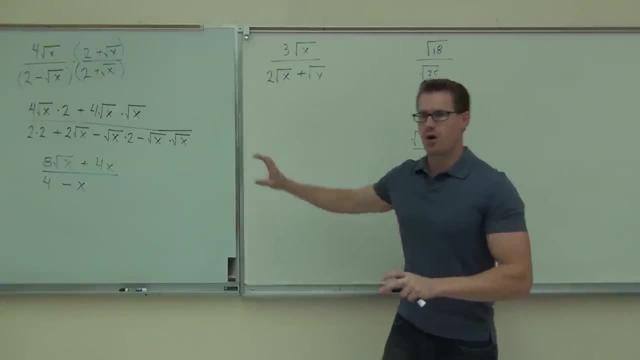 Distribute, Simplify, Go slowly, Show all the work like we just showed. Okay, The last one is enumerating the problem. right, We're going to do numerators on the last one. Oh, we'll talk about it. 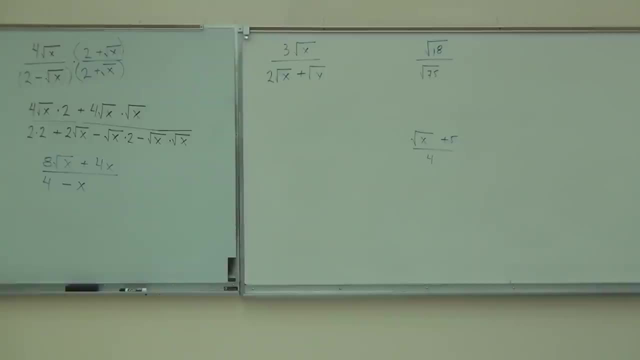 Conjures are kind of fun. huh, Kind of cool how that works. It's written square roots for you. Remember, this will only work for square roots, So that's all you'll have. So have we seen anything else? No, 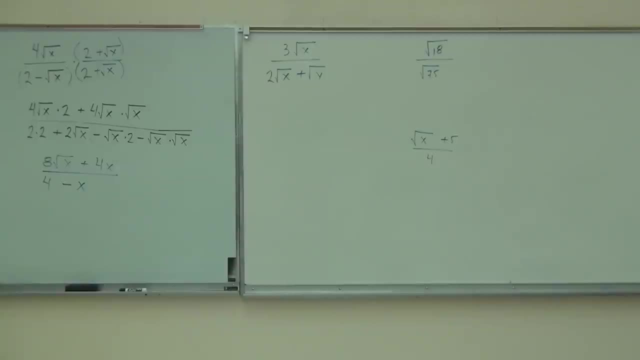 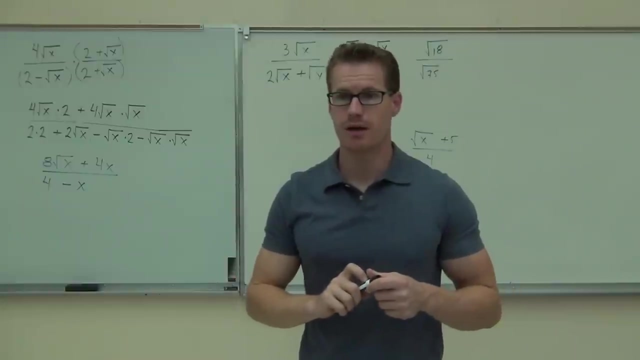 Okay, Thank you. So we're going to do the problem. We know it's a typo. Yeah, Or it's a different type of problem. Hopefully you got the correct conjugate: 2 root x minus root y. Do you all have that? 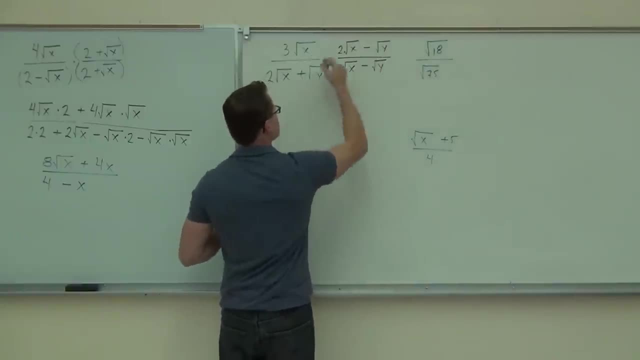 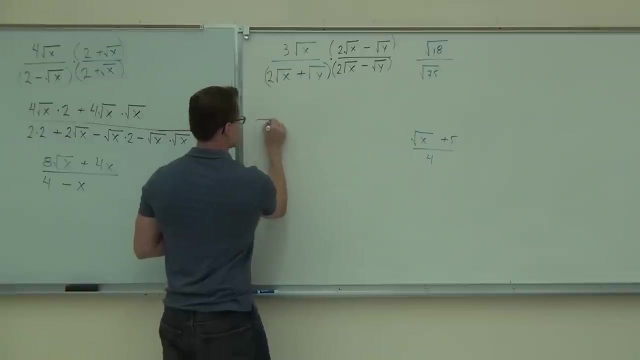 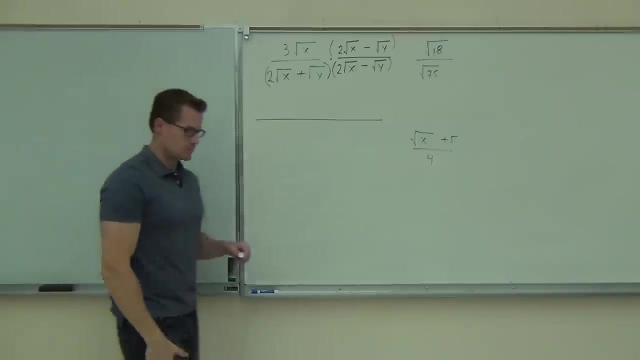 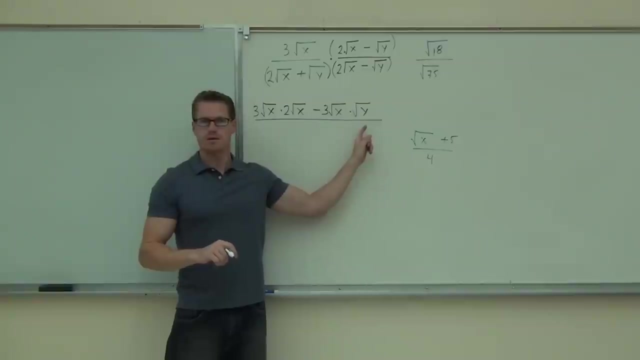 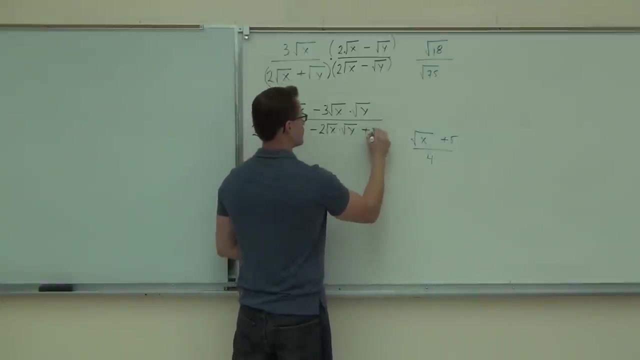 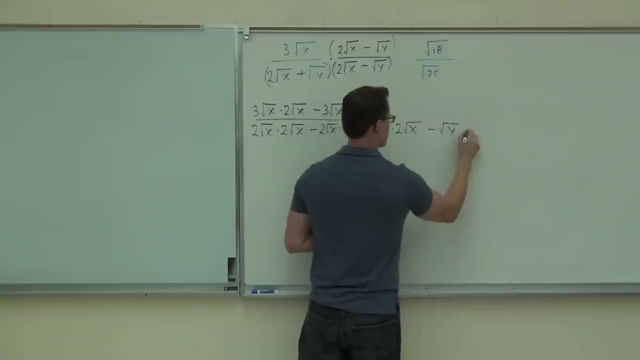 Okay, good, Continue. Thank you, Check your numerator. Did you get this on your next step? 3 root x times 2 root x minus 3 root x times root y. Do you all have that? Okay, good, Check your denominator. 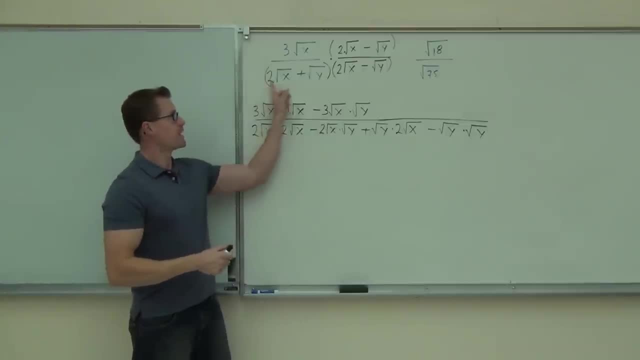 Do you all have that for your denominator 2 root x times 2 root x minus 2 root x times root y plus root y times 2 root x minus root y times root y. Do you have all those expressions with all those signs correct? 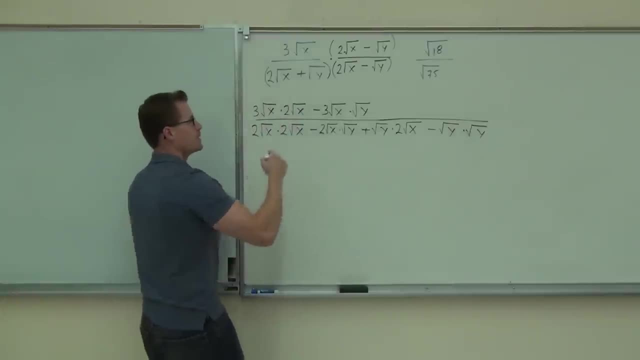 Yes, Okay. now it's the part where you're simplifying On this. this gets tricky if you're really not sticking with it and not understanding the difference between addition and multiplication On this example, with this first part, what are you going? 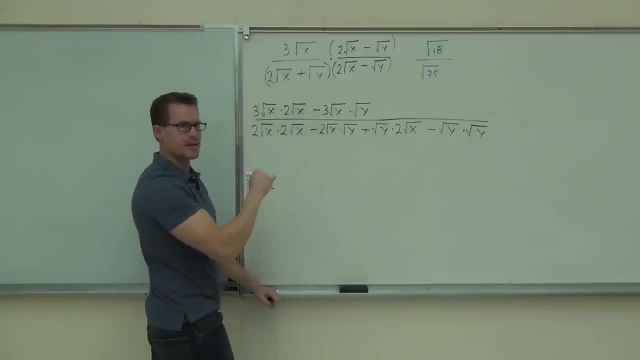 to get 6 root x or 6 x, 6 x, 6 x. good Root times. a root gives you the radicand 6 x. Perfect. On this one we of course have a minus, Minus. what? 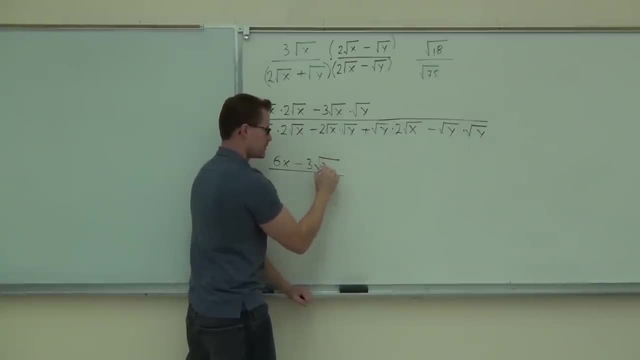 3 root x, 3, and then 3 root x plus xy, xy. perfect, put them together. They both have a square root. So far, so good. Denominator's the fun. part 2 root x times 2 root x, that gives you 4?. 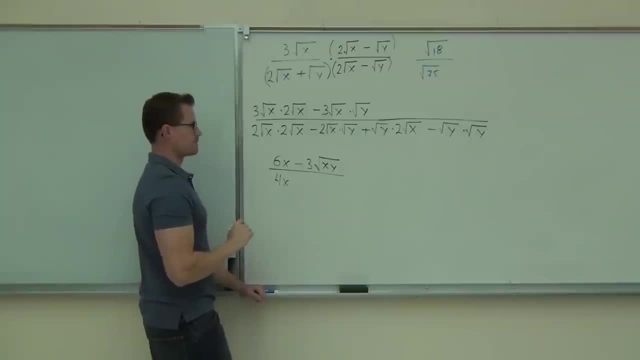 4x Perfect, 4x Good. Do the middle terms simplify out of my expression here? They're exactly the same thing. I've got these three things and these three things being multiplied a plus and a minus. They're gone, so I'm going to have a minus. 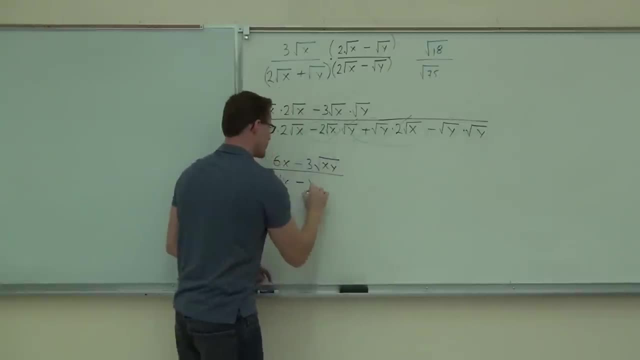 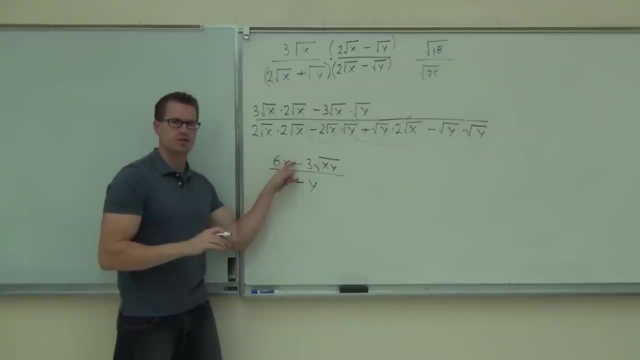 How much is your root y times your root y Y? Is there anything more I can do with my problem? No, Please do not simplify these. You can't. They're connected by a subtraction. You can't cross out the x's. 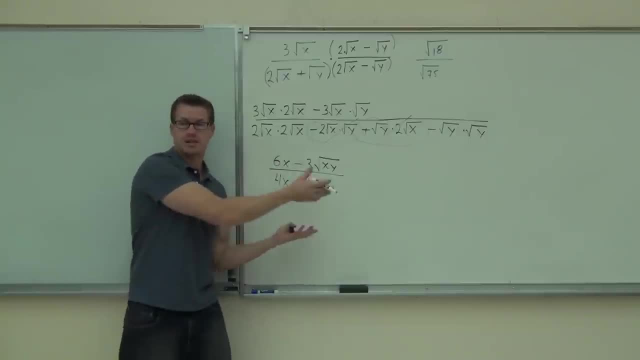 You can't make that 3 halves, Can't do anything with this. That's it. You're done. Okay, Don't invent more mathematics to make it look prettier. You can't do anything more. I'm going to feel all right with that. 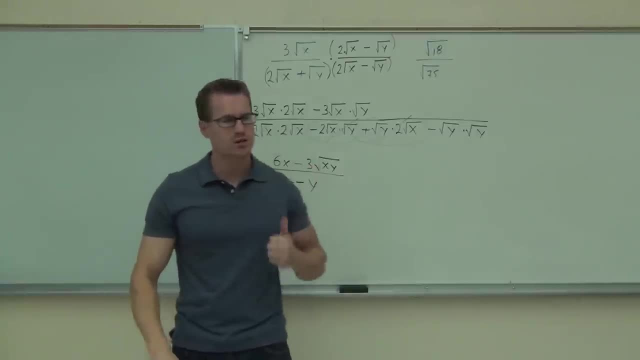 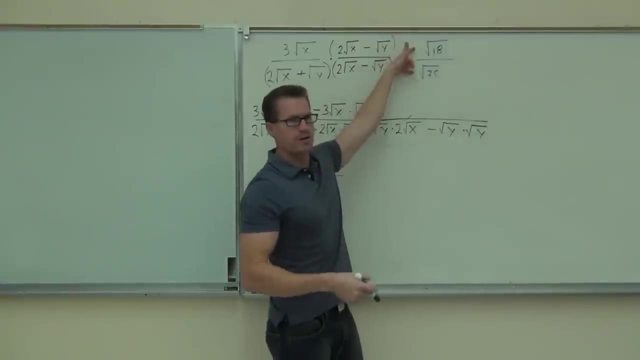 Did you get that far? Good for you. Remember how to do that problem And you're going to be set. Now, as far as the numerators go, the only difference we would have is: can you rationalize the numerator instead of the denominator? 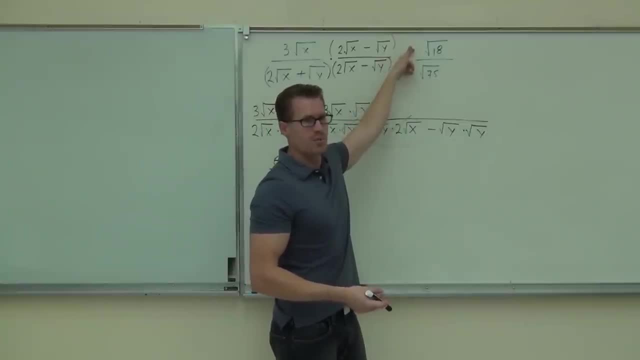 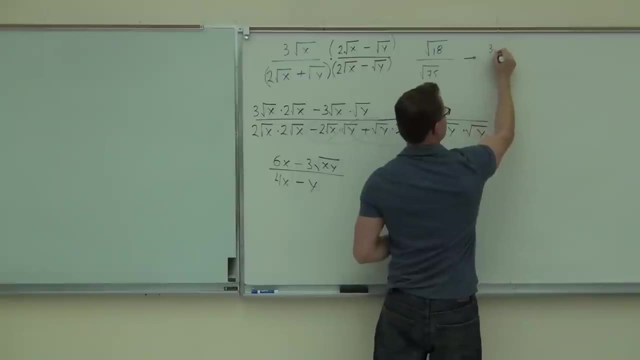 Sure, You'd simplify first and then multiply by the appropriate root. So here I'm going to do this quite quickly, But this you would simplify as, let's see, it's 9 times 2, so 3 root 2 over 5 root 3.. 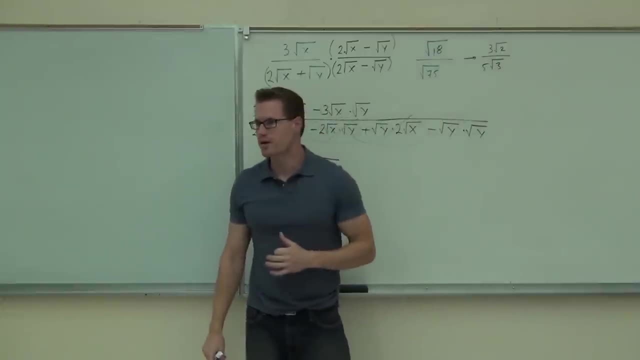 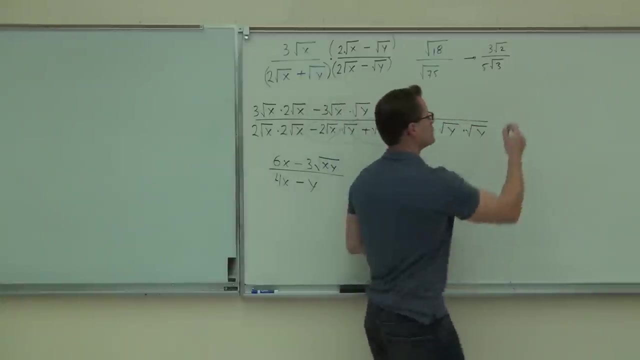 You see where those numbers are coming from. To rationalize the numerator, instead of multiplying by the square root of 3. We'd simply multiply by the square root of 2.. That's going to get rid of the square root on the top. 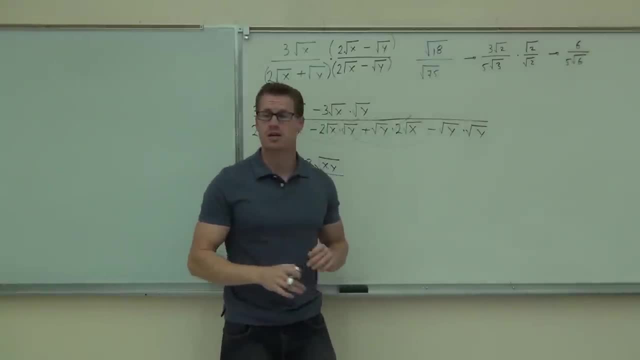 You would get 6 over 5 root 6.. That would be your answer there. Double check that on your own when you get home, The one thing that we're doing. hopefully, that's right. You double check that on your own right now. 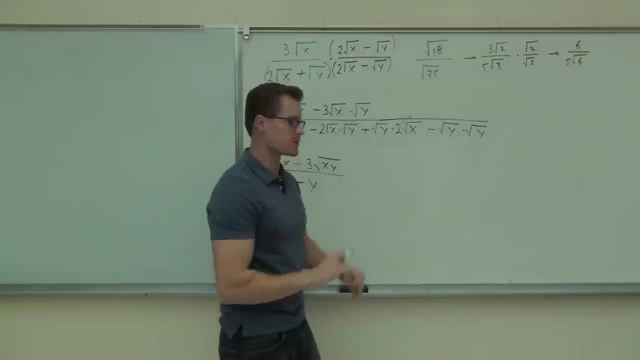 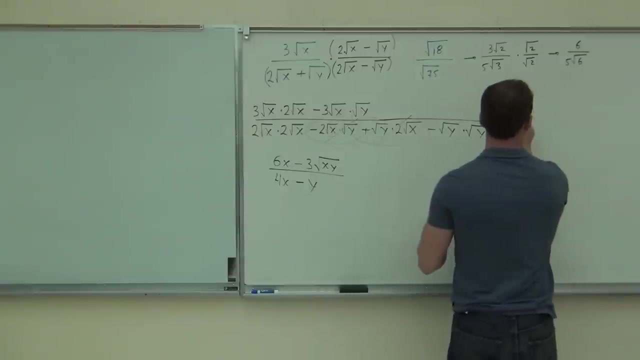 Yeah, Okay, The only thing you're doing is rationalizing the different part of those fractions, The other one that I gave you. Could you rationalize the numerator on this problem? What would you need to rationalize the numerator on this problem? 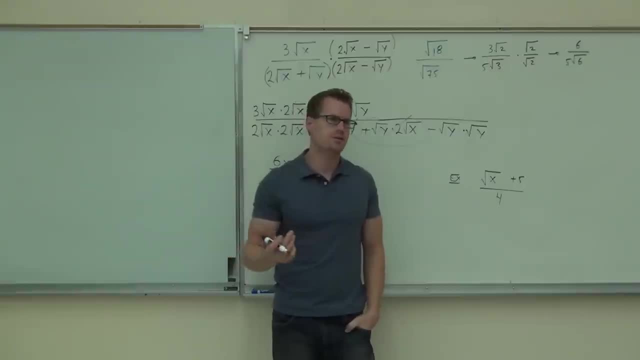 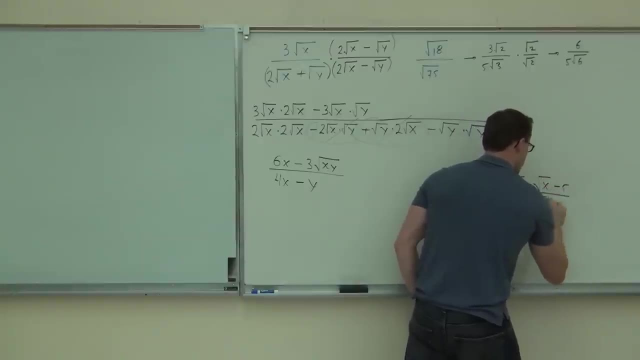 What's that called when you're doing the root x minus 5? 1 minus 3.. You still need the conjugate, even though it's on the top of the fraction. The only difference is you'd be doing root x minus 5,. 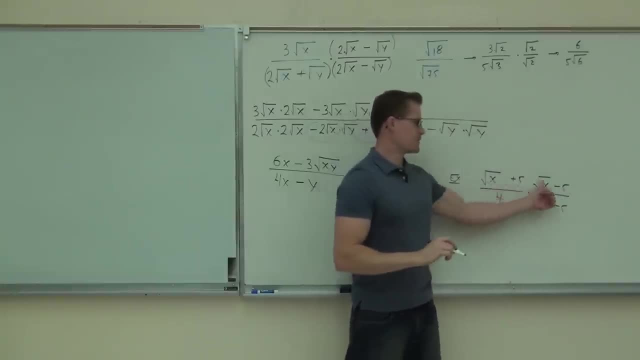 root x minus 5.. You're just going to be moving a root from the numerator to the denominator. That's what's going to happen here. This, if you notice, you still have that difference of squares idea. You're going to have x plus and minus 5, root x and then minus 25.. 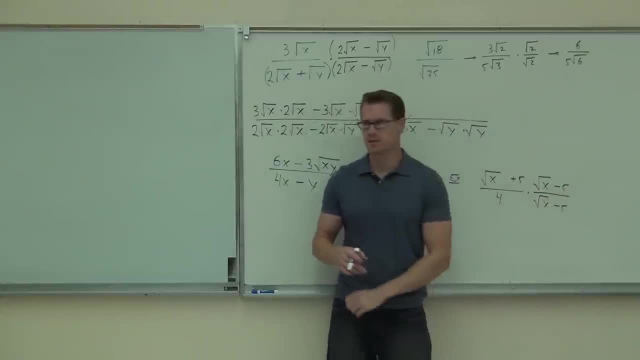 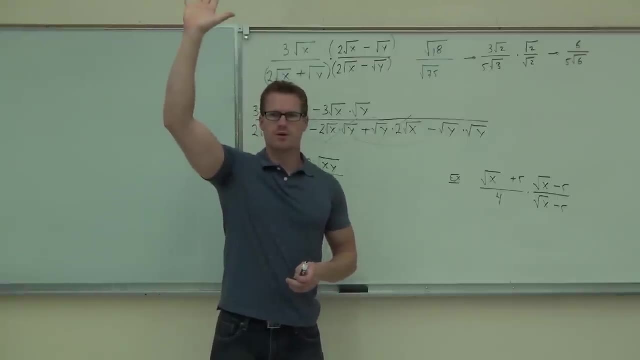 Your answer is going to be x minus 25 over whatever this is, when you distribute 4 root, x minus 20.. That would be your final answer there. How many will we get? How many people feel okay with what we've talked about so far? 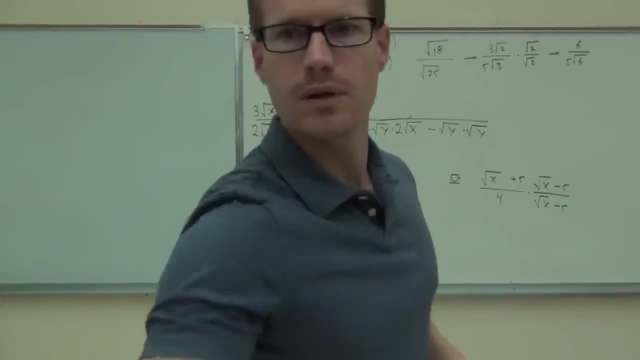 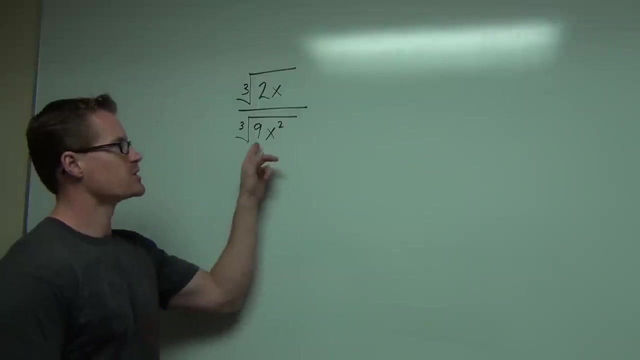 Good deal, All right. So I'm going to give you one more example on how to rationalize the denominator. Only this time I'm going to incorporate both variables and numbers, which I didn't show you in class. So what I'd like you to do is, instead of rationalizing the 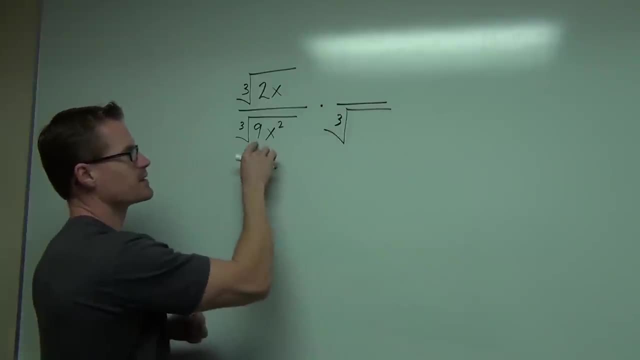 denominator by saying: okay, I need to rationalize and make this a perfect cube like multiply by 81 or something that's incredibly big. Instead of that, Think of this as something slightly different. Change that number into a power, Or in other words, change it into a number to some power. 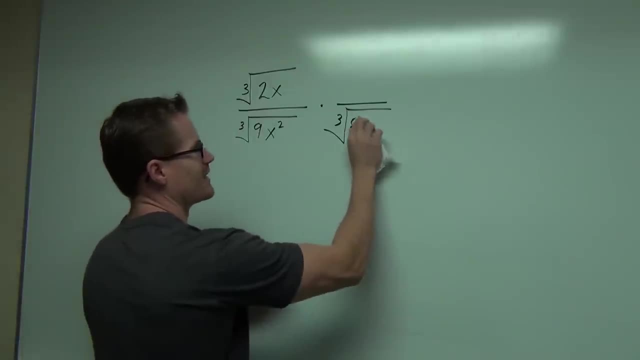 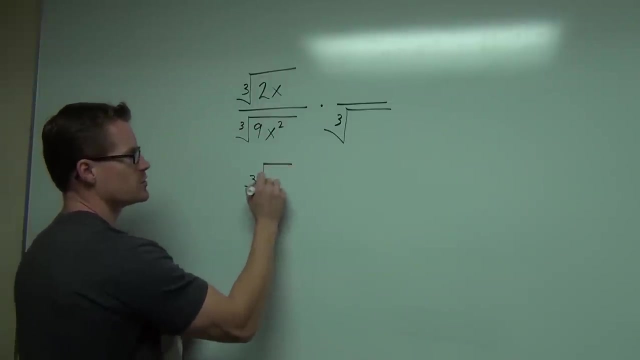 So, instead of doing this cube root of 81, no, no, no, no, no, We don't want to deal with that. Instead, think of this as the cube root of 2x. no problem over the cube root of you're going to change 9. 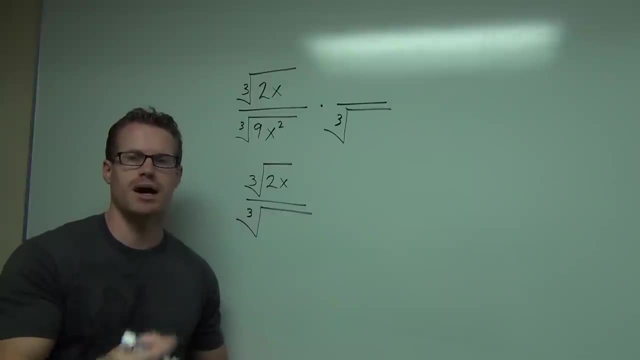 or whatever number you have into some number raised to some power. So for instance 9 you can write as 3 squared. Realize that that is still 9.. I'm just writing that as a power And x squared stays the same. 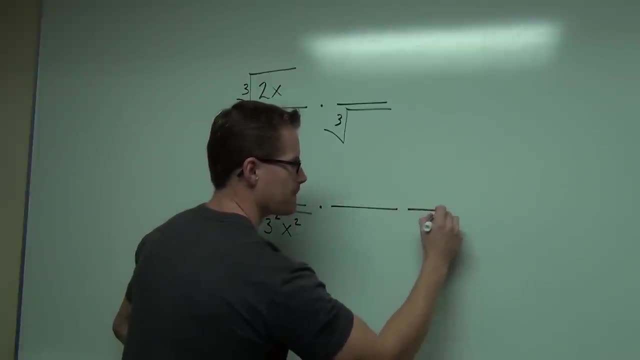 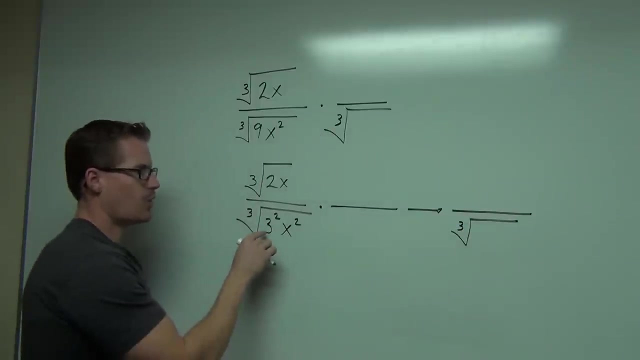 Now, when you rationalize it, what we're going to be trying to get is a cube root of. I want this to the third power. I want this to the third power Because I know every time I have a power matching the root. 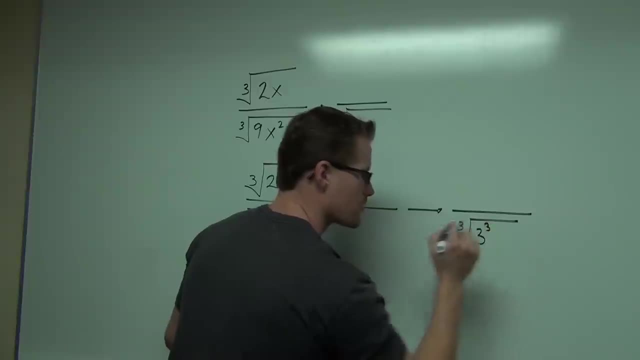 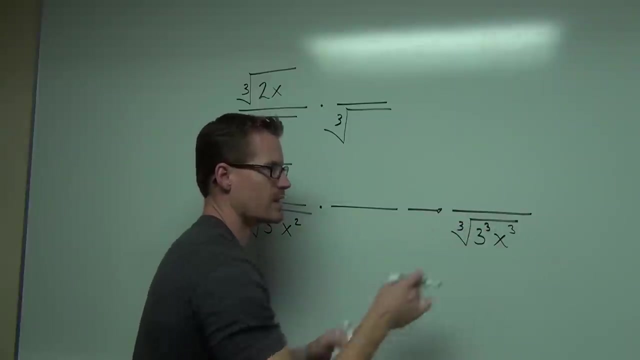 I'm going to simplify. So, in other words, I want 3 cubed, Just like I want x cubed. That's what I want, right, Because I want my cube and my cube root to match up. I want my cube and my cube root there to match up as well. 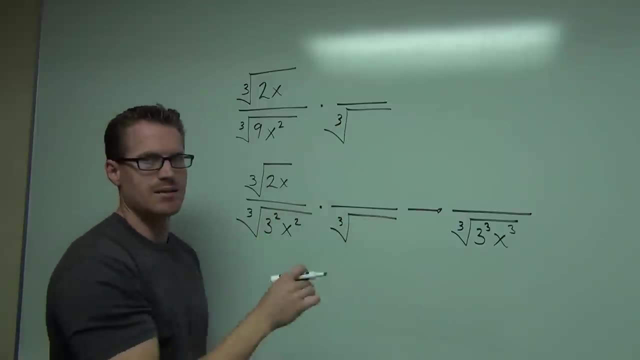 So then you think about, instead of a large number like 81, making that- I don't know even what that is. It's a huge number. We don't even want something that big. We want something very simple that we can cross out. 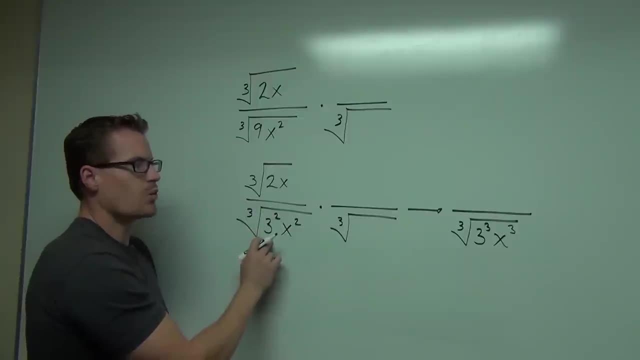 That's why we write this, instead of 9, as 3 squared. So what does it take to multiply 3 squared and get 3 squared, 3 cubed? That's just going to be 3 to the first power. 3 squared times 3 gives you 3 cubed. 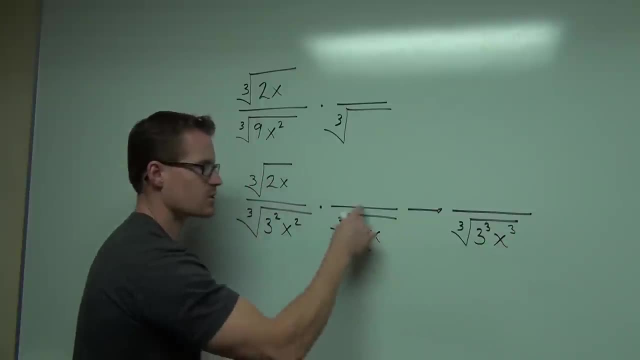 X squared times x to the first gives you x cubed. So this is the expression we need: to multiply. That's a lot better than multiplying by the cube root of 81. We don't want that at all. That would be a bad thing to do. 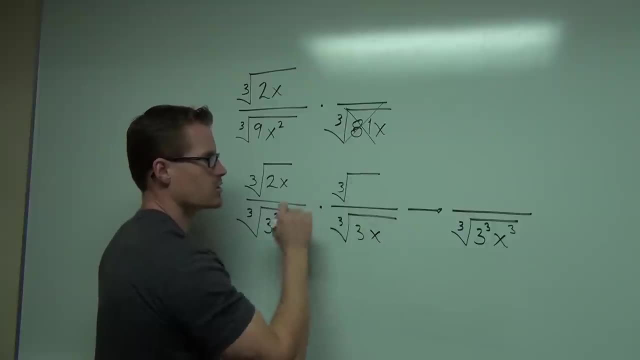 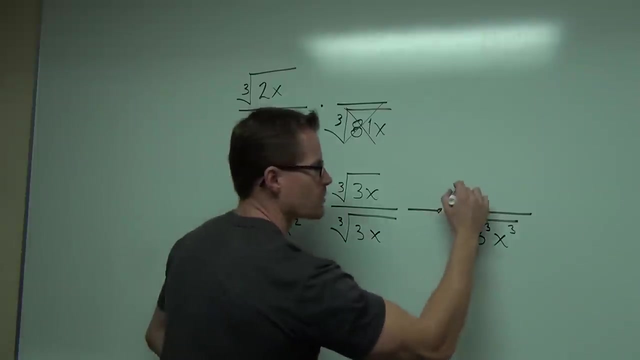 It's going to be way too large on our numerator. Of course, our numerator must match our denominator. We're going to have the same cube root- cube root here, cube root here- So we're going to get it. We're going to get it. 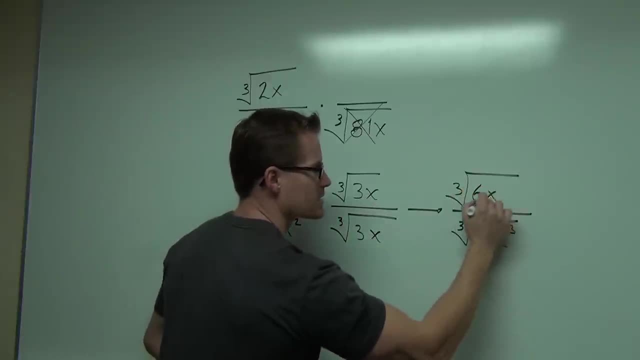 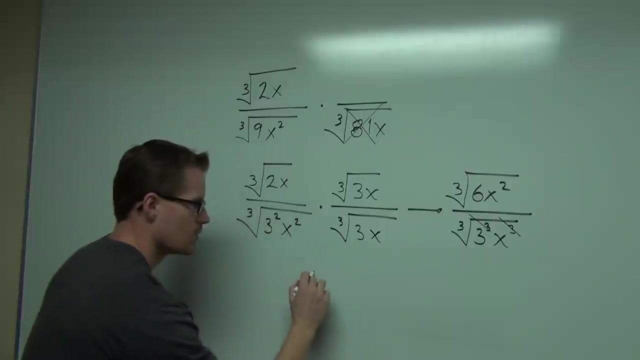 We get a cube root of 6x squared over the cube root of 3. cubed x, cubed Those. simplify: We get the cube root of 6x squared all over 3x. Cross that out, you get a 3.. 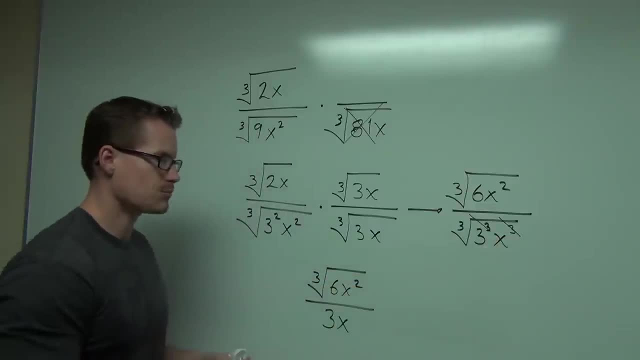 Cross this out, you get an x. That leaves us with 3x. So the whole idea: when you're dealing with numbers and variables, treat those numbers as a base to some power, just like you would a variable. Then you're multiplying by that number to an appropriate power. 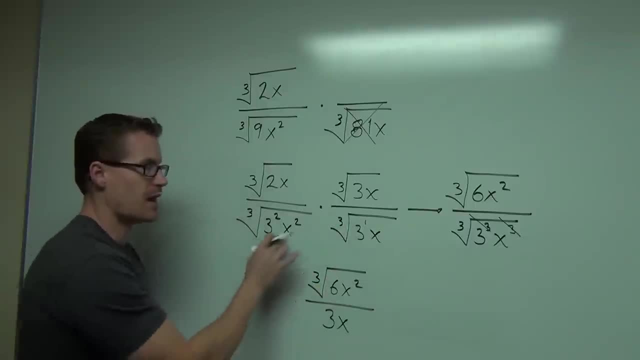 So here we have 3 to the 2nd multiplied by 3 to the 1st. That makes 3 to the 3rd, which you can cross out. Don't deal with them as the numbers that they are. Deal with them as a base to an exponent, just. 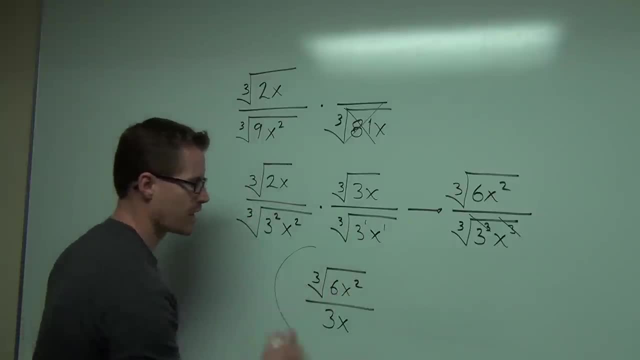 like you, would a variable and things become a little bit simpler. This is your final answer and that's the last example I'll do.